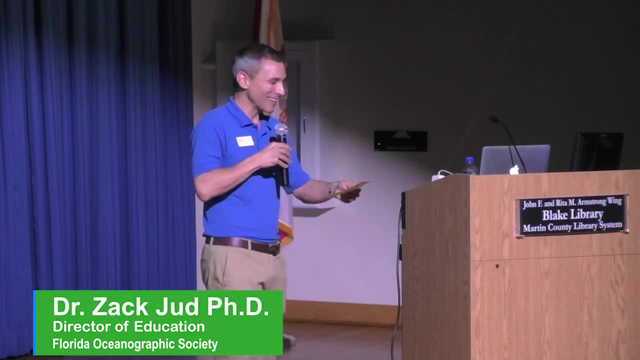 are all here for tonight. Tonight's special guest speaker, Dr Denise Herzing, is the Founder and Research Director of the Wild Dolphin Project. Dr Herzing holds a Master's Degree from San Francisco State University and a PhD from Union Graduate School. 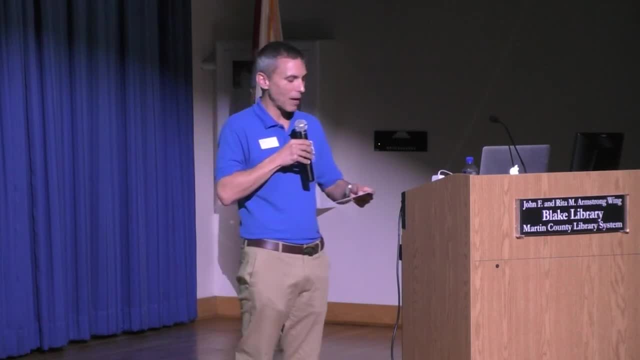 Since 1985, she's been monitoring a population of wild spotted dolphins in the Bahamas. Tonight, Dr Herzing is going to be telling us about her nearly four-decade long journey working with these incredible animals. It is with my greatest pleasure that I welcome to the. 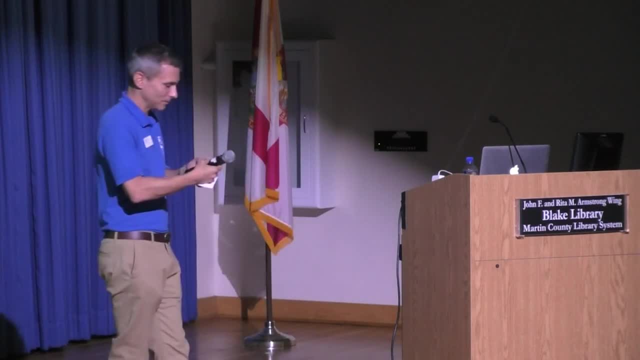 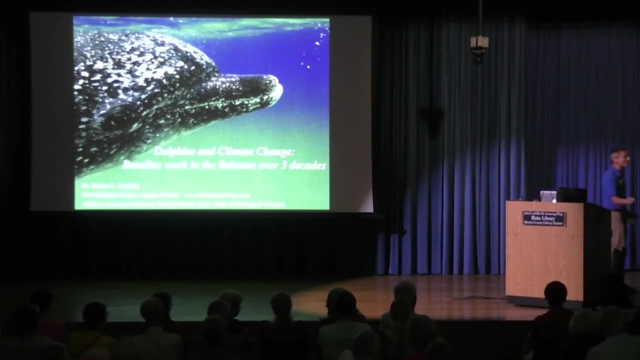 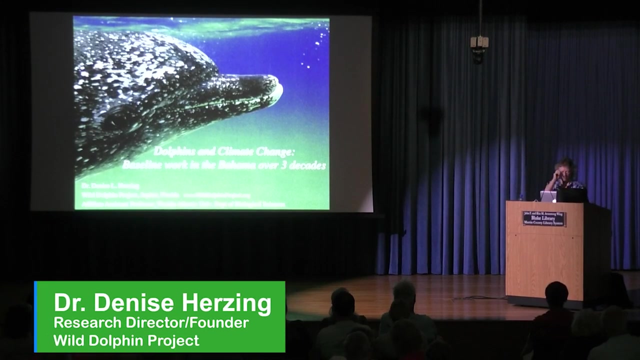 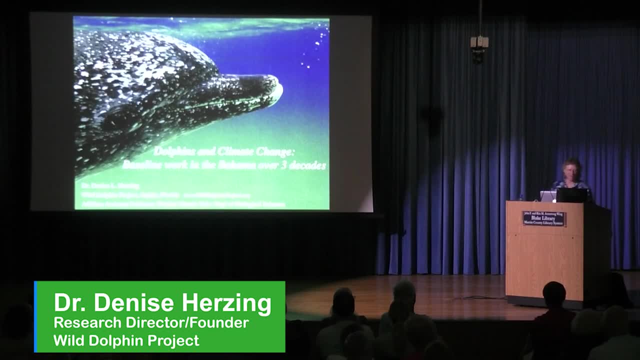 And it's terrific to be here. Thank you to Florida Oceanographic for having me. As you know, they've done decades of great work and continue to do so, so we're happy to share what we know about the dolphins and tell you our story. So I want to, first of all, tonight. 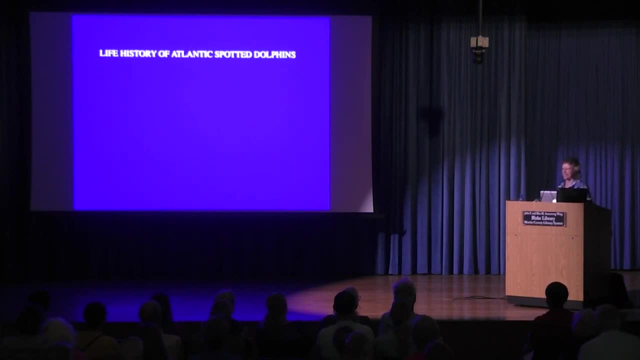 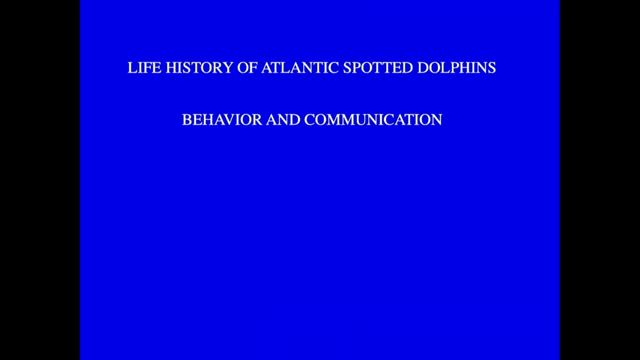 I want to tell you about the dolphins themselves, about their society and who they are as a species, so you can get to know them a little bit. want to tell you about their behavior and communication, because that's primarily what we study. I want to tell you what they eat and how they forage. 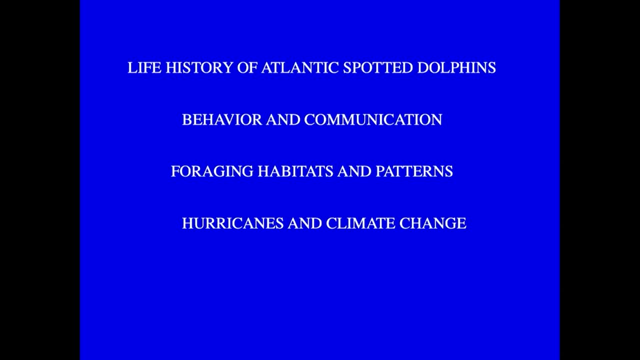 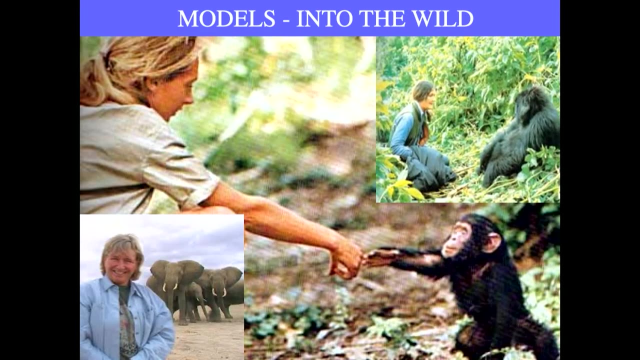 And then, finally, I want to tell you some of the big impacts that hurricanes and climate change has been having on the dolphins. And then we'll just finish with some of the tools that researchers are using all over the world to monitor marine mammals specifically. Now, I started my work because I was inspired. 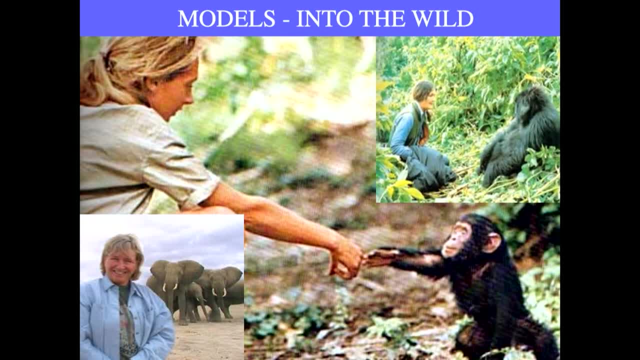 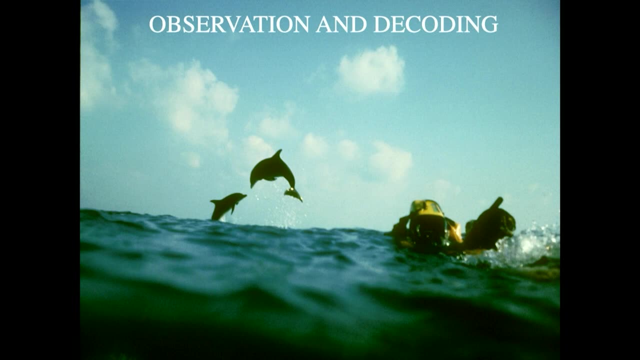 by the primatologists that were out there studying great apes and and even the Cynthia Moses studied elephants. So I picked a spot where I could watch these animals underwater and try to get a handle on their society. So most of what we do is by observation. Now, the reason I chose the Bahamas is because in most 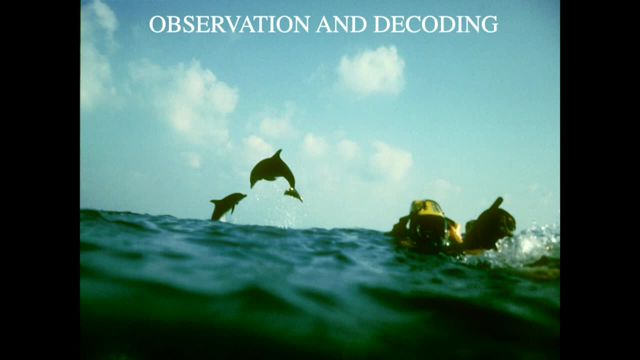 parts of the world. the water is just simply too murky to observe underwater. So you might see dolphins jumping like this, but you don't really know what they're doing underwater till you. till you look, And in fact they're probably fighting underwater. They're not playing, which is what most people think. 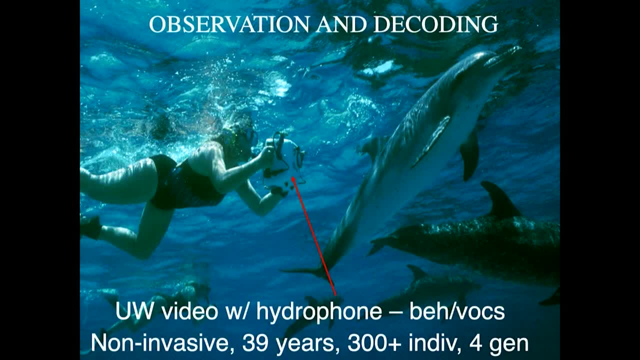 So we spend our time underwater. My primary tool is underwater video with a hydrophone, which is underwater microphone, And of course, we have GoPros and all sorts of new things these days And our work is non-invasive. We are almost at 40 years and four generations of dolphins, So we basically go out every 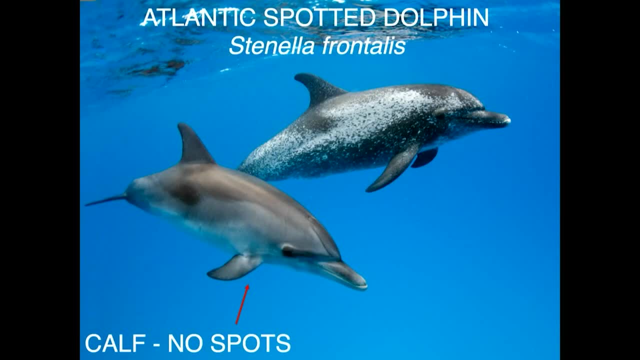 summer and observe dolphins. So we basically go out every summer and observe dolphins. these dolphins- now the species are Atlantic spotted dolphins- and the calves are born without spots and they gradually get spots, like you see here this animal, Mugsy- she's 35 years old. in this photograph We use Nixon notches in. 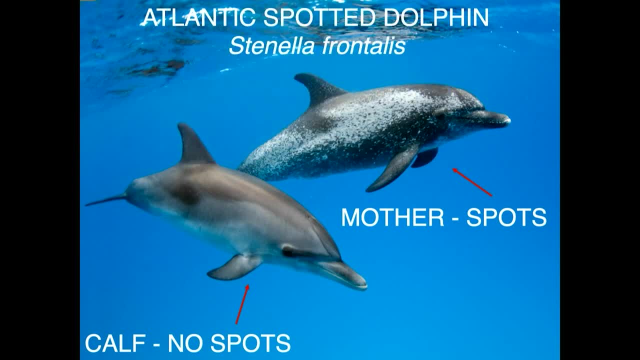 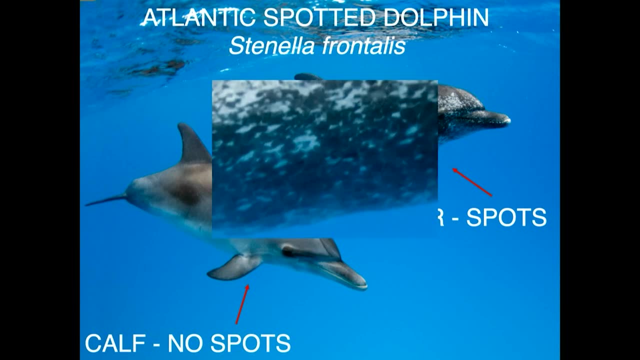 their dorsal fin, which is typical of dolphin researchers when you're working from the surface. But because we work underwater, we can also use their great spot patterns, which are like constellations. That's how we track individuals. So every summer we go out re-photograph. 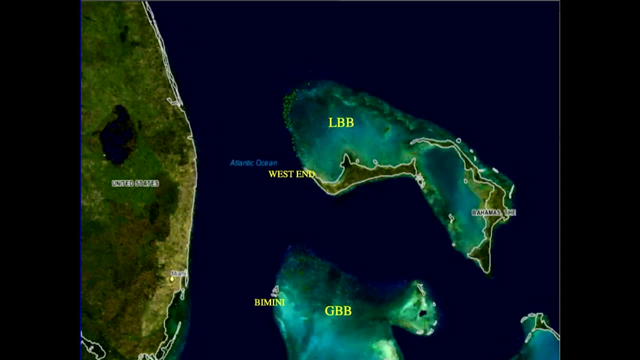 them and re-ID them and track them through their lives. Now you all know where you are in Florida. here We work primarily in the northern Bahamas, historically off Little Bahama Bank, on the top there and West End, and recently down in Bimini, down on a Great Bahama Bank, And it's a great. it's a great place. 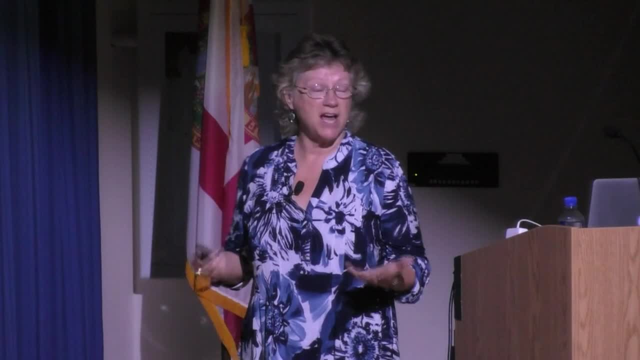 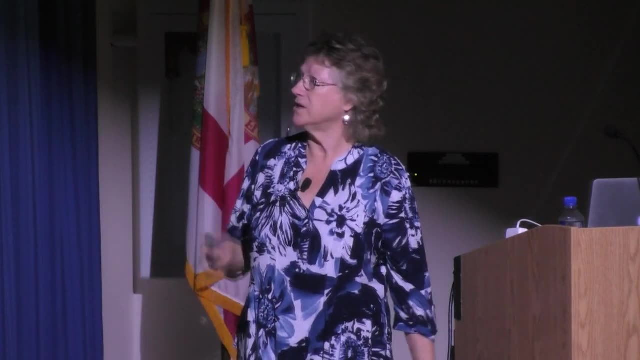 to be a dolphin, but it's also nice as a researcher because the water is shallow, it's clear, it's relatively safe from sharks, so you can be in the water a lot and not die worry too much. we work on a 62-foot power catamaran that my nonprofit got. 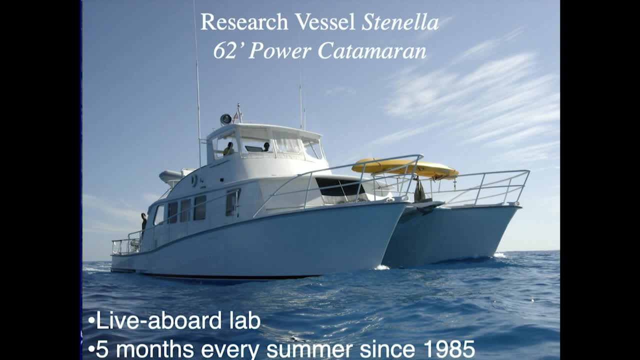 donated in 1992. that was a miracle in itself, which I can tell you about later. so we live, we sleep, we eat on board boat for about 10 days and then we come back to Florida refuel reprovision, then we go back out and we do this five months. 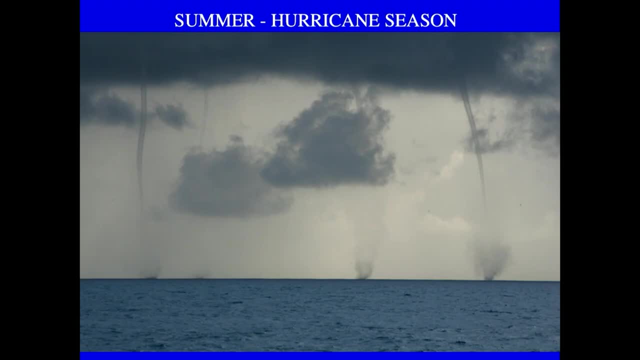 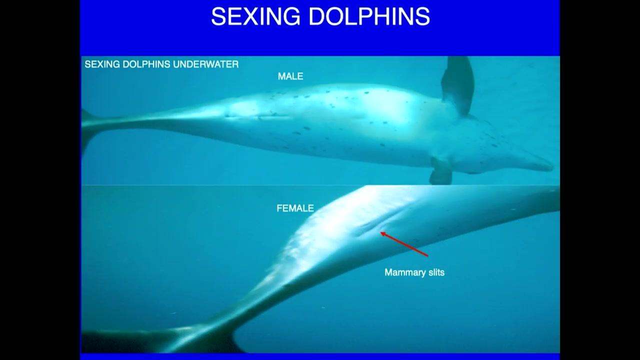 throughout the summer- and, yeah, we work in the summer- it's hurricane season but, believe it or not, it's usually the best weather to be out there, really, because of the direction of the winds and how protected we are by the island masses themselves. now some take-home information if your kids want to know. 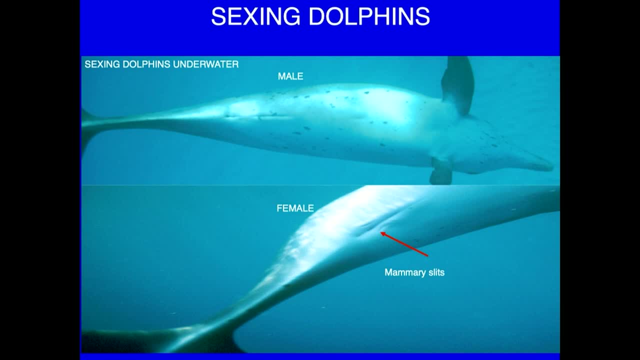 how do you sex the dolphin mommy? basically everything is internal right. so the females have little mammary slits next to their genital slits. the males just have a long slit and a little anal slit. so that's how we sex all these dolphins. so we know. 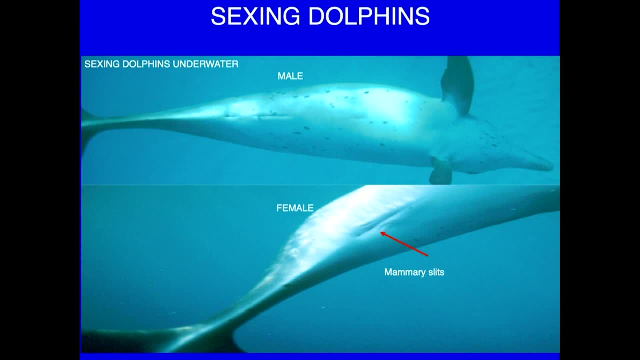 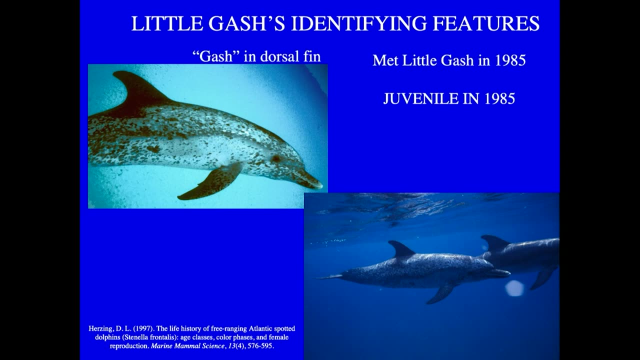 from females, and of course that does not change, at least as far as we know. now. here's an example. so I met this individual little gash in 1985. at that point she had no spots, but she had this tiny little gash in her fin that we 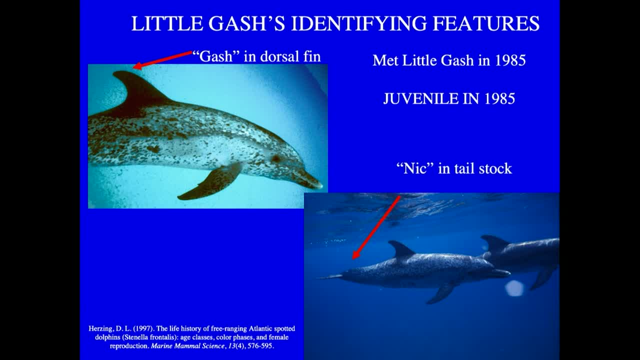 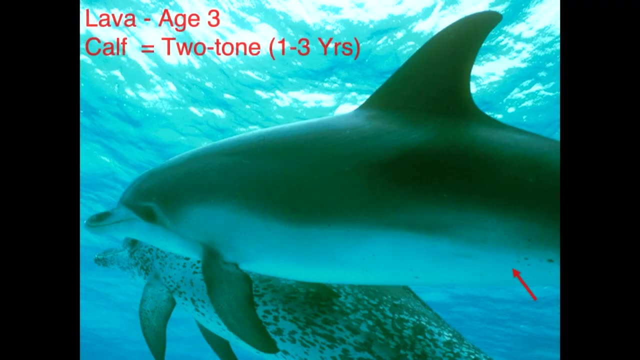 could use for identification. then over the years she got a notch in her tail stock and then gradually she got these spot patterns. so this is how we would literally track an individual, and every dolphin is really quite unique. for example, here's a named lava, she's at age three and she has some spots where 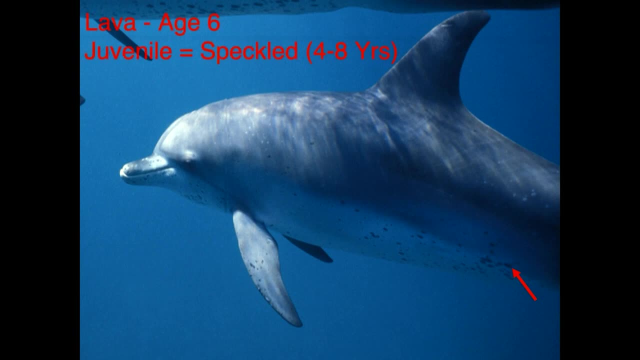 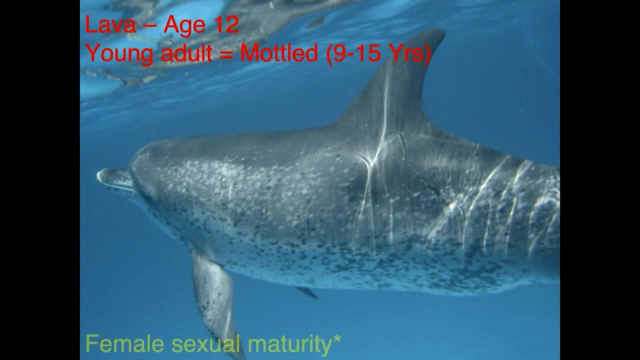 you see the red arrow. now she's age six. she gets a few more spots. we call her speckled and she's a juvenile. in that shot, here she is at age 12. she's a young adult called modeled. this is the age where females become sexually mature and 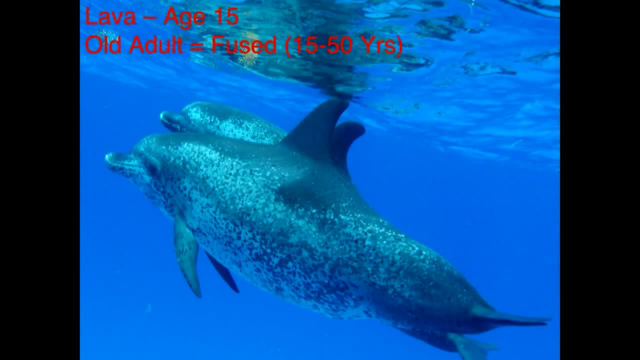 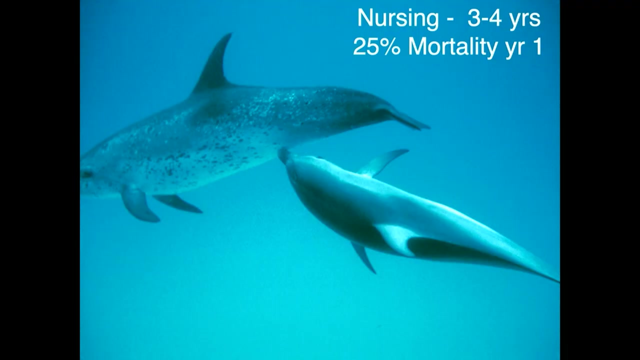 then finally, here's. here's lava at 15. she's an old adult, we call her fused. she's an old adult, we call her fused, and this is the age where the males mature sexually. so the females mature a bit earlier than the males. there's a joke in there somewhere too, I know so of. 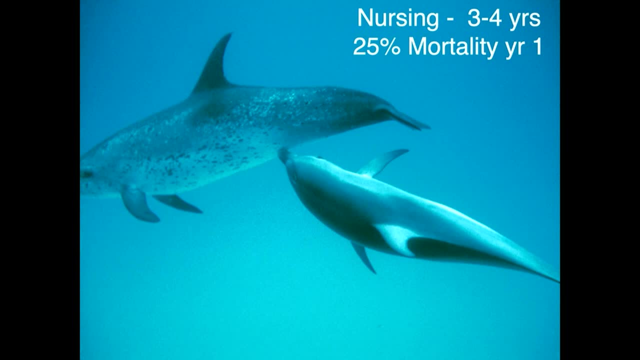 course dolphins are mammals, right, and so they nurse, and specifically they nurse for three to four years, usually, depending on when the female gets pregnant again. so I have three to four years in between births, but the first year we have about a 25% mortality and that's. 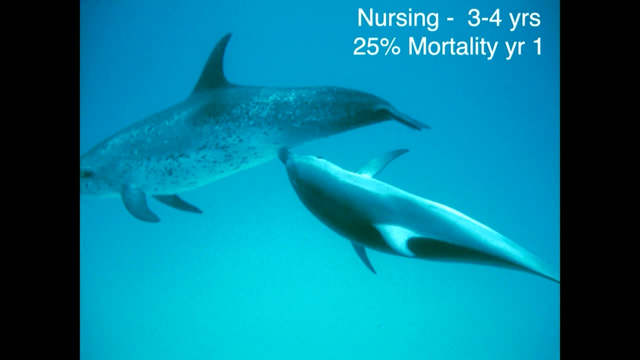 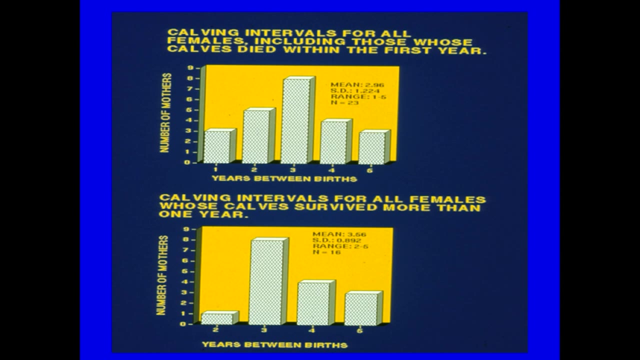 pretty mammalian. but that's just mother nature, right? we lose calves at that age. now this is just a quick little graph just showing that the years between births pretty much averages three to four. on the bottom graph this is calves that have survived more than one year. the top graph: what happens is if a 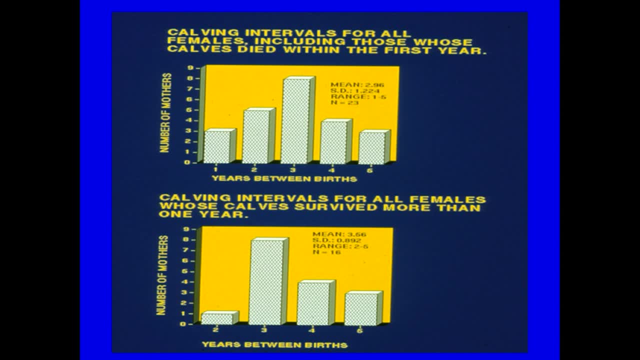 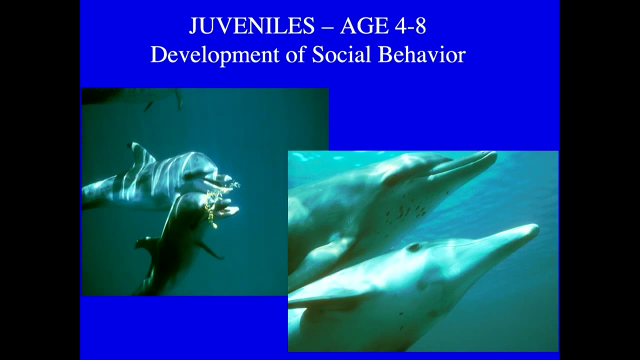 mother's pregnant. she gives birth. the calf dies for whatever reason- sharks or disease. she'll go into estrus quite quickly and mate again. so she'll really have a quick turnover of a year interval, but typically three to four years is the interval for giving birth. now juveniles are about what we 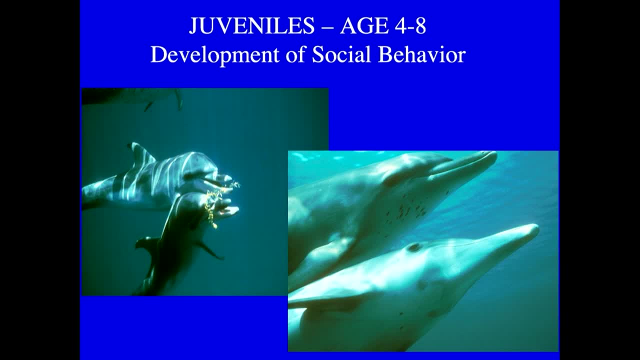 consider them juvenile, about age four to eight. they're kind of away from their moms now and they're wreaking havoc in the society. they're like little teenage gangs running around fighting and making trouble, as you could expect. so they're playing with Sargassum. they're learning how to fight and how to play again very. 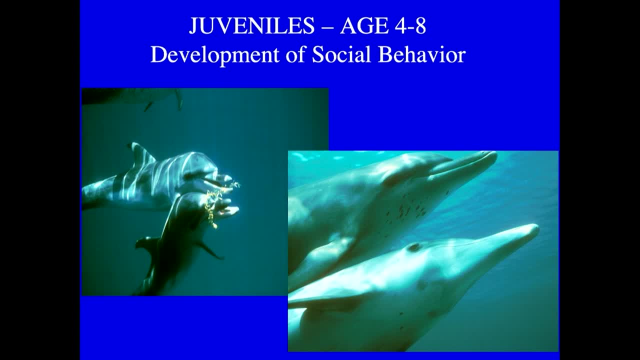 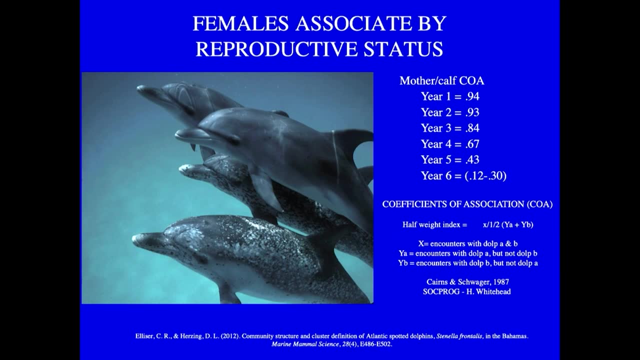 mammalian and very important for their development. They're learning how to become an adult dolphin safely by playing as a juvenile. Now, one thing we know is that females associate by reproductive status. So for example, here you have. you have two adults, Little Gash and Rosemal. So when I went out there in 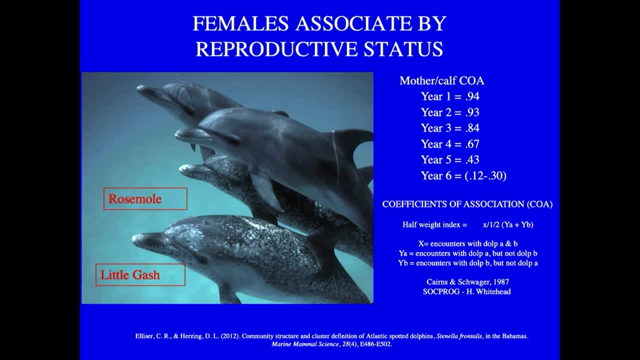 1985 they were juveniles and they were, you know, making trouble like everybody. So then Rosemal got pregnant and Little Gash was still dating the guys, but she, she wasn't pregnant. So they kind of separated, They hung out, Rosemal hung out. 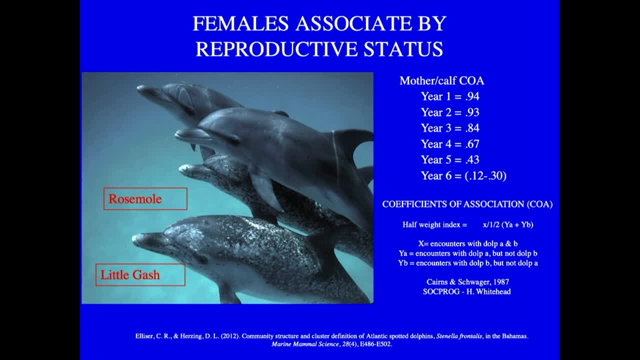 with other females that were pregnant or had calves. Then Little Gash finally got pregnant. They both had their little calves, Little Rosebud and Little Hailey, and then they all started hanging out together, So it's a really interesting thing to watch. As you can imagine, females probably need more food and 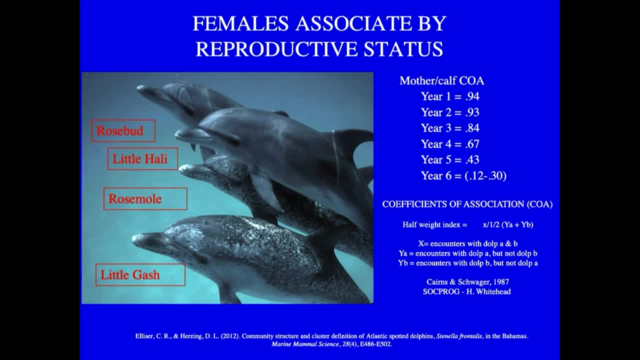 substance when they're pregnant, so they have to hang out where other mothers are, where the good food is. Now we measure this by basically measuring a coefficient of association, which basically just tells us how much they're together. So, for example, a mother and a calf COA in year one is 0.94, which 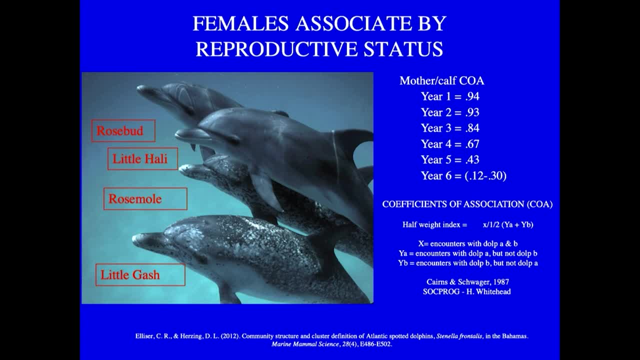 means they're pretty much always together. It drops off year two, year three, it goes down, and then finally year four, which is the year where the mother probably gets pregnant, again it really drops down. They'll still hang out, but not as much. So that's something we know about the. 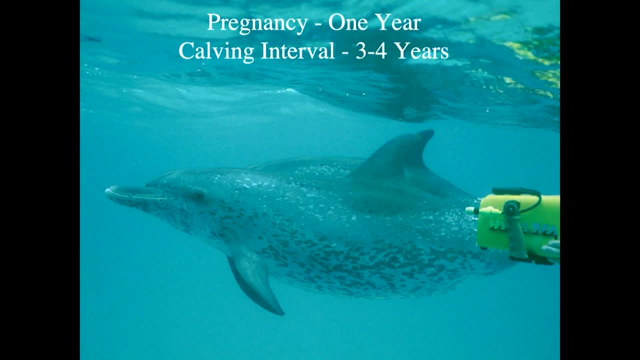 females. Pregnancy is about a year and calving every three to four years. So this is a very pregnant dolphin named Katie. I met her in 1986.. Her mother's Blotches and Katie had our first third-generation dolphin named Kai He. 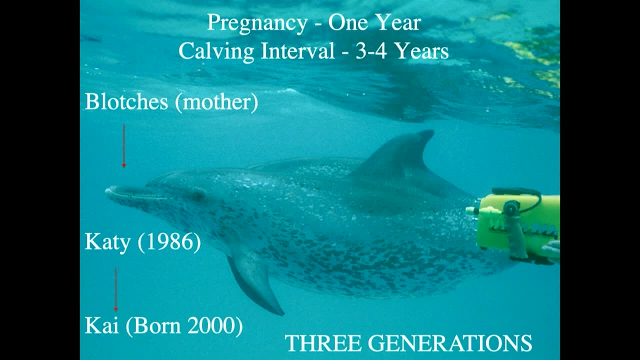 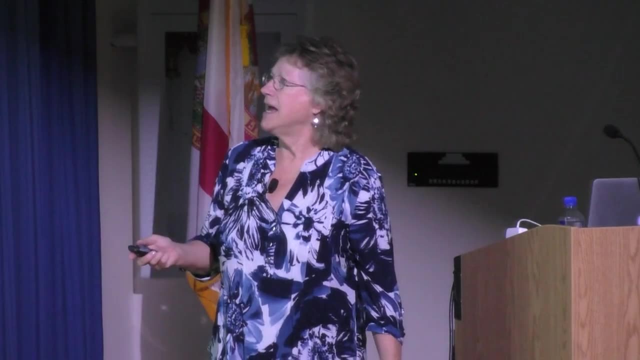 was born in 2000.. So they get really, really pregnant. We haven't seen a birth, but it sure looks like they're gonna pop when we're out there sometime So they can have really extensive family trees. this is an example of blotches Katie's mom. this is. 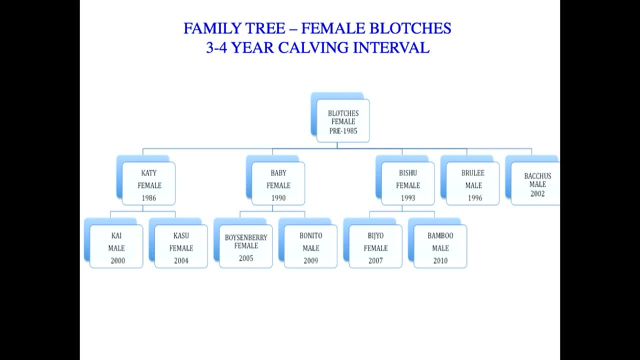 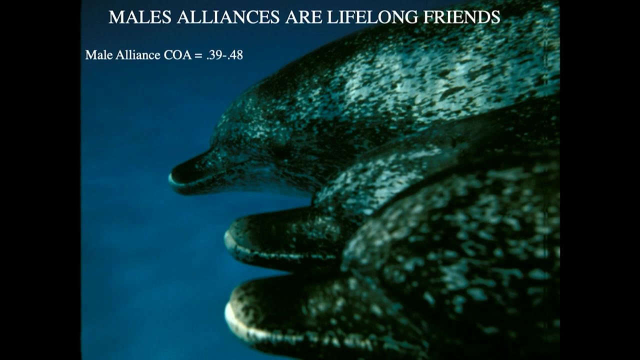 all her offspring and then her offspring's offspring. so those are her grandkids. this is really how we track their family lines. not everybody survives, but we can see who's related to who. now the males are doing something different. the males are forming teams and alliances, pretty much when they're 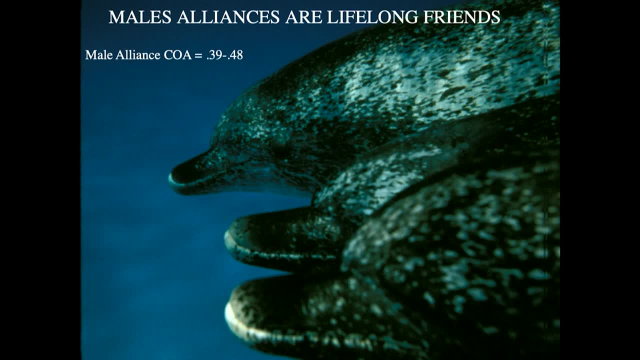 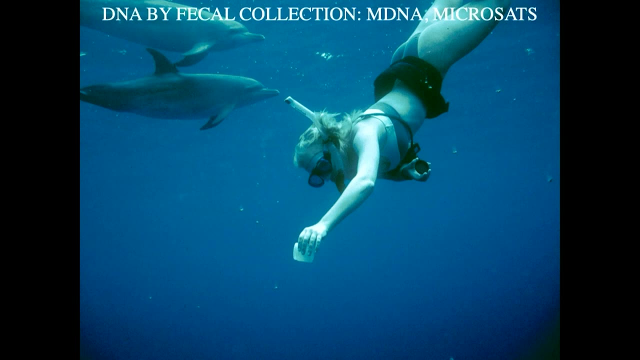 kind of late juveniles. so they've been practicing fighting and getting in trouble, and their coefficient of association is actually the second highest in the whole society. so they're very tightly bonded. the males are now. we really want to know who sires the offspring, so we have to collect DNA for. 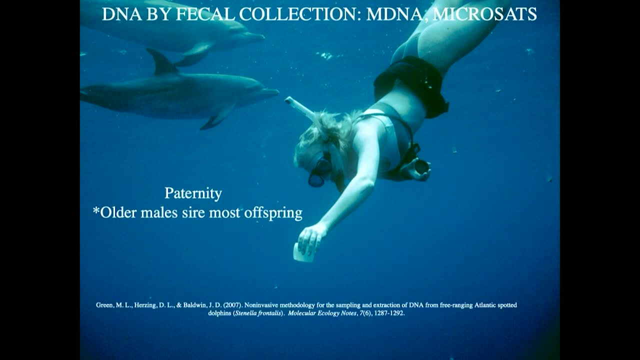 that we basically scoop their poop. these are my, my graduate students. we call them my femme for cows, swimming behind the Dolphins, scooping poop in the water of and we know which dolphin just defecated. and it turns out, if you analyze their DNA- either their mitochondrial DNA or micro satellites, which is used for paternity- it looks. 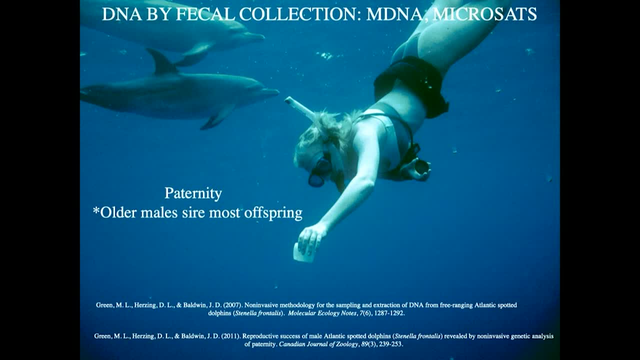 like the older males are siring the most offspring, right, so you may see the younger males, you know mating and engaging females all the time, but the old males, they're the ones that actually you know count as far as siring offspring. now, this is some very interesting data that we're going to look at in just a 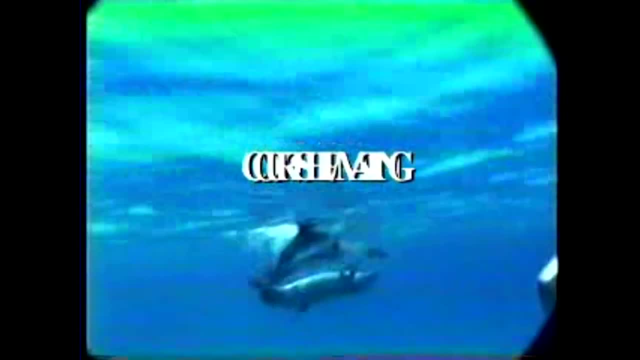 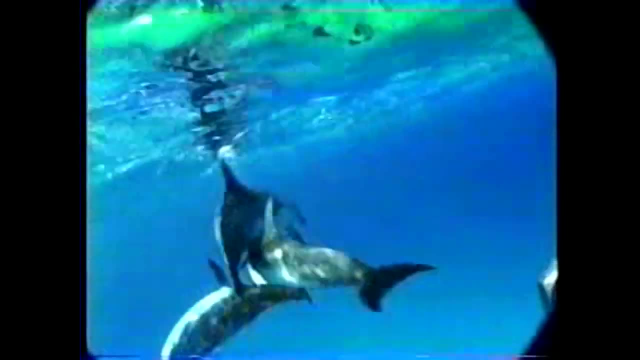 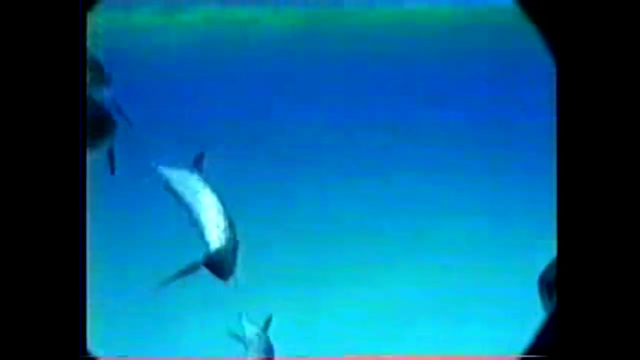 few moments. okay, so this is footage. I hope so. this is old footage, it's not so clear, but it's really cool. so a little gash and her calf, a two year old calf. underneath her, the male is upside down. there's a group of males around. 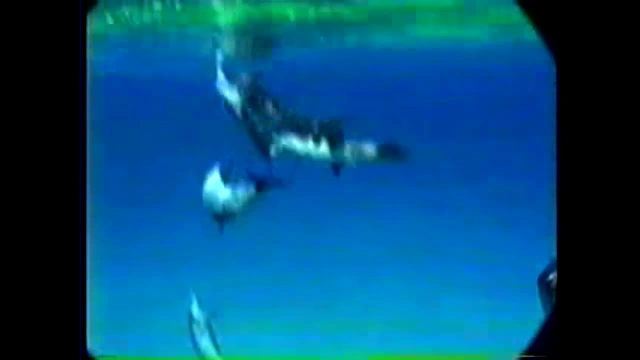 he's trying to get underneath today because that's how they mate, so they stack up underneath her trying to get their chance and have their in. what I think is really cool about this video- it's very easy to know that the what i think is really cool about this video is that when they get their chance and have their in. 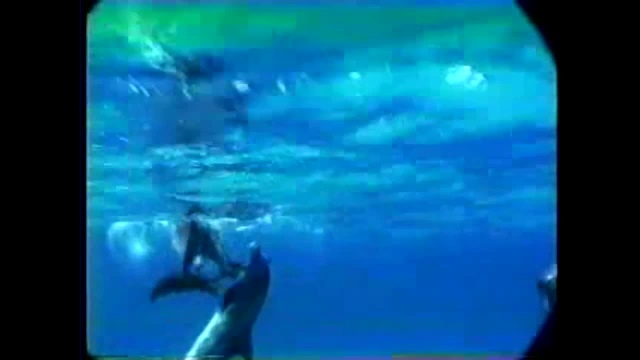 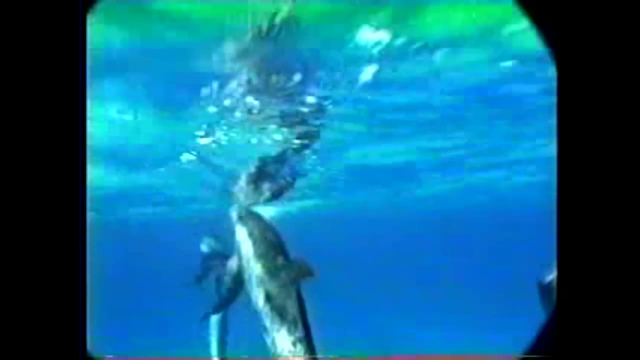 video footage is that when they get their chance and have their in, is that the calf is just in? the way The calf is hearing and seeing everything that's going on, So they're getting exposed to the whole social system, even as a calf. 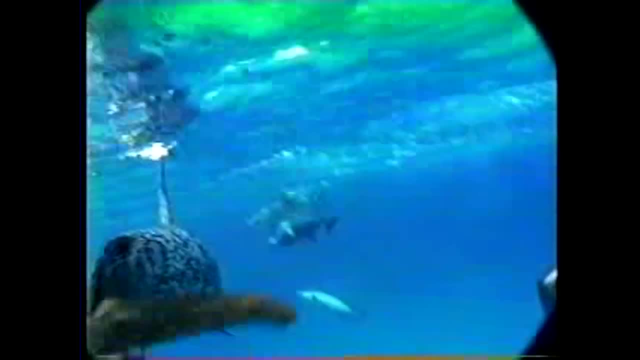 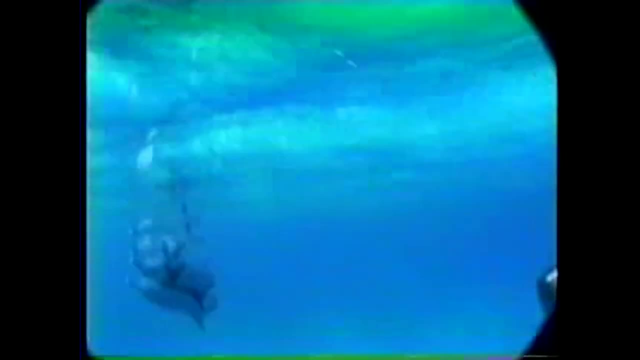 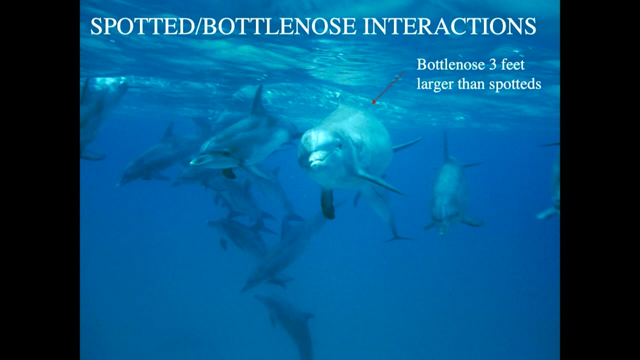 There's a lot of social exposure, So the males just keep trying to mirror her mate with her, And if she's not interested, she'll watch you slap them away. It'll be interesting. Now there are also bottlenose dolphins out in the Bahamas, where we work. 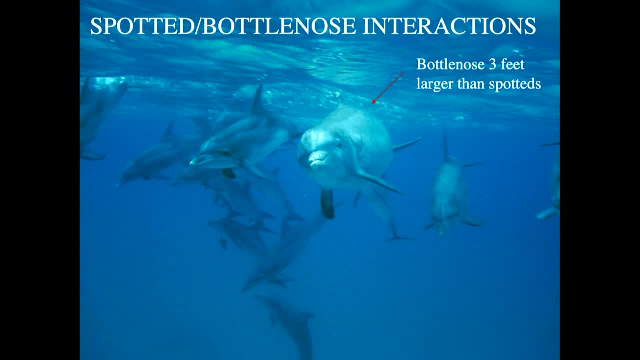 And they're about three feet larger than the spotted And we see them together, And this is something I didn't expect When I went out. I was planning to work with the spotted dolphins primarily, But we see them together about 50% of the time when we see the spotted. 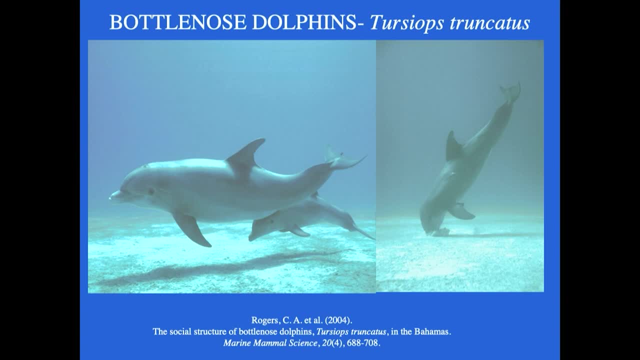 So they have a pretty interesting relationship. I've had graduate students that have studied just the bottlenose dolphins and they have kind of a similar life history. They give birth every three to four years. They form maternal groups and male alliances, that sort of thing. 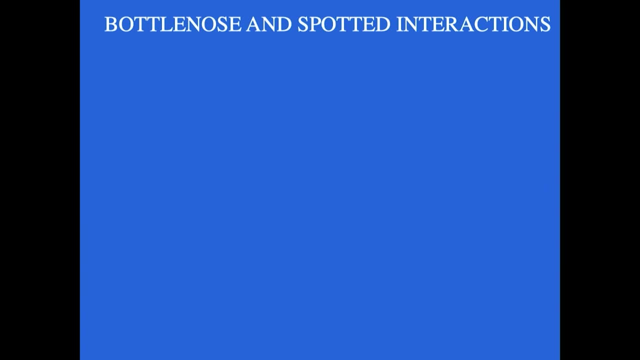 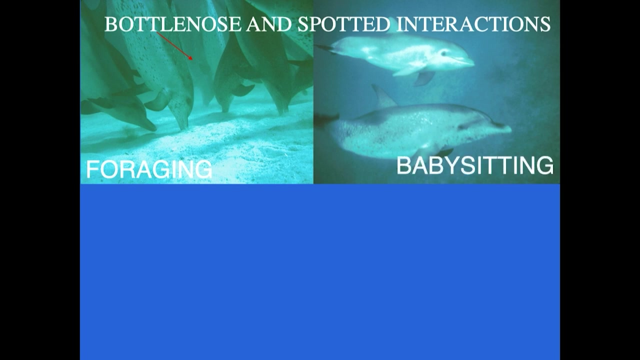 They dig in the bottom for fish, like the spotted do, But what's really interesting is that they forage together a bit. Not very often That red arrow is pointing at a bottlenose dolphin amongst the spotted. But the young female spotted dolphins babysit young calves. 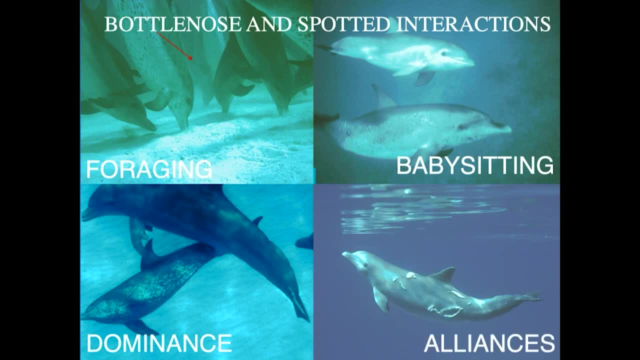 Of bottlenose, which is really interesting. So interspecies babysitting On the left corner, you see bottom. you see male bottlenose dominating. It will mount and copulate, with male spotted as a dominance. So they're actually trying to get at each other's females, which is really interesting. 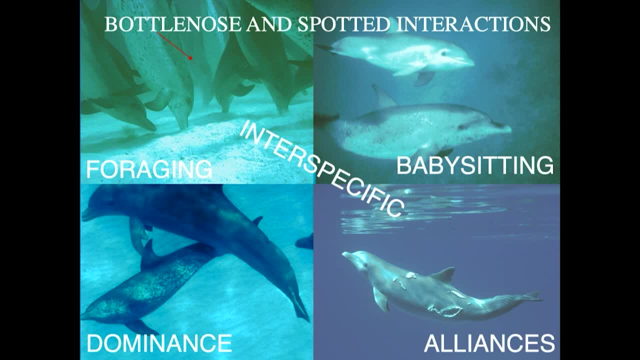 And they do hybridize a bit. So there's a lot of competition for mates, regardless of what species- Now the male alliances of both species- they will also help eachother. So if they're fighting, so if we have a group of bottlenose fighting spotted and a big shark comes in the area, 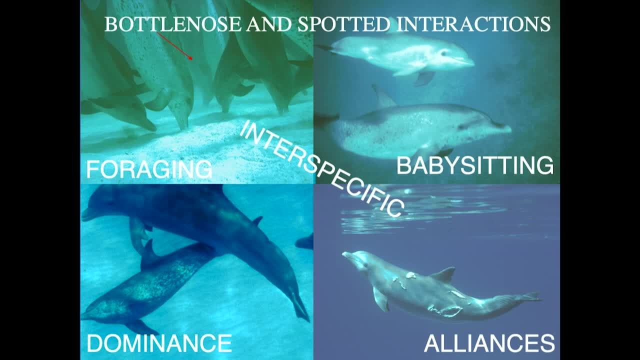 they'll like stop fighting. they'll form a group and they'll chase the shark away. So it's pretty cool. They really know each other as neighbors and they fight, but they also help each other. So very cool interspecies behavior. 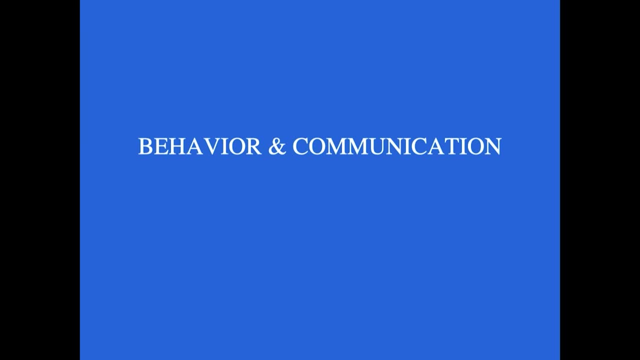 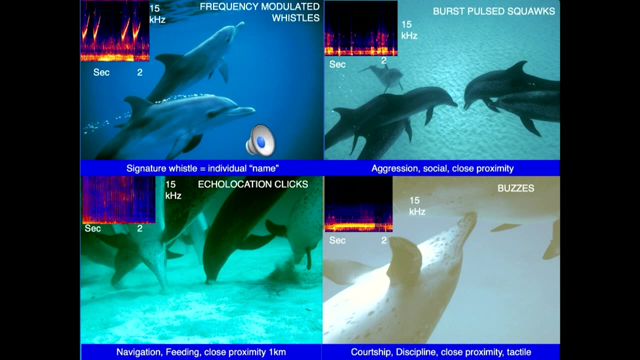 Now we do know quite a bit about their sound and their communication. In the upper left we see a signature whistle which is a frequency, Which is a frequency modulated whistle, And this is like an individual name, So they have specific names. 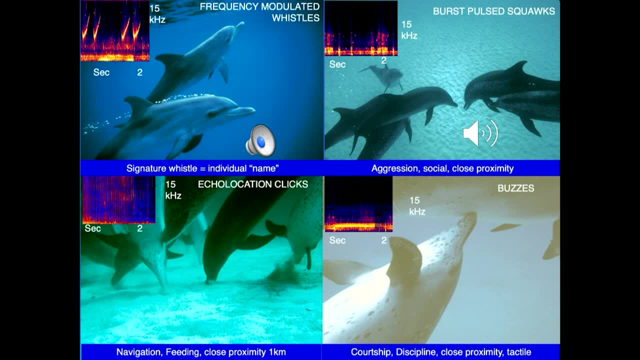 On the upper right- this is that was a burst- pulse squawks. They're fighting sounds. basically, On the bottom left we have echolocation clicks, which is their sonar for digging in the sand and navigating. On the bottom right we have buzzes, which are considered. they're kind of clumps of clicks. 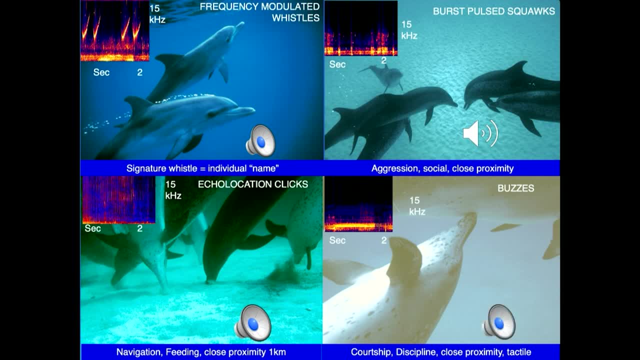 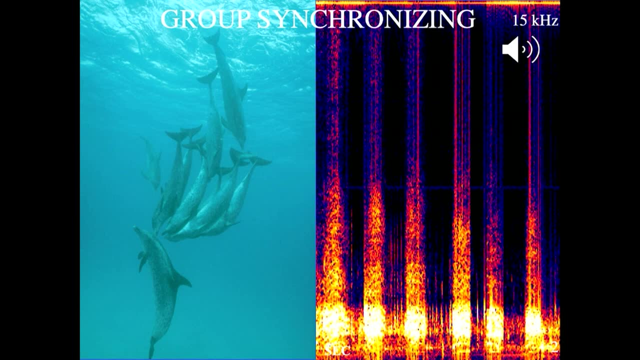 They're disciplinary buzzes, buzzes they use to chase sharks away. One cool thing that the dolphins do, So they synchronize their vocalizations. like you just heard, Those are synchronized squawks, And so they're kind of like a football huddle. 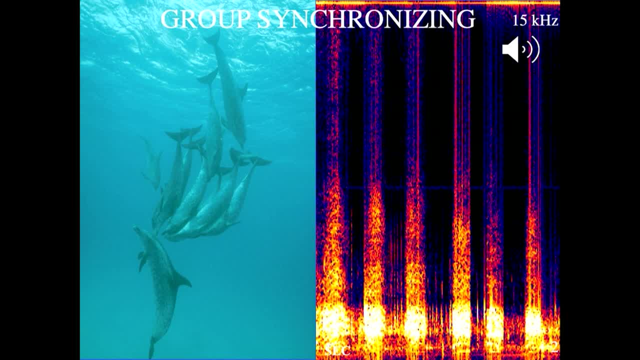 They'll synchronize their physical behavior and their vocalizations And this makes them kind of look bigger and badder, But it's pretty pertinent to their lives. Now. this video is really cool and really rare. This is a group of bottlenose dolphins. 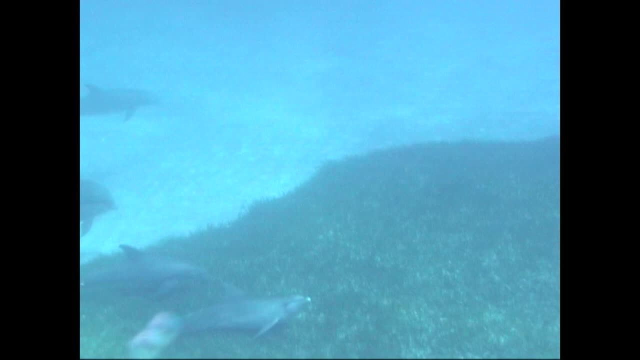 And what you're going to see and hear. you're going to see them synchronize their postures. They're going to kind of turn to each other and whistle and squawk and then turn away, And then they're going to turn and whistle and squawk. 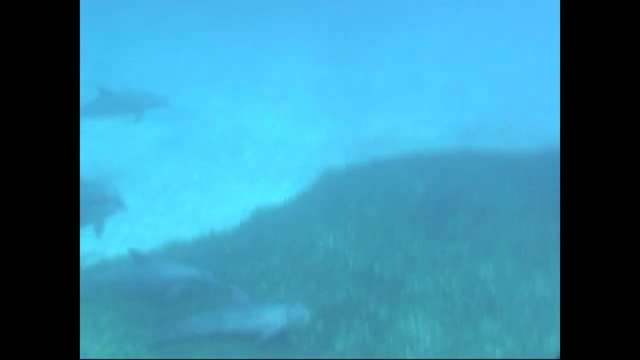 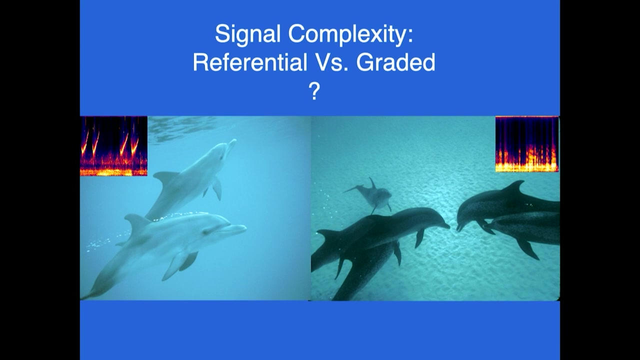 And it's very rhythmic. It just gives you an idea of how specific they use this for. I don't know what they're saying, But they're saying something interesting. Now, one of the challenges with studying specifically acoustics of dolphins. 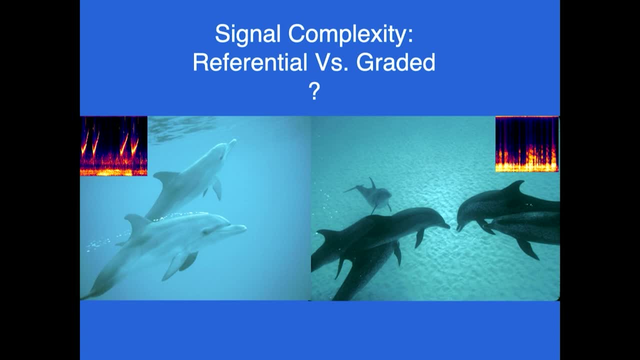 well, there's many challenges, But one of them is we want to know if they have something like a language or they have some kind of order and structure to their sounds. Now, in the larger field of animal communication, what we're looking for is either a referential signal or a graded signal. 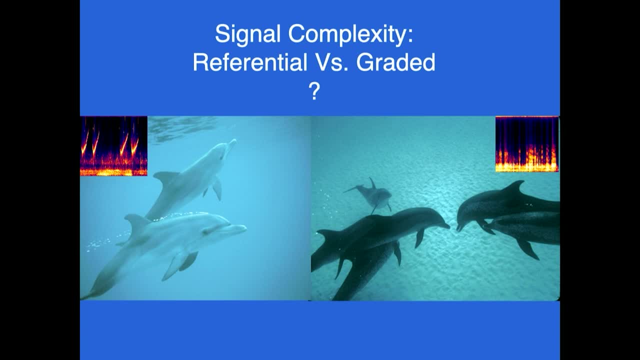 What that means is so a referential signal just means something that's labeled Like your name is a word. right, It's a word, It refers to something. So on the left side you see those signature whistles again And they're whistles. 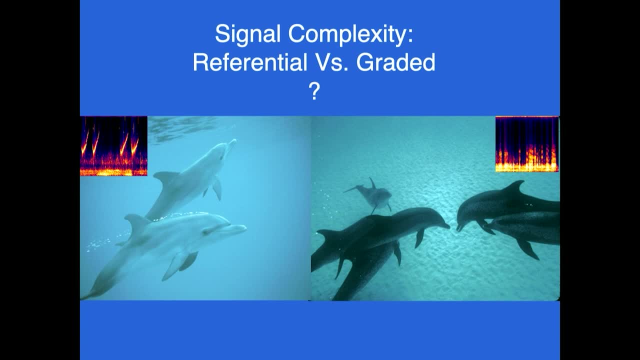 You basically would hear those whistles in the water. They sound like, Right, They're human hearing. They're kind of read like a musical score, right? So frequency time And those are considered referential signals. So they're names of specific dolphins. 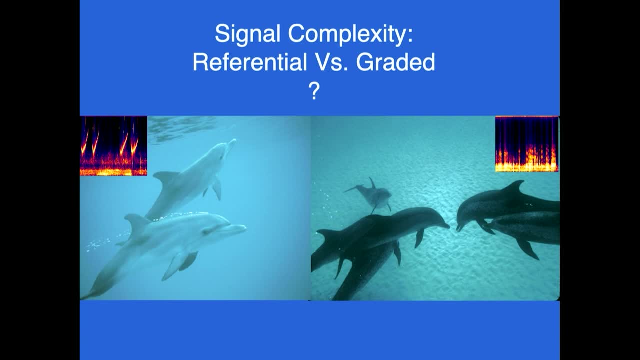 On the right, the squawks and things you've been hearing. that's considered more of a graded signal, which means it's just expressing emotion and motivation of an animal. So we have both. I'm talking to you with words, but I'm flailing my hands. 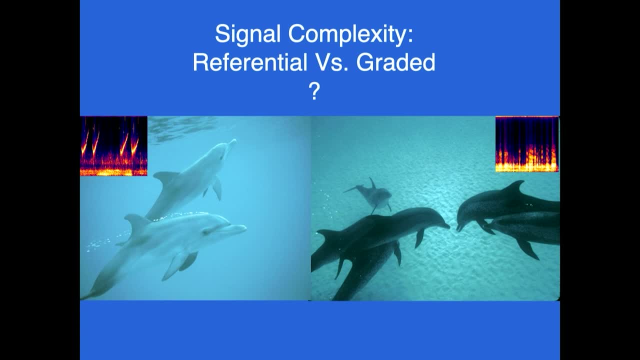 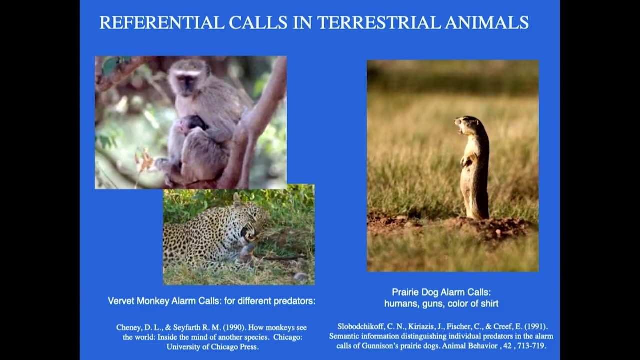 and I'm talking loud and talking excited sometimes, right, And these are all signals that modify my words. So we don't know what a lot of animals have, and specifically dolphins. Now we've known for many decades that some terrestrial animals 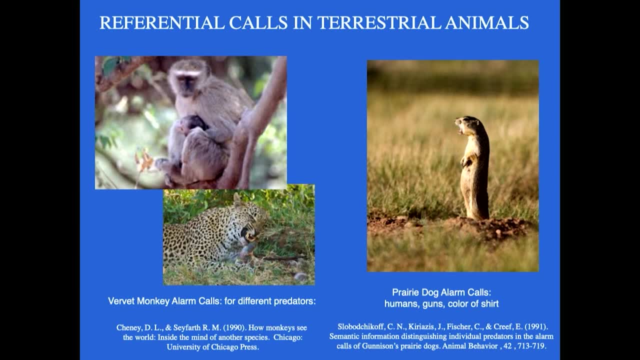 specifically vervet. monkeys have signals for specific predators, So they can make a specific alarm call that tells their buddies that there's a leopard chasing them or there's an eagle in the sky, and then their friends can take the appropriate action. We know this from prairie dogs. 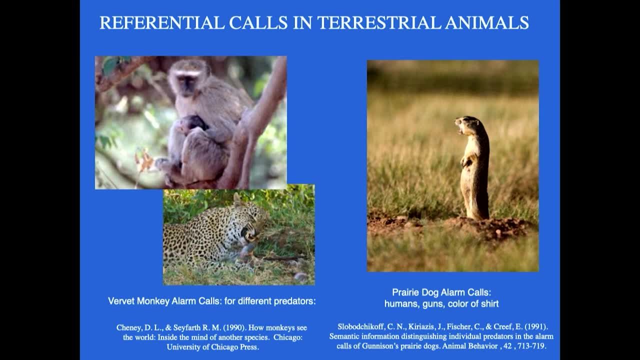 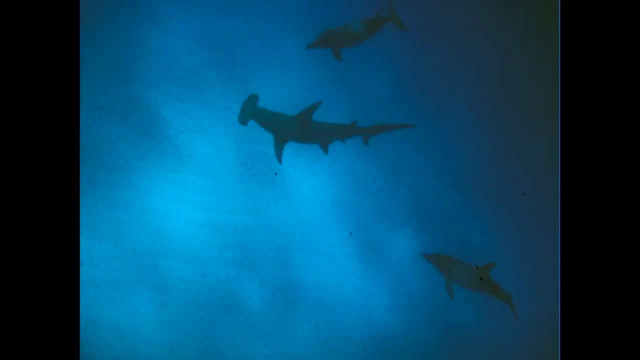 Actually, some incredible work has been done with prairie dog alarm calls to signal the colony about there's a human walking in the field with a gun. Just amazing work. So we know terrestrial animals do this and it's survival right. It's a smart thing to be able to refer to something specifically. 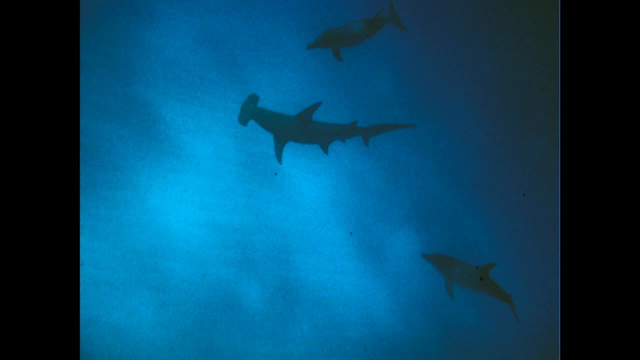 So you can imagine it would be pretty important for a dolphin maybe to have a label for a type of shark. This is a hammerhead shark. Two juveniles are chasing them because they're just fun and harassing them. But you can imagine it would be pretty important. 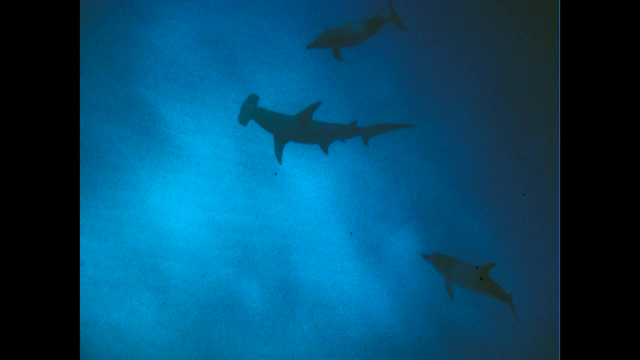 for an animal to signal: oh there's a big tiger shark who's going to go after us versus a nurse shark that's harmless, for example. So we look for those kinds of signals. We look for those kinds of things to try to get a handle on what their communication system is like. 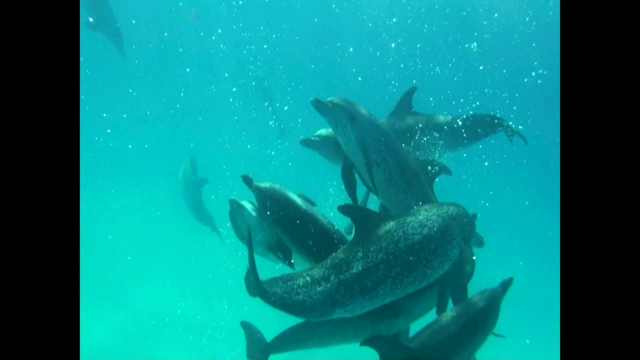 Now this is just a group of spotted dolphins fighting. I just wanted to give you a sense of what that is. And again you're going to see kind of two groups separate. They're going to take head-to-head stances again, which is mammalian and kind of aggressive. 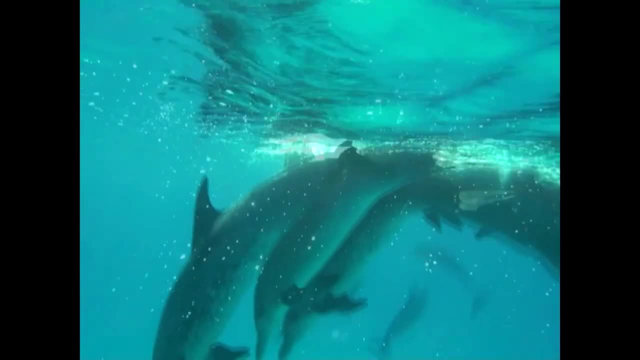 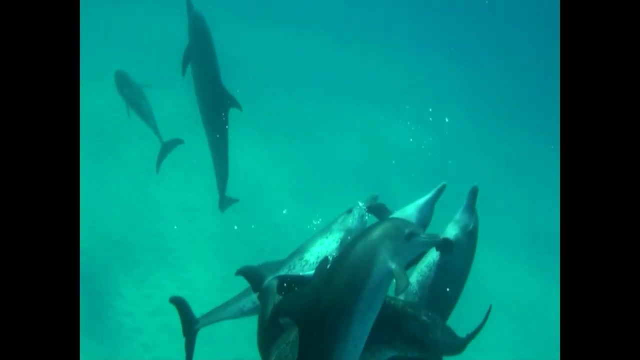 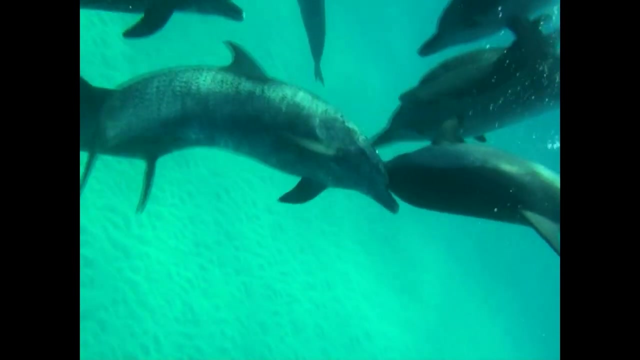 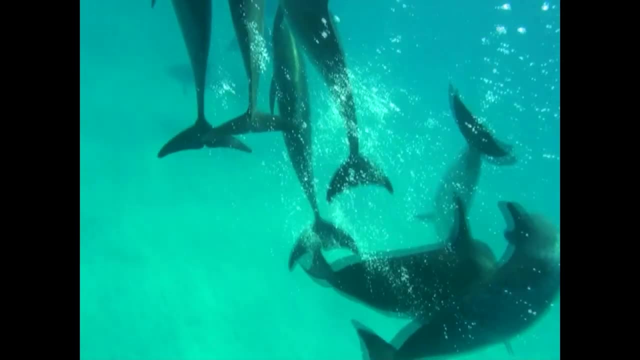 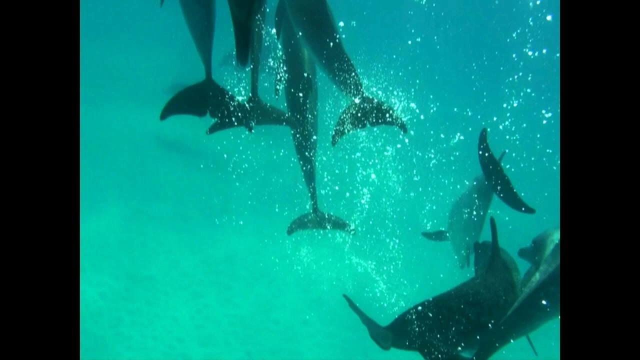 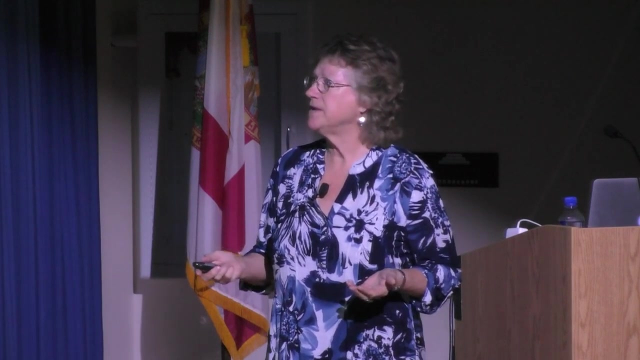 They're going to squawk, And then they're going to squawk. So how are you going to interpret all this? It's a bit of a muddle. I will tell you right off. there are two big challenges working with dolphins. 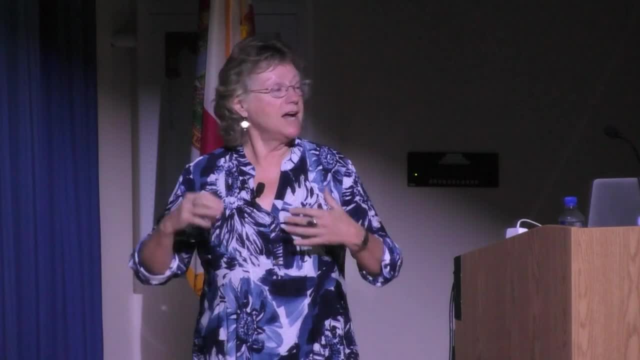 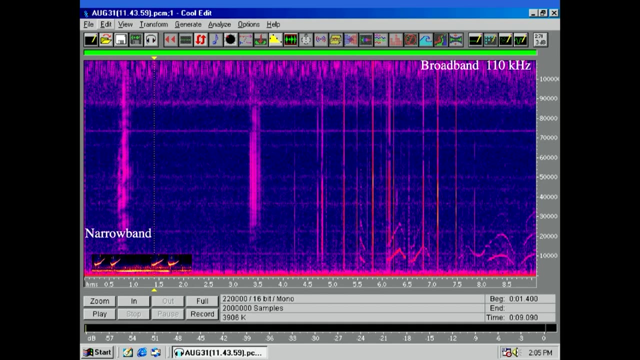 and they involve number one, looking at high frequency signals, right, So we know dolphins make echolocation, that's really high ultrasound, like bats et cetera. So for example, this spectrogram sound picture you see on the bottom left where it says narrowband. 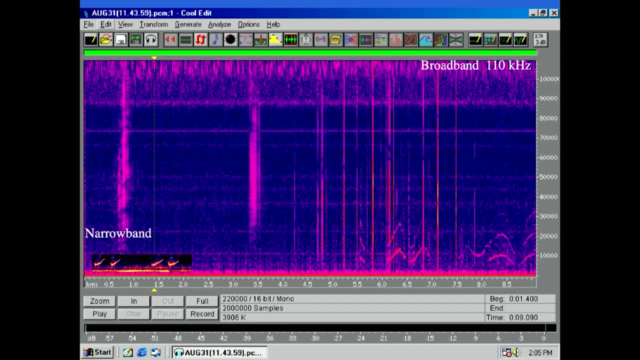 those are the whistles you've been hearing. That's our hearing range there, about to 15 kilohertz kind of max. The rest of the image is an image of sound collected to 110 kilohertz way above our hearing. 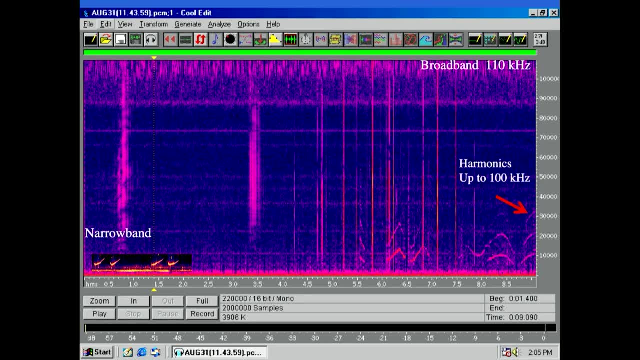 And what you start noticing is number one: you see harmonics that are created naturally, but harmonics which gives cues to the animals. You also see, we knew their clicks were broadband. We've known that with the Navy forever. But what we noticed is also: there are places. 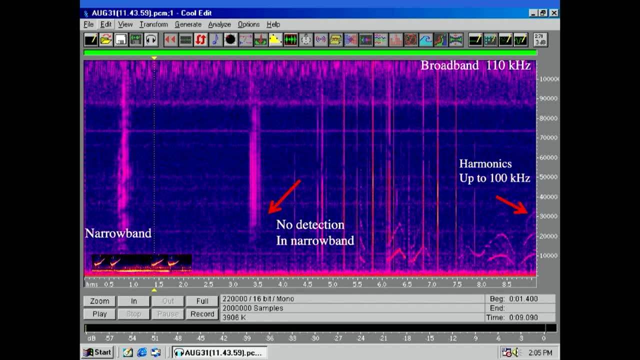 in our sound files, where there's nothing in the lower frequencies, which means if we were only recording in narrowband, we wouldn't even know a sound. is there right? So it's like studying any animal: You have to know what its sensory system is. 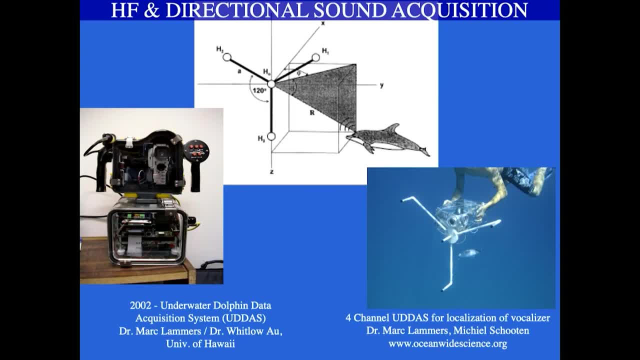 and the range of information. Now the other big thing is we wanna know who's making the sound when it happens. right, You just saw that muddle of dolphins. So we've worked with various colleagues over the years. We finally have a prototype in the water. 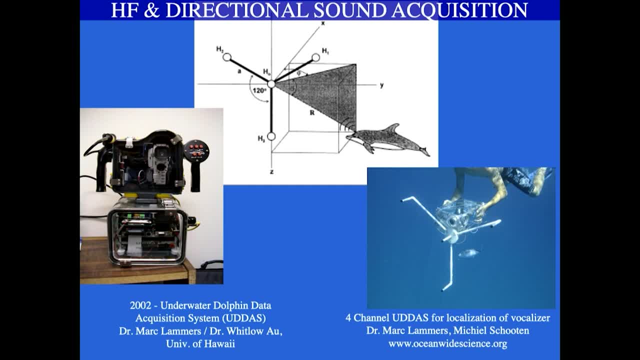 It's basically a unit on the bottom right, You see. it's a hydrophone array with four hydrophones and a video camera in there, And basically what that array is doing it's recording sounds coming in at different times and then it can localize who's making the sound. 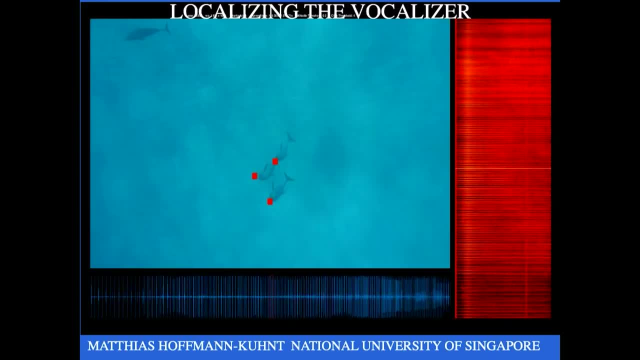 And then it puts a image on the video after it's processed. So all those little red squares are showing us that each dolphin is making echolocation clicks. So it's a start. So what we wanna do basically is look at- okay, mothers and calves. 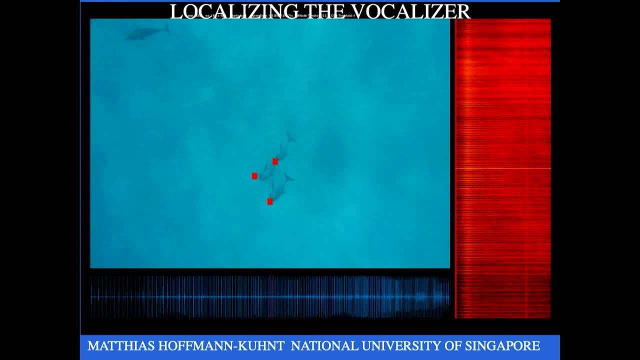 when they're whistling at each other, does the mother whistle and then the calf, or how does that kind of interplay? Or if a group of dolphins, if a dolphins is fighting, is one dolphin making all the squawks and the threats? 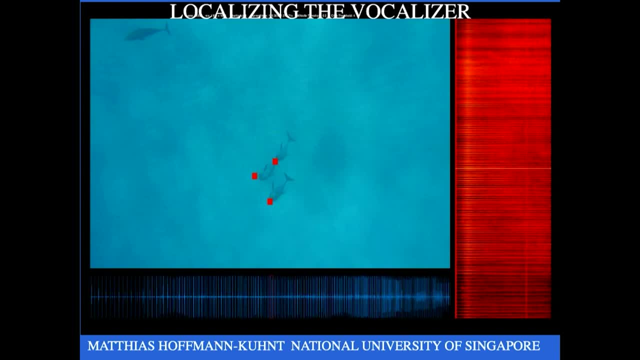 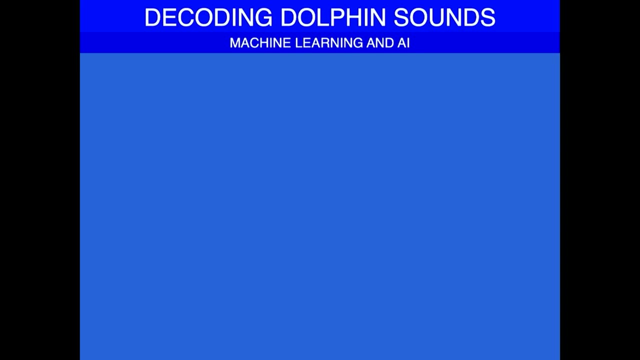 or is it a bunch of them? So a lot of unanswered questions, honestly, but you need the technology in the water. Now, one of the really cool things we're doing right now, and I can't probably go into too much detail. 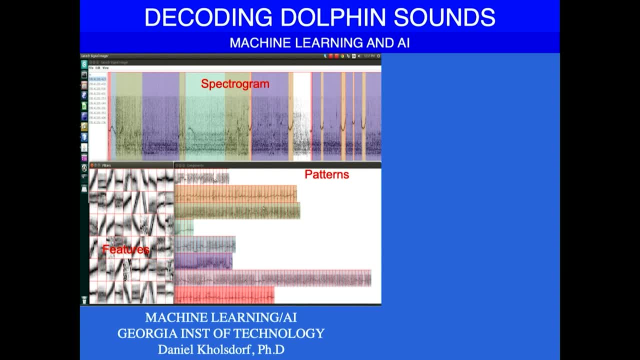 but it's using machine learning, which you all know. you've heard of this artificial intelligence, to help us label our spectrograms. so that top picture you see is labeling by color types of sounds that the computer has coded with our help a little bit. 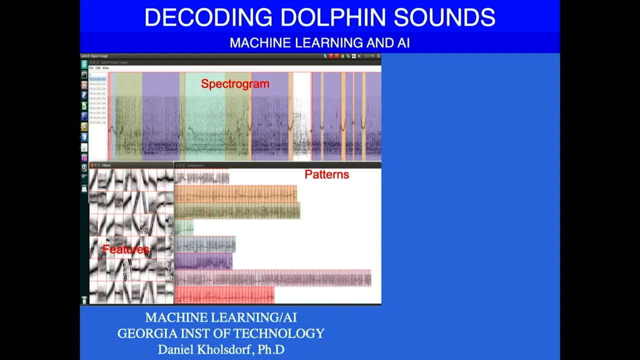 And then it pulls out patterns. So where you see on the bottom, you see patterns. each of those colored rows is a type of sound that the computer has said: these are all the same, so I'm gonna make them all brown or I'm gonna make them all green. 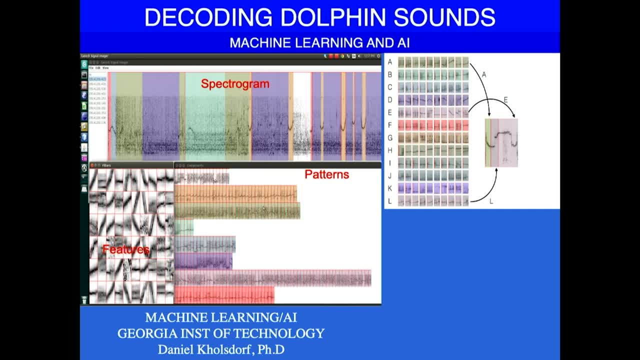 Then what we can do is start looking at the orders of sound types. So sound type A is followed by sound type L, followed by A. So sound type A is followed by sound type L, followed by A by E. So it starts looking at what we would have phonemes in our language, For example. 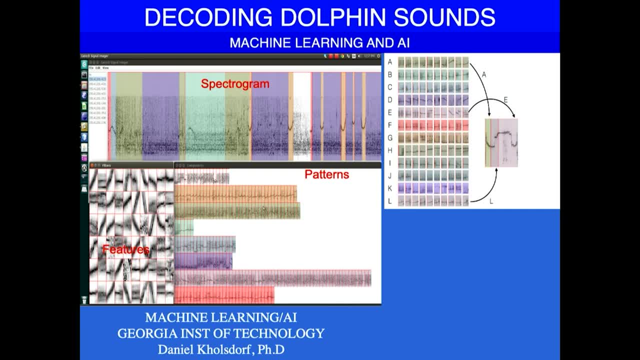 we'd look at that process- you know what follows what- And then we can look at really advanced aspects of what kind of rules or order are there in these patterns? If A is followed by B, it's followed by A, D, D. Is that a specific sequence that a mom is producing? 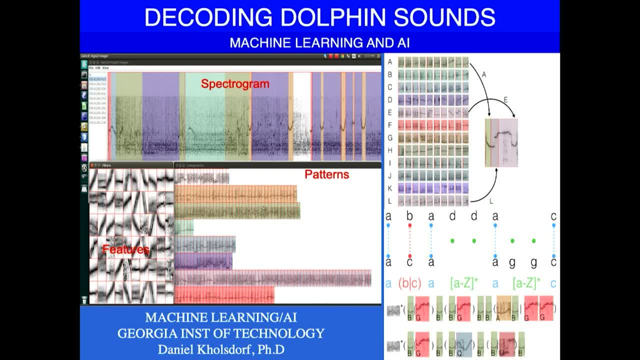 to her calf. So it's really cool work but it's really difficult. I tell you, I've learned a lot. I work with a group of computer scientists up at Georgia Tech primarily, and I've worked with multiple students of theirs And it's exciting work but it's really really challenging. 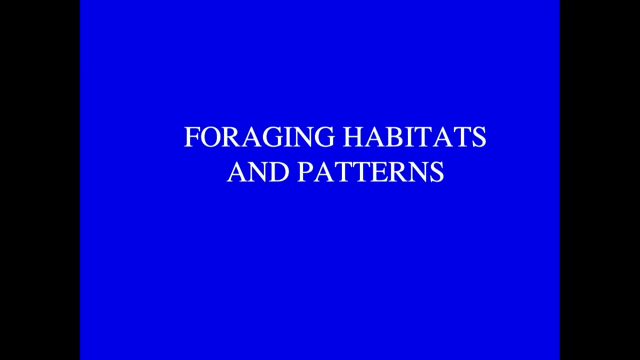 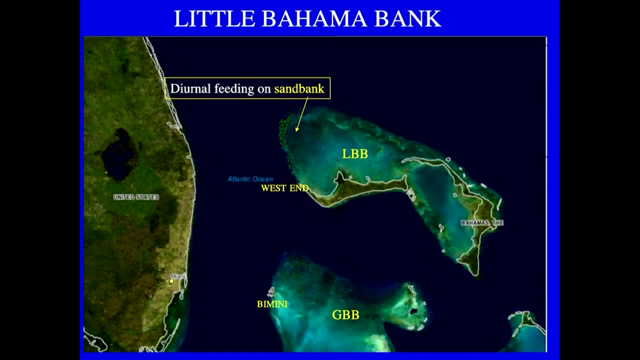 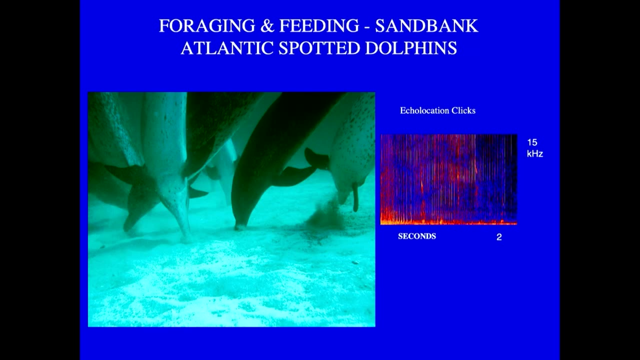 in many ways And I'm happy to talk to you later in more detail if anybody's interested in that. So the dolphins spend a lot of their time feeding during the day on the sandbank And this is, like you know, 10 feet to 40 feet kind of depth They love to do. 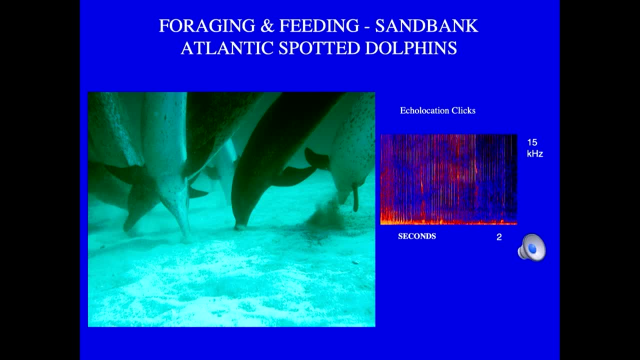 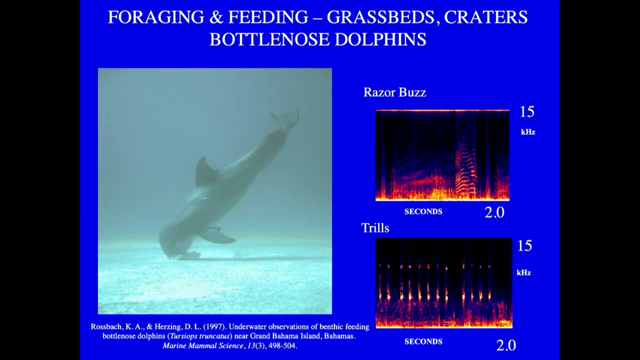 They dig razorfish. They use their clicks under the sand to find the fish. Sorry, We really tried to lower the sound. I don't know what happened. I think that's the last nasty one. Bottlenose also dig in the sand. They use a couple unique sounds: razor, buzz. 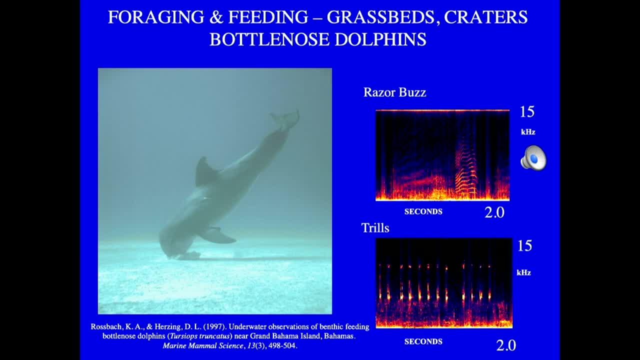 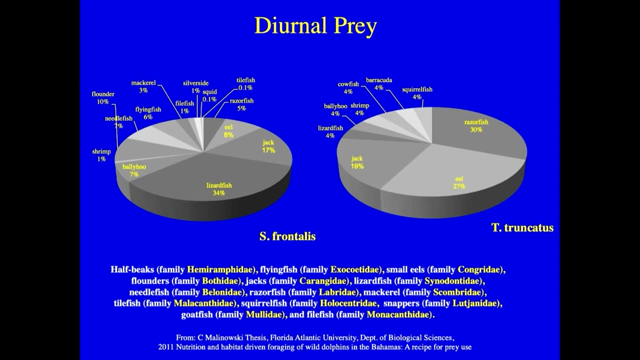 which sounds like a shaving razor and trills- I call them digital trills- And bottlenose are digging for really deep fish like eels, whereas the spotted are kind of going after flounder and razorfish primarily. They have different diets. This is from one. 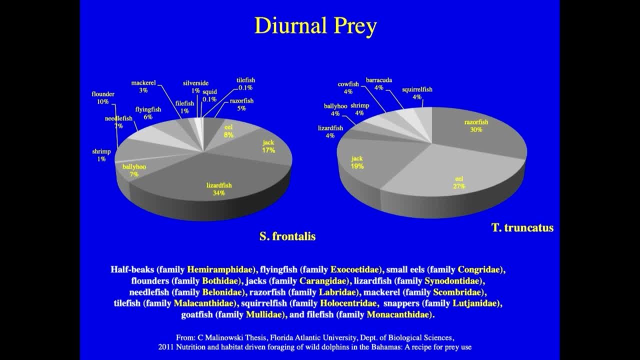 of my master's students, Chris Malinowski. Over the years he sort of tallied what sort of fish we saw them eat. So they have a pretty good variety of fish, just quite different. Like I said, the bottlenose are digging deeper in grass beds. They're going deeper into the 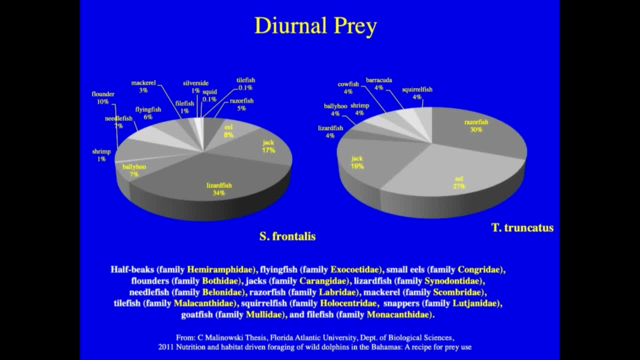 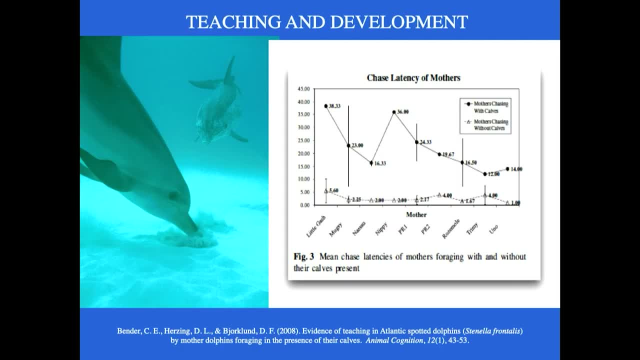 sand. They're going for eels jacks sometimes, where the spotted are eating lizardfish, razorfish, ballyhoo that sort of thing. So they have a pretty good diet. Another cool project one of my students did was looking for teaching right. So how do? 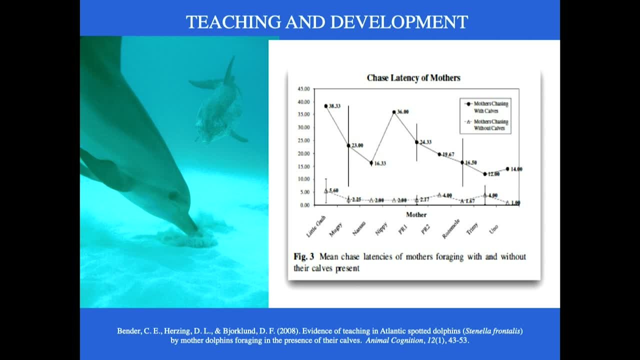 you measure teaching in dolphins? So she took our video and she said: okay, I'm going to measure the time that the mother spends around the calf chasing a fish, or versus when the mother is alone chasing fish without a calf. And when she put the data together, what you 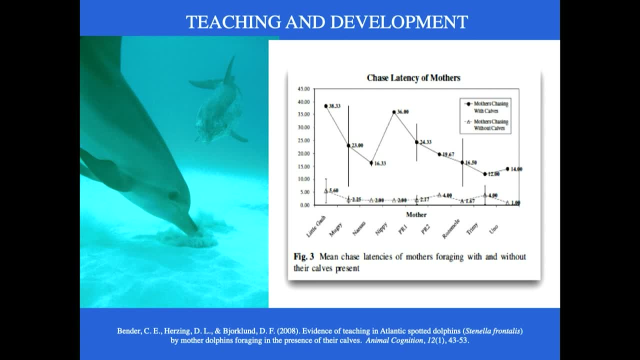 see is on the horizontal. you see the names of the mothers, Little Gash Mugsy, et cetera, et cetera, And the seconds that they spent. when I'm going to point it with a laser pointer on this bottom data line here, the number of seconds. it was really quick, of course. 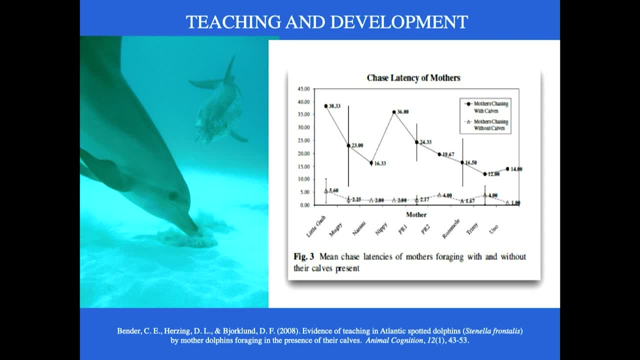 when they're just eating themselves, But when they're with their calf, these extreme, extreme separation takes them a long time. So basically teaching them, encouraging them, chasing up the fish and then letting the little calf chase it, eat it. So this is how they learn And this is considered teaching. 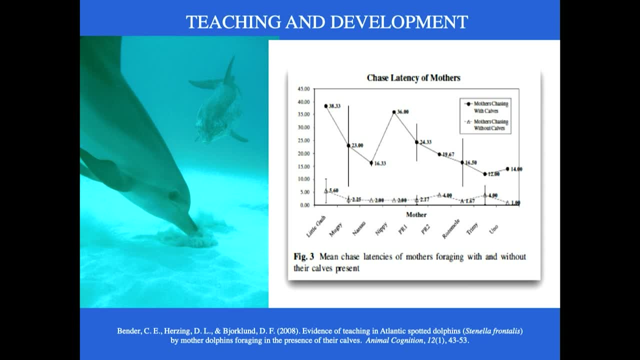 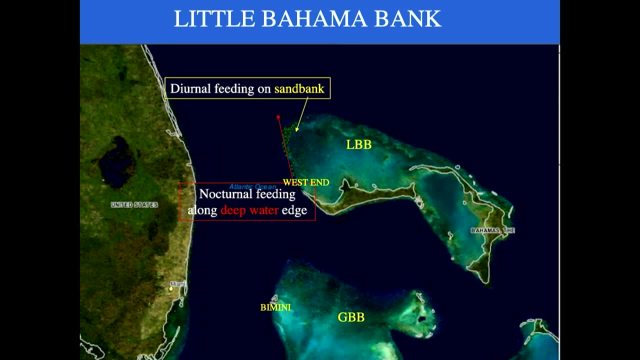 in all definitions of scientific terms. anyway, Now, at night the dolphins also have a pretty interesting life. They go off the shallow bank, the western side of the sand bank, and they drift along the deep water to feed at night. Okay. 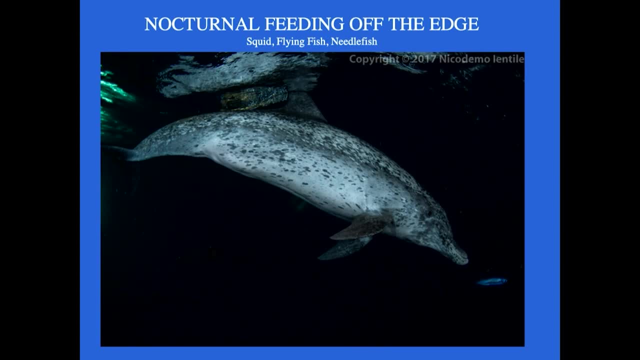 And here's a shot by a colleague of ours, Nick, And they are chasing flying fish and squid very deep in the water and they spend pretty much all night doing it. So they are just. this guy looks kind of fat, huh. So anyway, fatty fish squid, that's really one of the 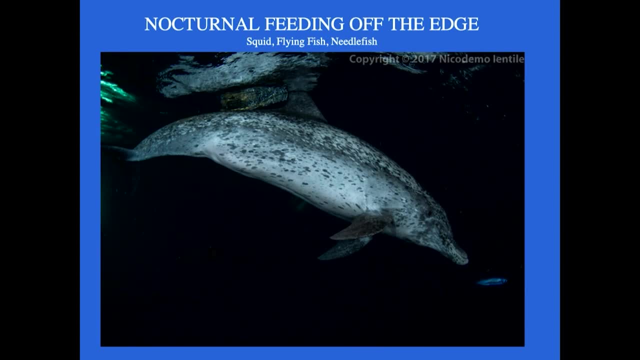 main sources of their food. I think the daytime feeding, I think, is more like snacking- resting dolphin potato chips, I don't know something like that, But they definitely can. Okay. Okay, They're definitely cashing in at night when they're feeding, And this is kind of small. 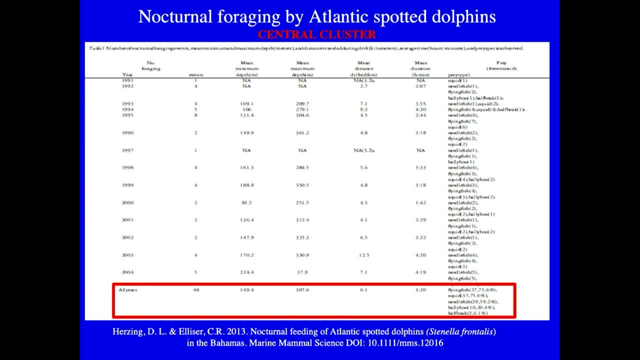 for you to see. but basically this is just showing that you know they can be found somewhere between, you know, 300 feet and 900 feet of depth, usually on the sand bank, And they'll drift, you know, for hours and hours. We've done some all-night drifts with. 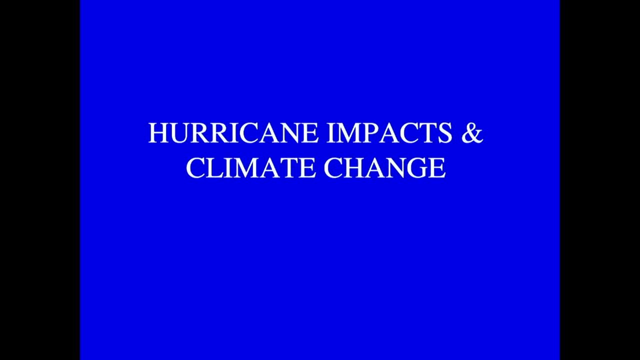 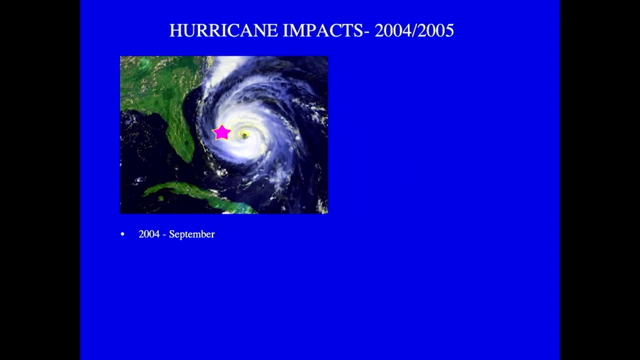 them and they just keep drifting and eating. Now we've had a few natural experiments on the sand banks- Not that we liked it, but I just want to talk about some of those impacts. So the hurricanes of 2004 and 2005 were pretty. 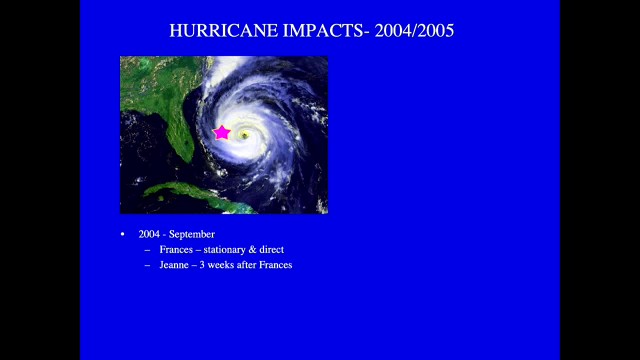 intense. As you know, they hit Stewart right. They hit right here. The pink star is our study site And, for instance, the first storm was stationary and direct. it hovered over our study site for hours and hours and hours and hours- actually a day and a half Gene. 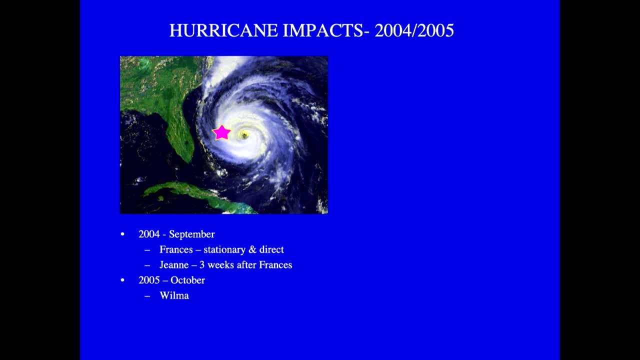 hit three weeks later and then the next year we had Wilma, which was a storm from the Gulf of Mexico, Mexico, but it came over also to the study site and when we got back out to look to see how our dolphins did, we found that we lost 30% of both species. 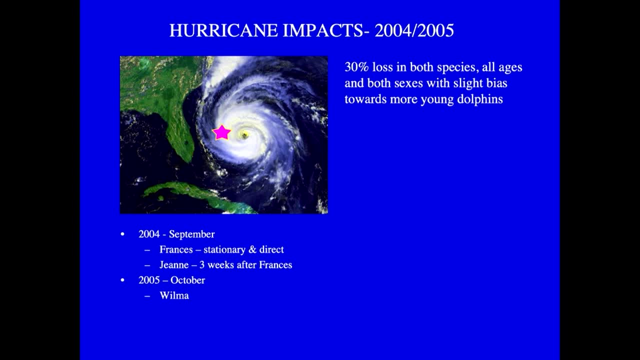 bottlenose and spotted leaned a little heavily towards the young animals, as you might expect, but we had new bottlenose move in to replace the ones. I guess that died or maybe they moved the. what was really striking to me was it totally destabilized the behavior of the spotted dolphins. you know, we knew their behavior. 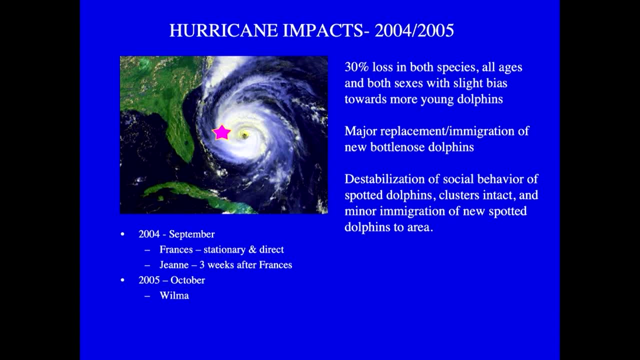 really well and who they hung up with and they just, they just weren't acting normal. they, their groups, were really discombobulated and we had some new spotted show up in the area. maybe they were from some other place that we didn't study, but it took them years and years and years. 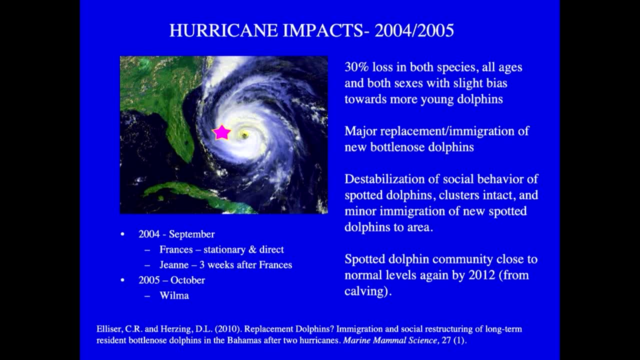 to restabilize and because they started calving again, of course, they started reaching their normal levels, which is about a hundred. you know their population is small, about a hundred animals by 2012. they were kind of getting there back to normal, acting normal, back to their numbers. so that was. 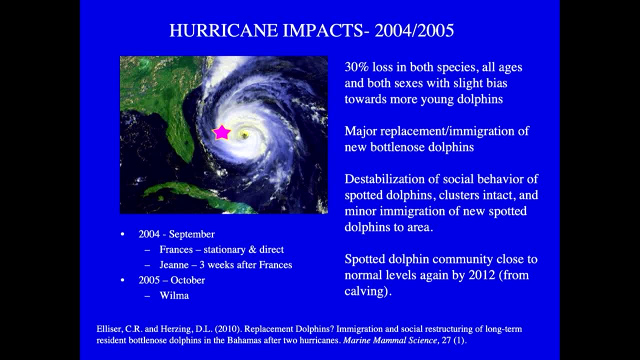 that was encouraging. but it was shocking actually to me that how hard hit they were. but if you can imagine surviving a hurricane for 36 hours, you know you're a young animal, you have to be able to breathe and you know, go back into the water and there's, you know, water in the air the whole time. so 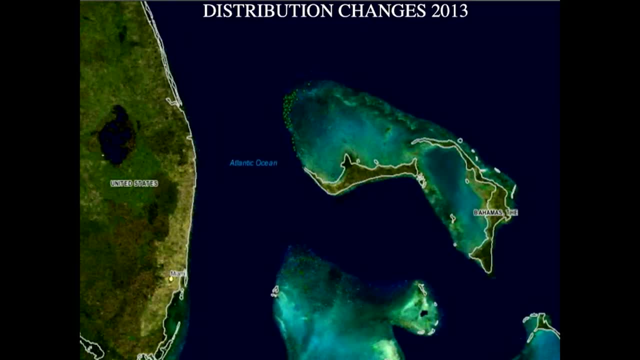 anyway predators around. I imagine that's challenging. then another thing happened. so in 2013 we went out there and you know we had always measured our groups as three clusters, so we had a southern cluster and northern cluster and a central cluster and they were pretty distinct behaviorally and genetically. 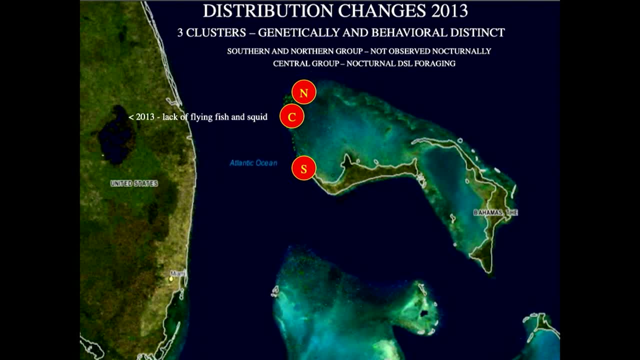 and in 2013 we went out there and the central group was completely gone and after some frantic looking, we finally found them down in Bimini on Great Bahama Bank, crossing about about a hundred miles difference, crossing this deep water which we didn't know they really did. they're dolphins. 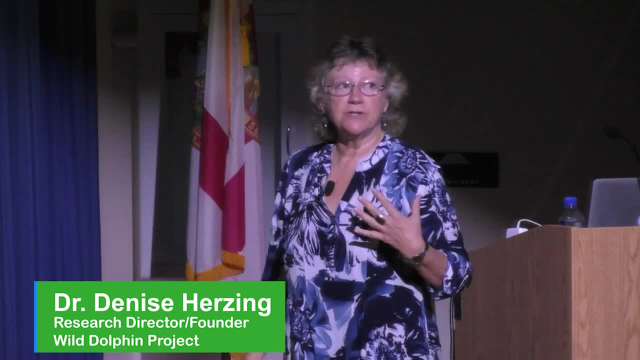 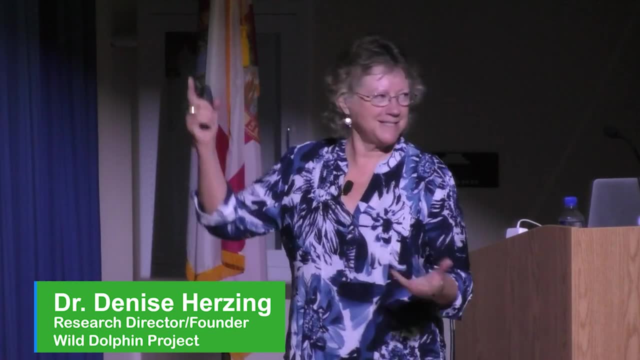 but still we never saw them do it before and you know it was really interesting. we had kind of anecdotally noticed that gosh, the fishermen aren't fishing off the edge of the sandbank anymore and and we stopped seeing sorry flying fish and squid. it was like where's all the prey? 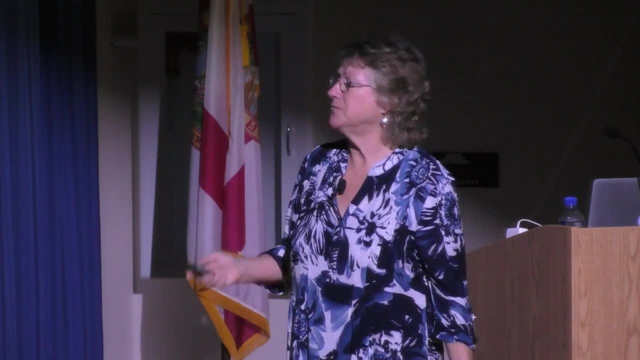 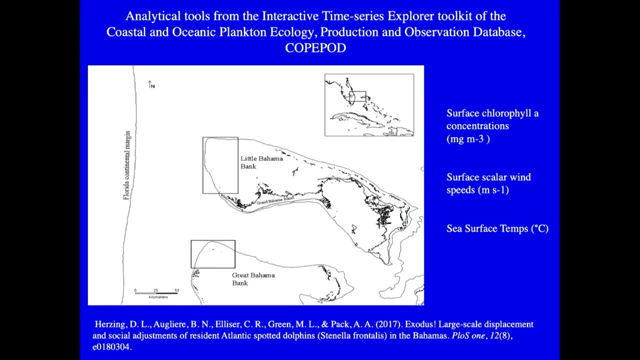 and so I guess the dolphins just they just had to move. so that was kind of a shocker. so we decided, after we kind of eliminated Navy sonar and orcas and you know some of the things you can imagine would scare the dolphins enough to leave. 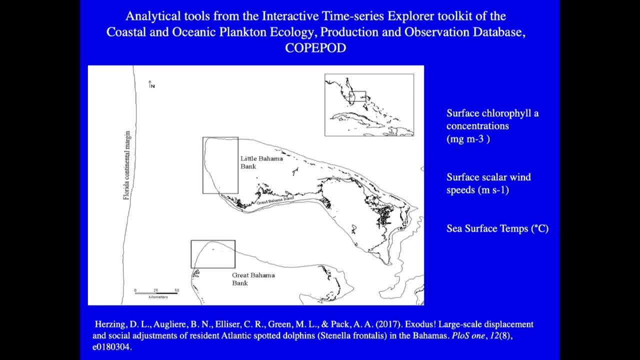 we started looking at oceanographic features, So we tapped into a database called COPAPOD- Coastal and Oceanic Plankton Ecology Production and Observation Database- Phew, COPAPOD, And so NOAA database that was available to us, And so we decided to look at both Little Bahama Bank and Great Bahama Bank and see what we could see in their database, to see if there's any changes. 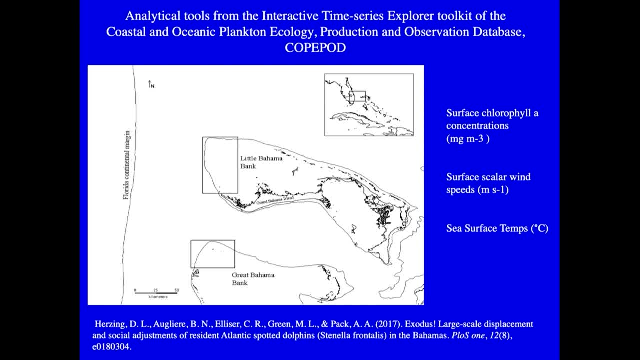 And this is based on satellite imagery right. This is not, you know, hands-on in the Bahamas measurements, Everything is taken from satellite imagery and as a proxy. So we wanted to look at surface chlorophyll, which is a measure of a proxy for plankton right. 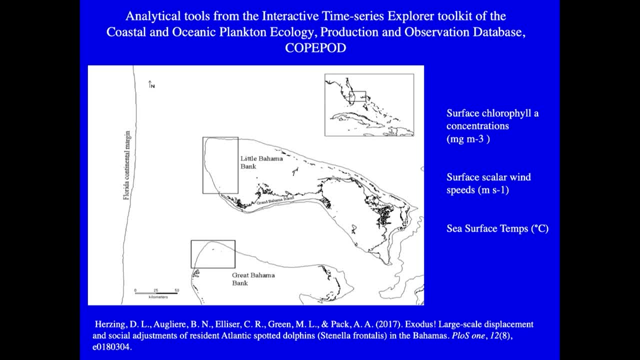 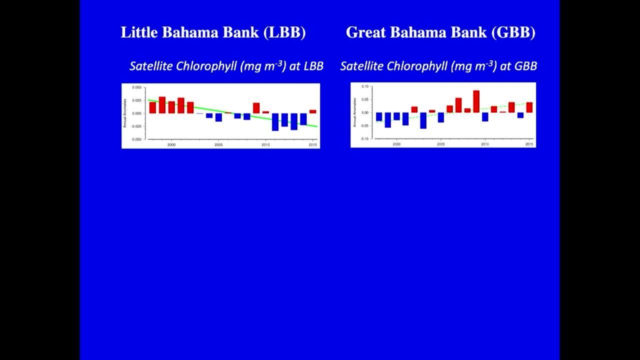 The food chain. We wanted to look at the wind speeds and the sea surface temperatures in both those spots. So when we took a look, we saw the satellite. chlorophyll had a significant drop At Little Bahama Bank. so you see, on the left side, the blue. it's actually a measure of anomalies over the years. 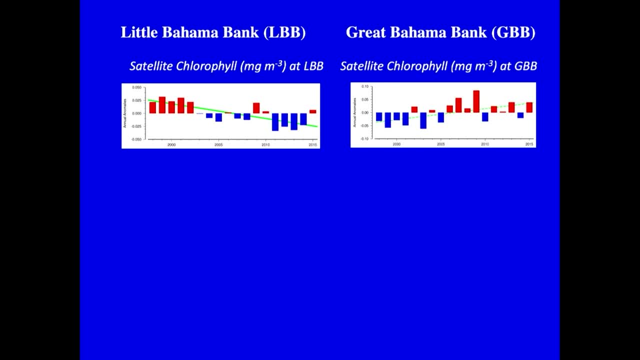 So that's a yearly, that's from 1998 through 2015 is the measurement. So there was a significant drop in chlorophyll on Little Bahama Bank but not on Great Bahama Bank. There were some, but not significant. 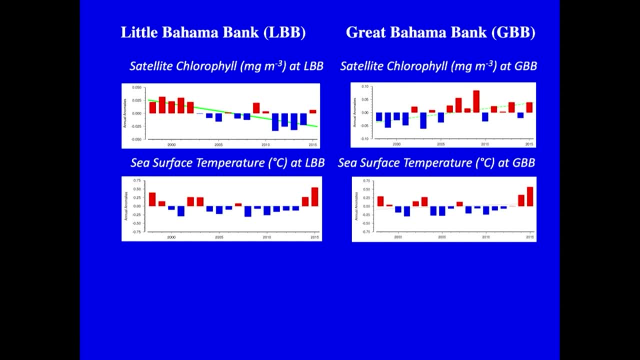 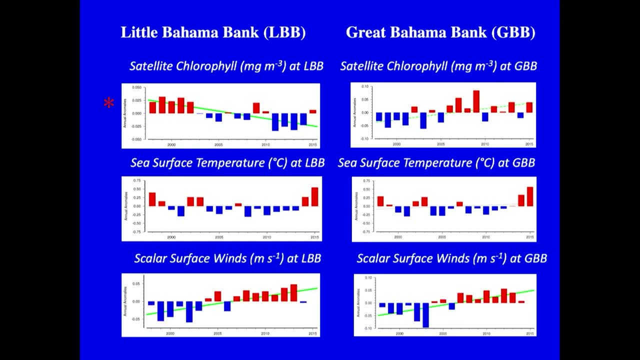 The sea surface temperature. there were fluctuations again, but nothing actually significant. The winds were quite significant in both places, So the wind speeds just were off the scale in both locations. And you know, again we kind of noticed this. You know we're out there all summer. 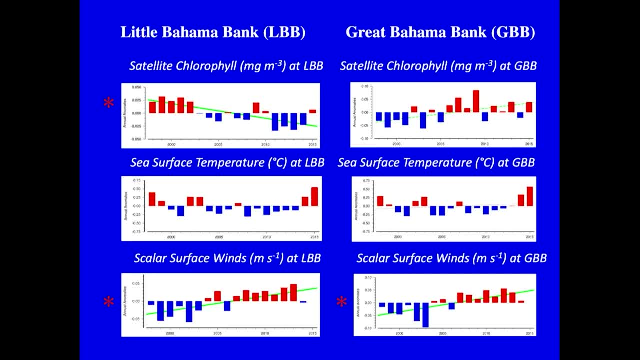 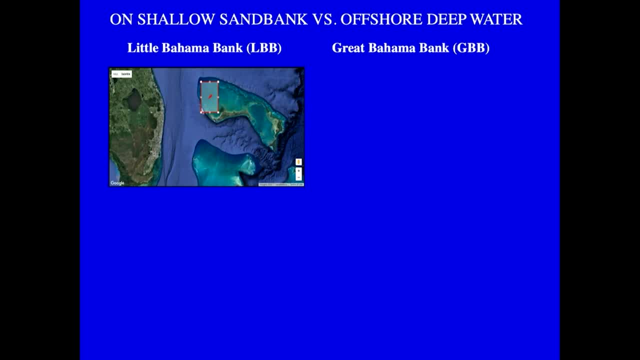 It was like it's always windy. Why is it always windy? So then we thought, okay, well, maybe we should look at the shallow sandbank versus the deep water, right, Because they're kind of two different ecologies, I guess ecosystems. 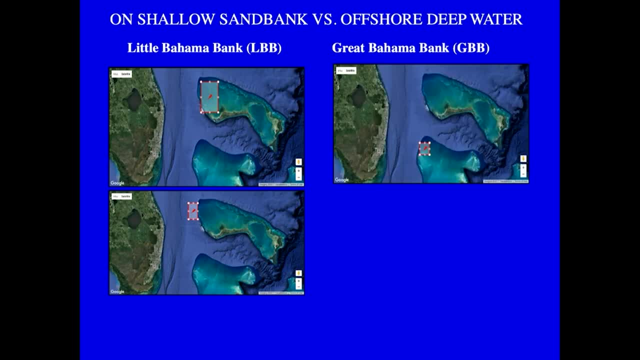 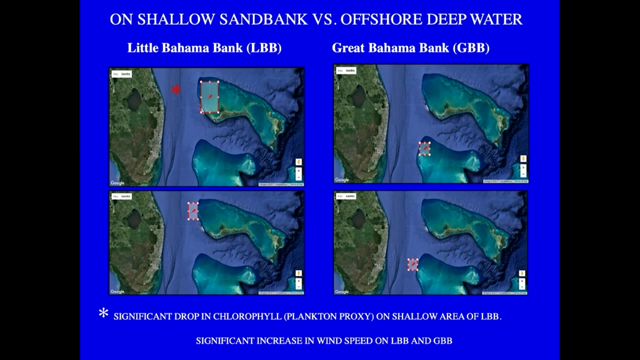 And we thought it'd be pretty interesting to look at. So we blocked off areas on the sandbank- Little Bahama Bank, offshore and shallow, Same on Great Bahama Bank. We did sandbank and offshore And what we found is the only place where the chlorophyll was really significant on Little Bahama Bank was on the shallow, on the shallow sandbank. 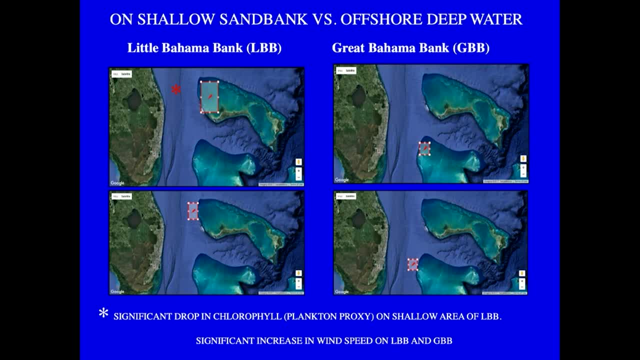 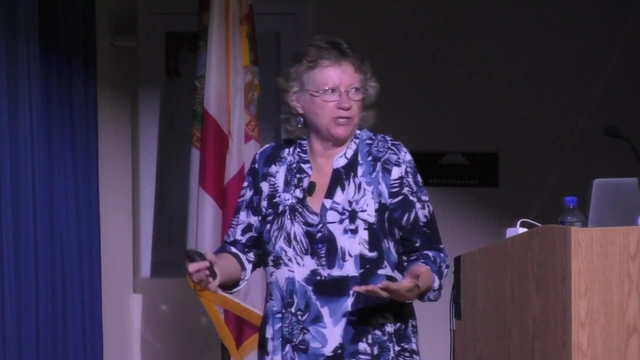 So this suggests a food crash. Now, what was also really interesting is, Because the wind speeds had increased in both locations significantly over you know a decade. we thought, wow, how would that affect? you know production, you know plankton production. 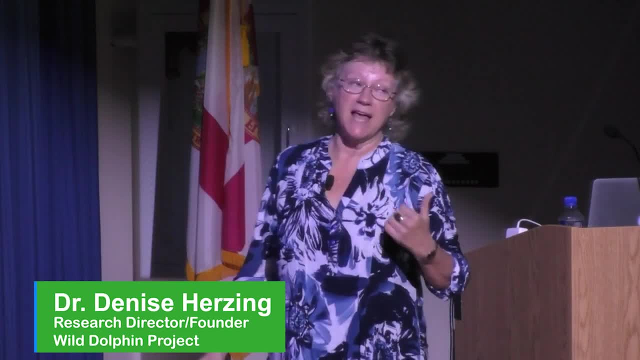 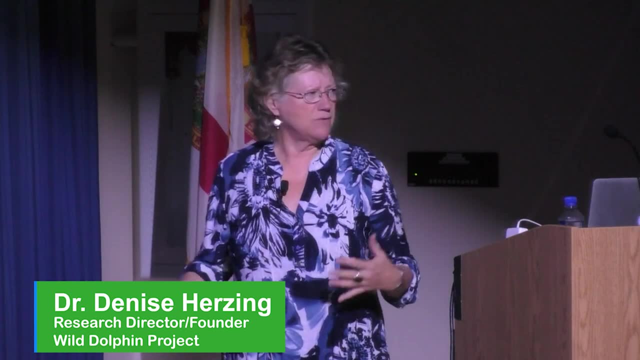 We don't know for sure, But what we did notice- and this was actually not in the NOAA database- we actually collected wind direction when we're out there And we had seen. I don't know if you all remember- some of you probably live here in the summer. 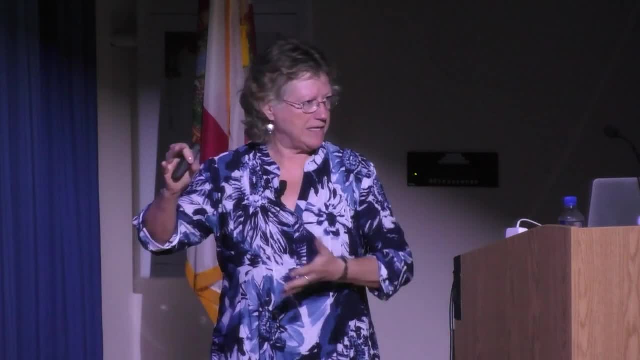 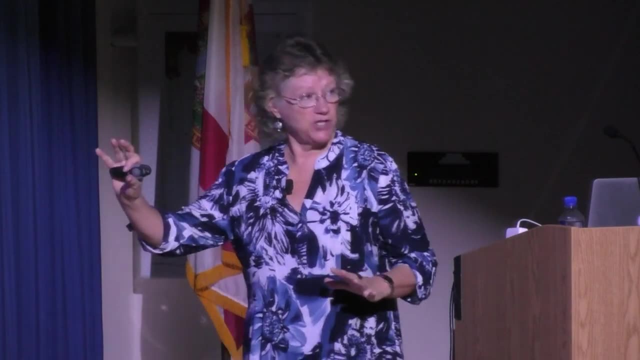 We've had wind coming from the west And we've had wind coming from the west and southwest in the summer a lot, instead of southeast, which is the direction, So you can imagine. so on the sandbank there's a tidal flow right. 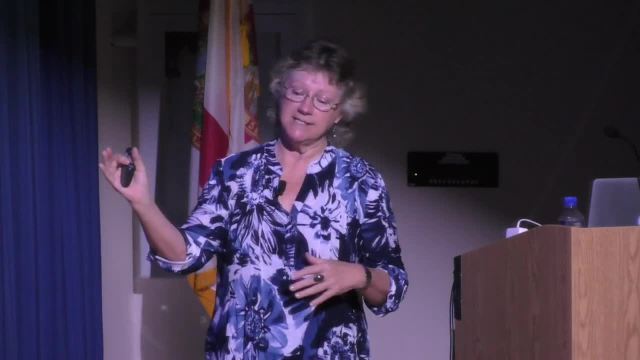 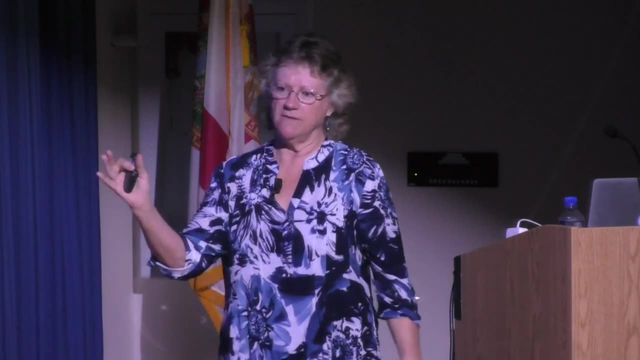 Six hours on, six hours off, And you can. when you're out there, you can actually see on this beautiful- you know- blue sandbank. you can see the murky but productive water coming off the sandbank from the grass beds, and all that. 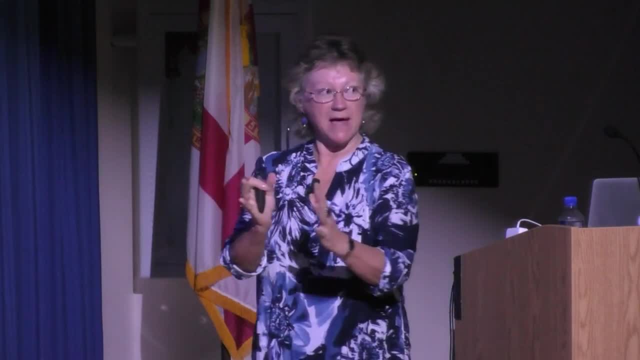 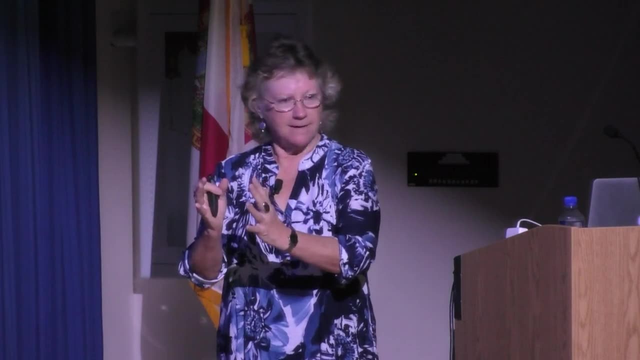 You can see the line And then it goes offshore And then it comes back with the beautiful gulf water right, And so when it was windy you could see that, But the wind actually stopped that murkier water from getting offshore. 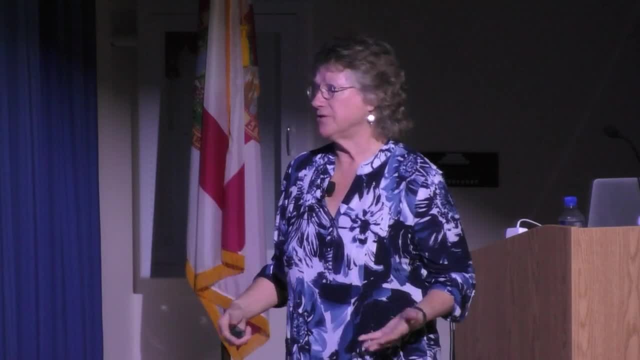 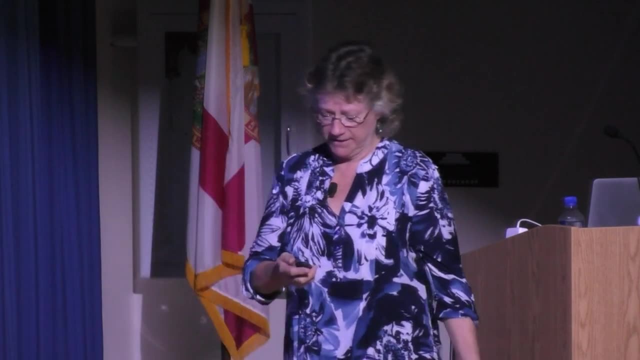 And so we suspect maybe that was part of the issue and the food crashed because the nutrients weren't getting offshore, They were stopping. We're not sure And I've talked to a lot of population ecologists and nobody's quite sure what to make of it. 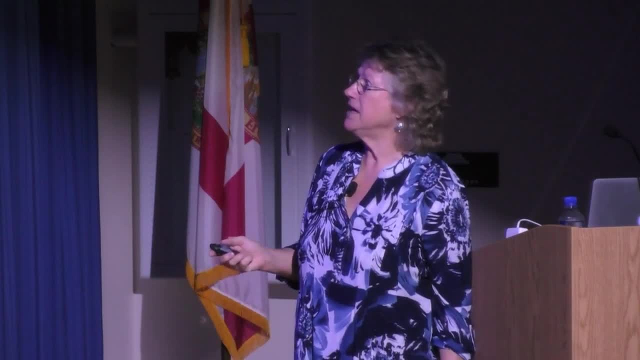 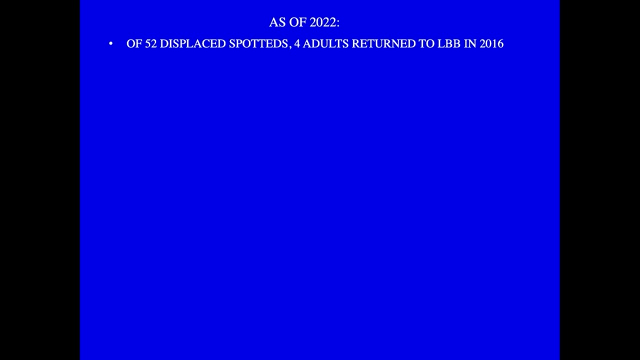 But it was pretty clear that the food chain crashed. Anybody has any ideas? please talk to me. So, as of last year, 2022, the 52 displaced spotted from the central group that moved, we did have four individuals come back to where they were resident and they've stayed. 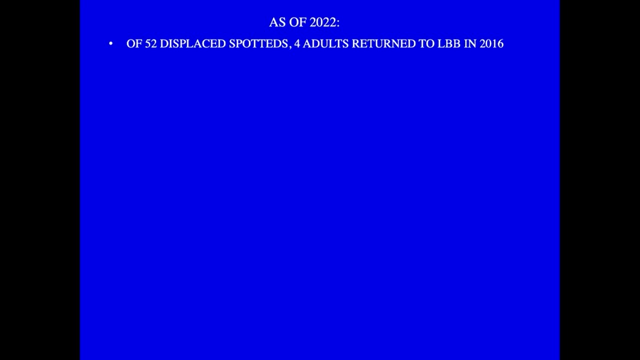 And we didn't actually know. at first. we were like, could they just be lost? I don't know. Could they be lost? Did the hurricane blow them somewhere and they don't know where they are? But four of them came back. 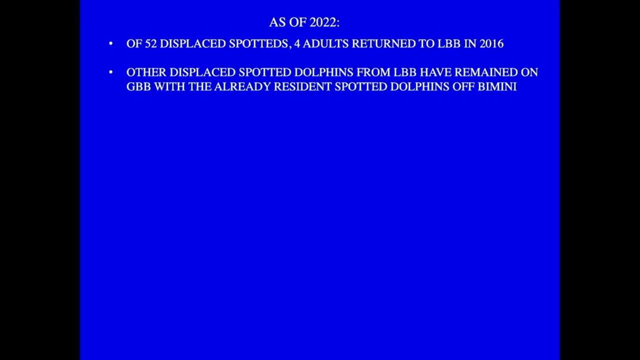 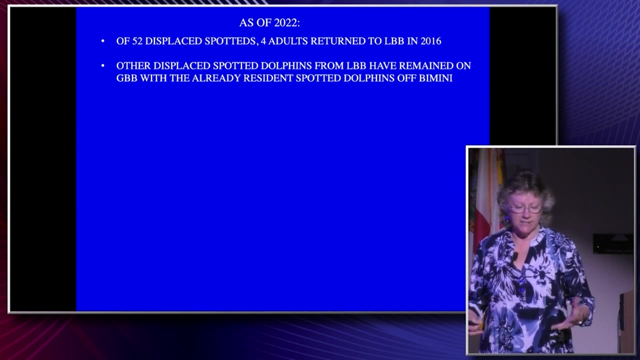 So we think, okay, they probably knew where they were and found their way back home. All the other dolphins that moved from Little Bahama Bank, they've stayed on Great Bahama Bank Around Bimini And they are now trying to interact and associate with the already resident group of spotted there. 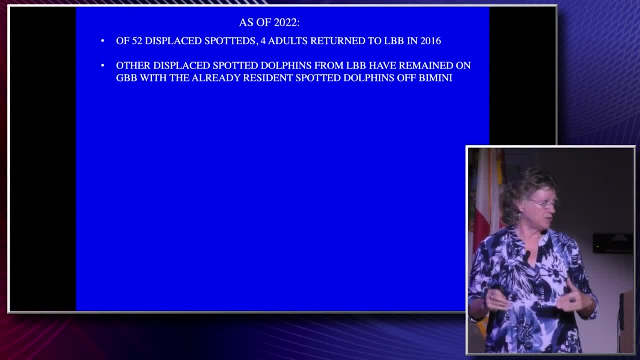 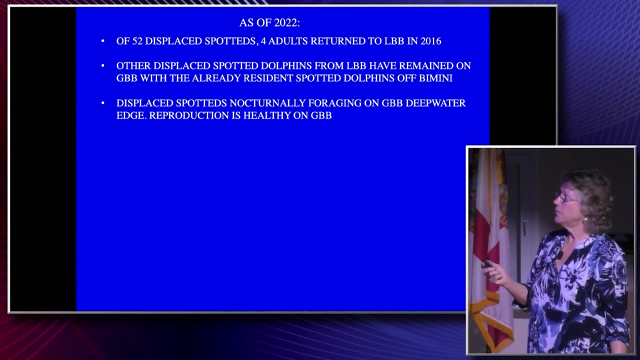 So when these displaced dolphins moved, they moved into someone else's territory, right? So this is what's also happening around the world, with climate change and raising sea levels, as animals that usually don't interact are starting to interact, So they moved into someone else's territory already. 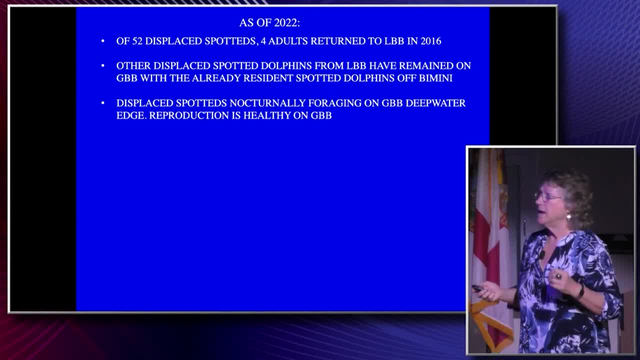 Um, the spot, the spotted that moved from Little Bahama Bank. they are now feeding off that deep water edge nocturnally. So that's kind of the pattern they had in their previous home. So at least they've been able to do that. 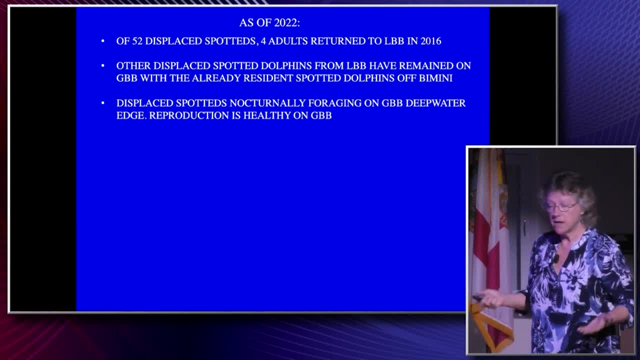 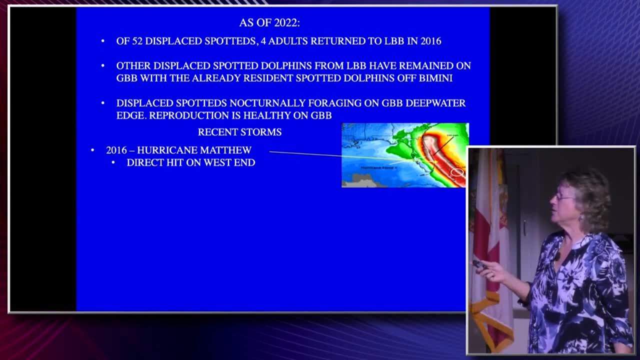 And their reproduction looks pretty healthy. Actually, they're calving well, which is great, Um, but then we had some recent storms, 2016,. we had Hurricane Matthew, which was a direct hit on West End. It was actually supposed to hit us and right at the last minute it veered in the Gulf Stream and hit West End. 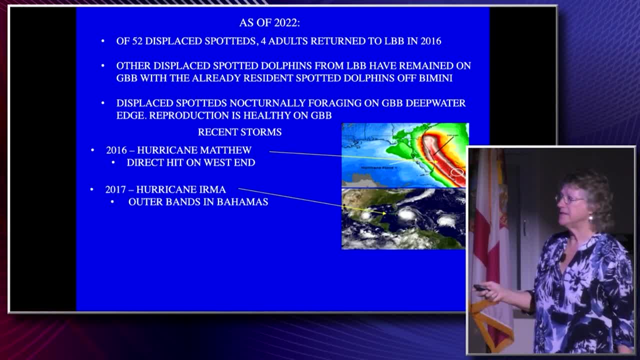 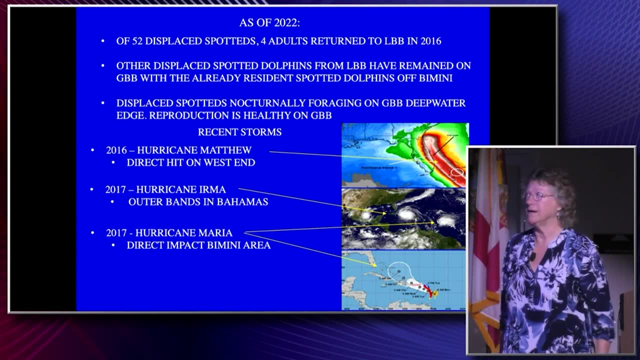 And that was a big hit. And then in 2017, we had Hurricane Irma. That was a really bad year- And Maria, those also went through the Bahamas, So it was like, oh, come on, like, give my dolphins a break, you know. 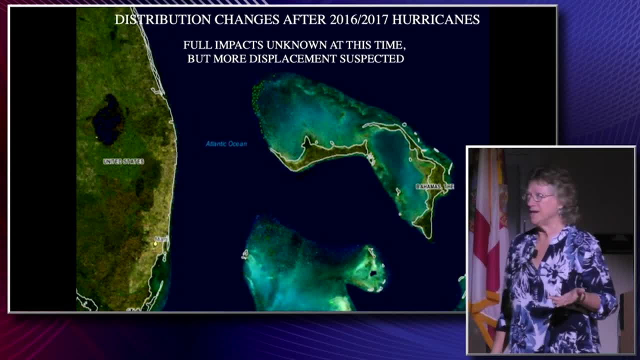 Ah. so we don't really know what the big impact of that was. We're still kind of monitoring and checking it out. We have seen um more of our animals from Little Bahama Bank up north move to the south. So you see the central group now. 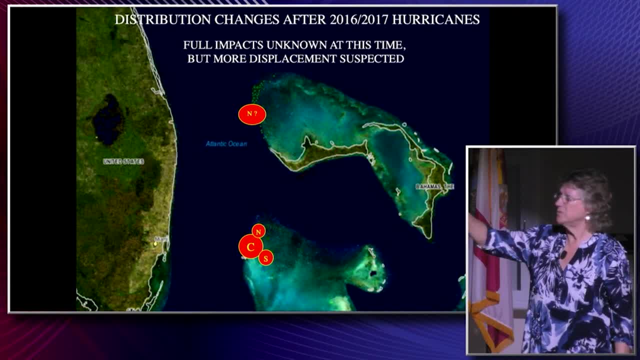 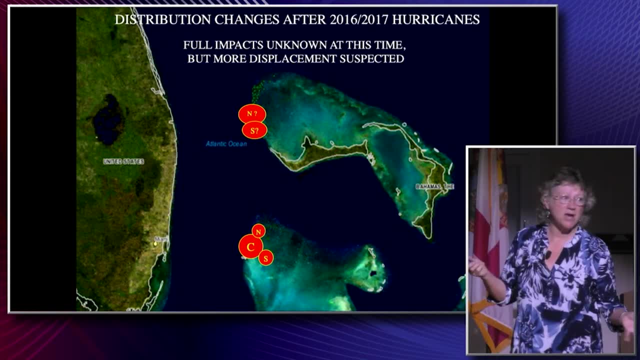 And now you see some. We have northern animals and southern animals that have also moved. Um, we don't know totally what's going on. uh, Little Bahama Bank. There are some remnant spotted dolphins up there, but not many. 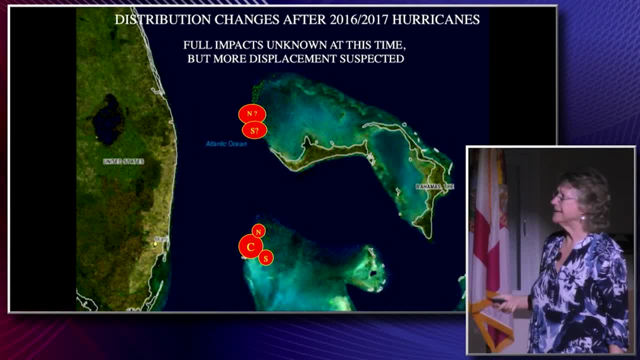 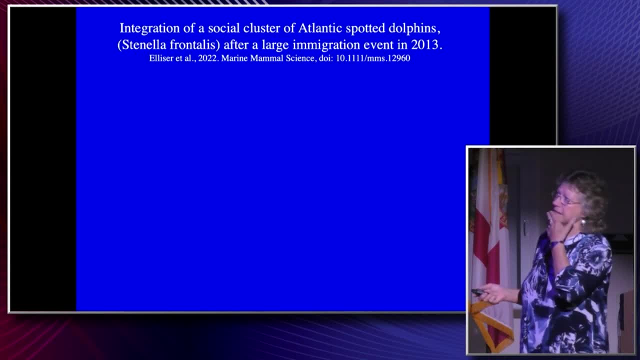 And not many bottlenose either, So it's a bit of a wasteland. Um, there's some, but not a lot. So, uh, recently we did a paper on how the displaced dolphins were integrating with the resident Bimini dolphins. 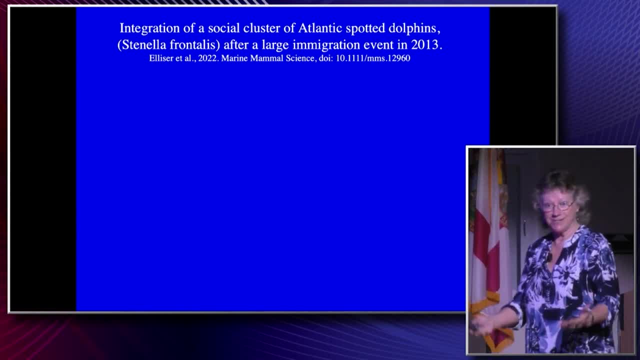 It's pretty interesting. So, like what happened When you move into someone else's territory, is there enough food? Do you mate with each other? You know what? what goes on? Um, so it's a lot of data analysis. 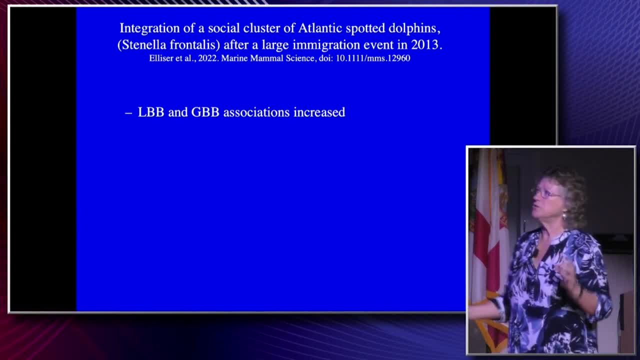 And basically, uh, what we found is that the two groups basically started associating more, as you would suspect- I guess they have to to a certain extent. Um, they still did prefer their own groups, so they kind of stayed with their groups, even while they were interacting, uh, with the local, local dolphins. 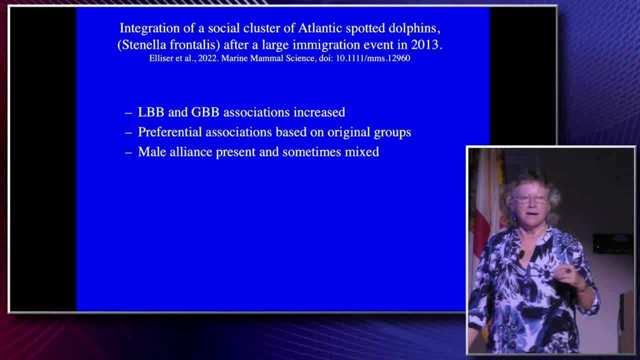 Um, the male alliances were still present, Um, but we had some um defections. So we had a couple, a couple of the- how shall I say this- The very bold males of our group moving into male alliances with the, uh, the new guys. 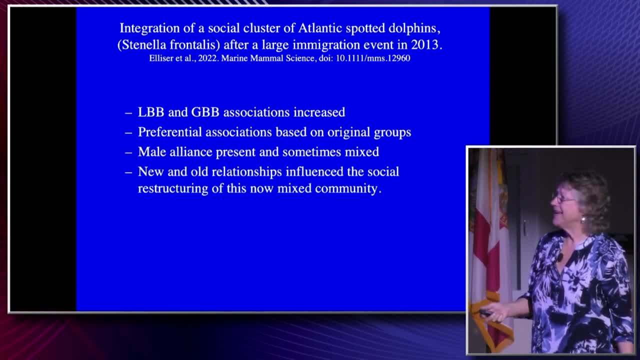 So that was pretty interesting. So so that shifted, But still their new and old relations were heavily, uh, influenced by the whole restructuring. So basically, you know it's a big mixture. They're getting along, They're calving. 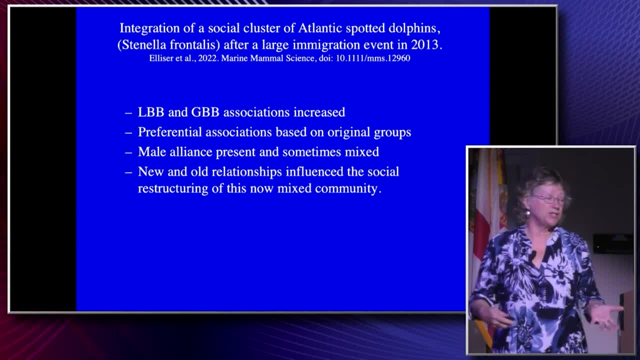 But it's still, you know, it's still a mixture And we're still trying to do genetics to find out, really, who's siring the offspring. So, is it males from the resident group? Uh, are the immigrants, you know, still siring offspring? 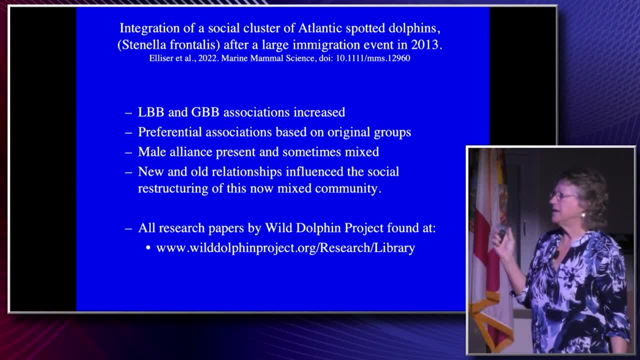 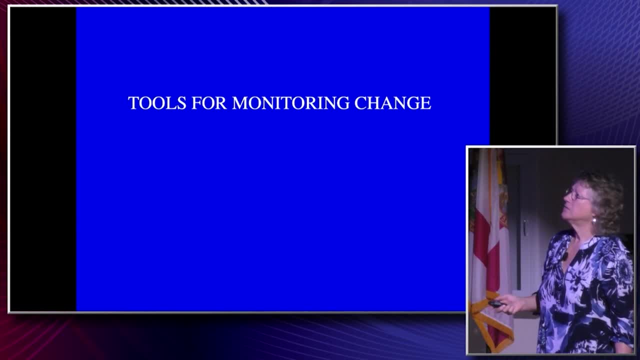 We don't know. And if you're interested in any of our research papers, uh, they can be found on our website, uh, under the research and library. Now some of the tools. I just want to talk briefly about some of the tools that researchers are using all over the world. 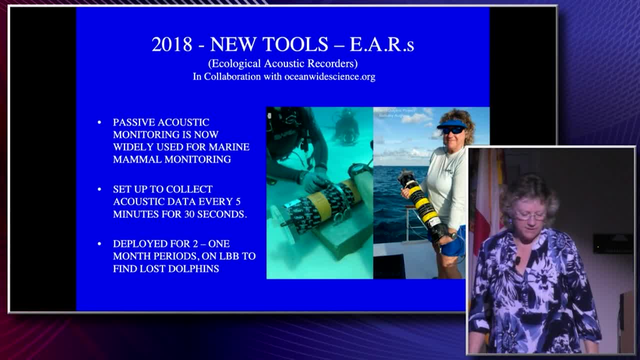 To monitor change. Uh, the first tool is uh really a passive acoustic tool. So these are various uh units of sound collecting units that uh researchers use, And they're uh basically passive acoustic monitoring devices. They sit on the bottom of the ocean or they're uh, you know um mounted on the bottom of the ocean. 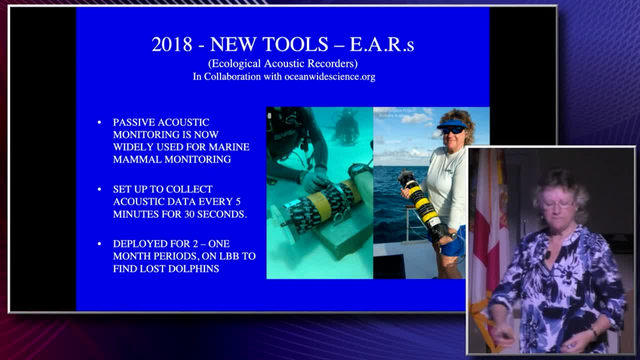 And they collect data while you're not there, So you can set them out, Leave them going for uh months actually, And some even go a year. Uh. so in 2018, we actually did this- We set up uh a device called the Ear Ecological Acoustic Recorder. 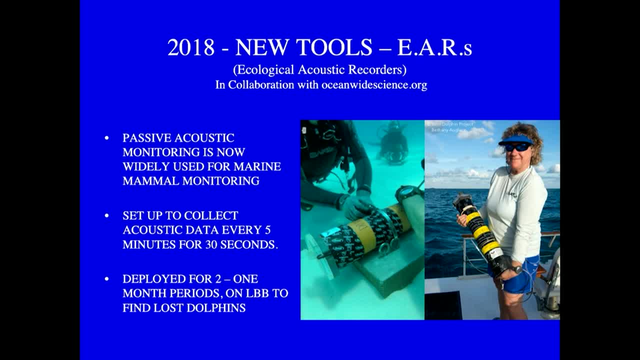 And it was basically a lot of battery, a hard drive, a hydrophone that would record sound, And it was uh, set up to record sound, uh, every five minutes for 30 seconds, And so we deployed them. Then one month later we'd pick them up, swap out hard drives, put it back, et cetera, et cetera. 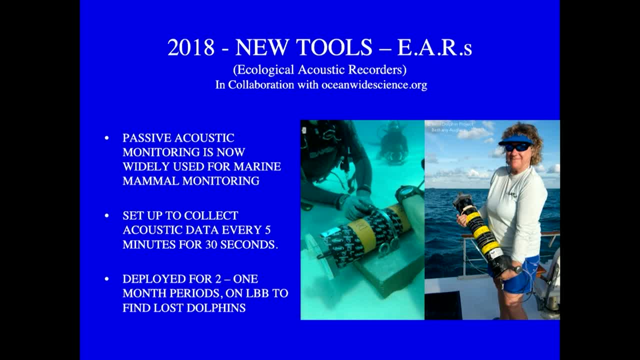 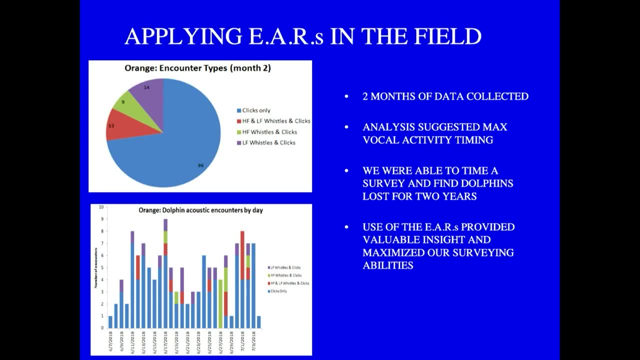 And so what was really cool, though, Is we were able to um find some of our lost dolphins from the data, So it basically the data would give us uh clicks, high frequency clicks- Uh, high frequency whistles- low frequency whistles. 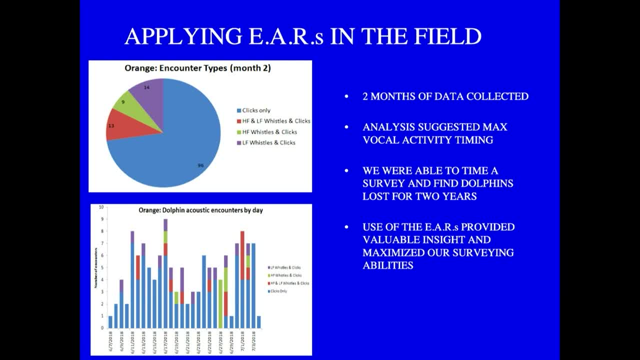 And that was basically species specific, And so what we did. So on the bottom left is actually just a graph by date. So this, uh, it was data from June, June 2018.. And we were able to look at this graph and go okay. 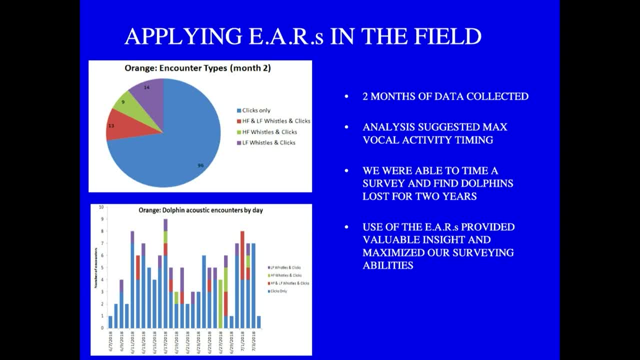 Oh, on June 15th and, and they were here whistling away. so we looked at the tidal cycle and said, okay, let's try to get out there during the same tidal cycle the next month to see if that is maybe when they came by. and, sure enough, we went out. 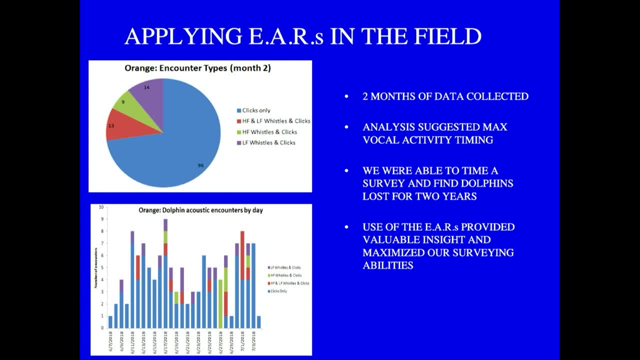 there and there were some of our dolphins, and because there were so few dolphins left, we really wanted to find the ones that you know we were looking for. so it was really a valuable tool to show us the activity of who went by when, and researchers really use this all over the world they can look at species. 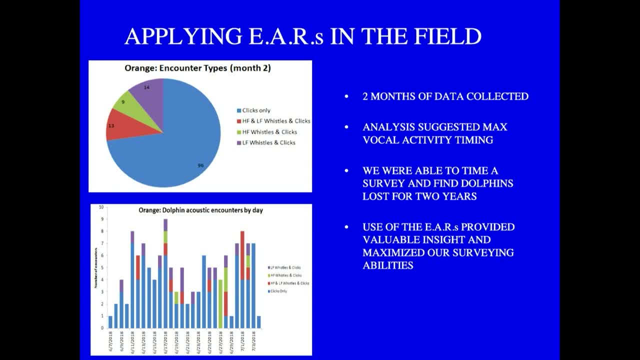 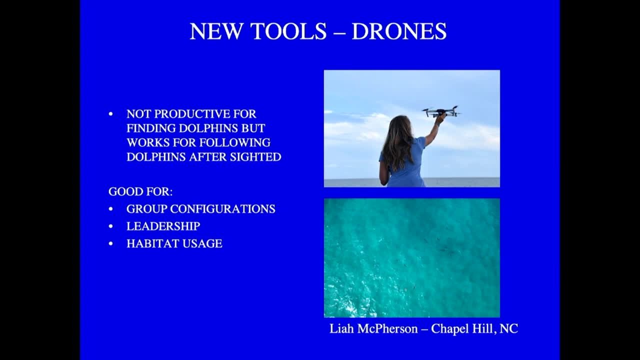 you know when species go by the activity, that sort of thing. now drones, of course, everybody's using drones. this is a great view that we haven't had on marine mammals did. a lot of you probably saw the right whale video, the from the drones, the aerial video. that was fantastic, right, so it's a fantastic tool to just. 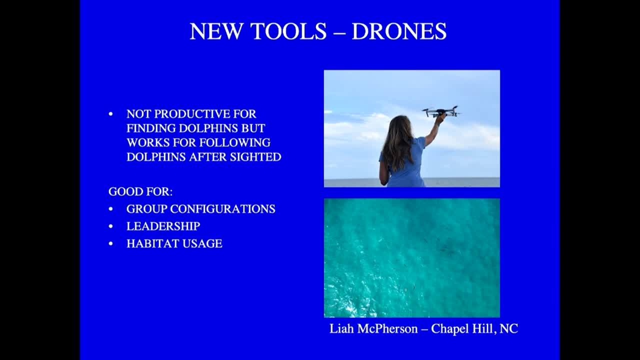 see animals. in our case, we found because we were on our research boat. we found it wasn't so productive to find dolphins just by looking, because you know the drones still have limited battery life and and you can't fly them dirt during certain wind speeds, so they have some. 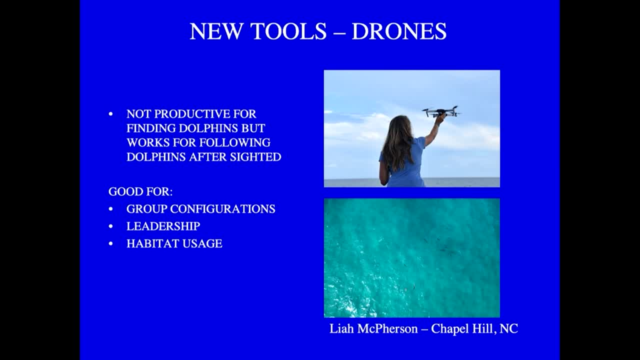 limitations, but if you see dolphins, you put up the drone, you can follow them. you can look at their group configuration in the water. you can look who's leading the pack, for example. you can look at what habitat use they go over. so there's a lot, a lot of uses for for drones, and so that's the work that we're doing, and so 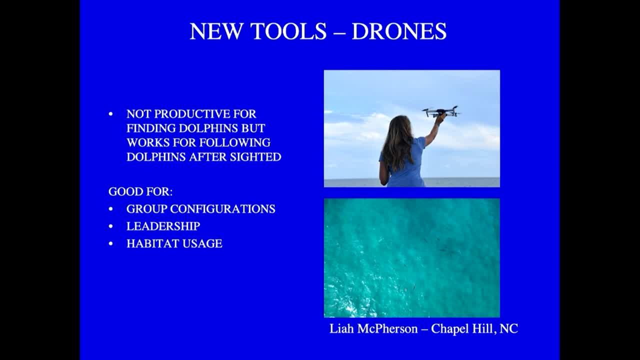 One of the main tools actually is looking at the health of animals. now they can take a drone and they can look at whether an animal is pregnant, Emaciated, that sort of thing, so they're being used all over the world for large whales as well as dolphins. 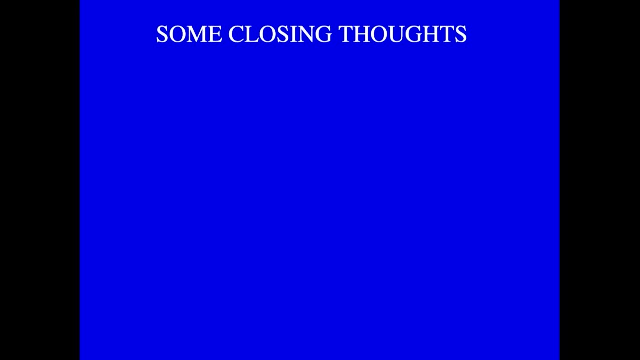 Just some closing thoughts and then I guess we can have some question and answer. so There's a lot of impacts that are going on with ocean animals because of these environmental changes and climate changes. I really never expected The dolphins of the Bahamas to have such dramatic Impacts. I really didn't, because they were there, were really considered, You know, fairly safe. 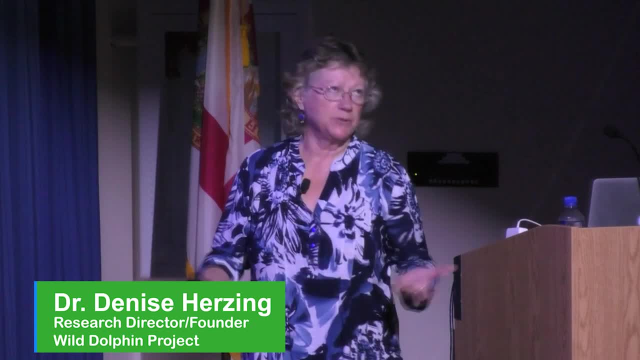 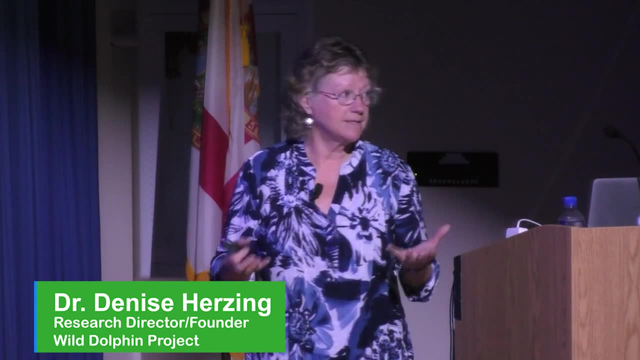 They didn't have a lot of fishing net issues- and I mean there's pollution everywhere- but you know they were relatively healthy population. So we felt like, wow, we have this view of this great, healthy population. That's normal. and then all of a sudden the food crashes right, so things change. so this is happening everywhere and Because dolphins And whales are so mobile, You know they have the ability to adjust their locations, but At what cost? you know, are they going to not be able to integrate with local animals, disturbing their resources? You know this is a big, big question. There's not room for everybody necessarily. 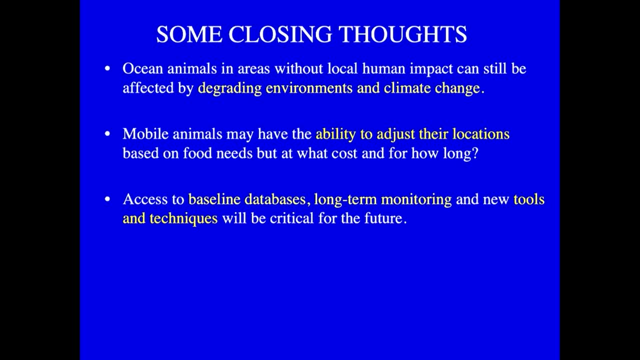 And you know the. the only reason we knew what was happening with this Displaced activity with the dolphins is because we were out there every year and we knew Individuals, we knew their relationship, so we knew where they were, so we could see the changes. and you know, long-term research is. 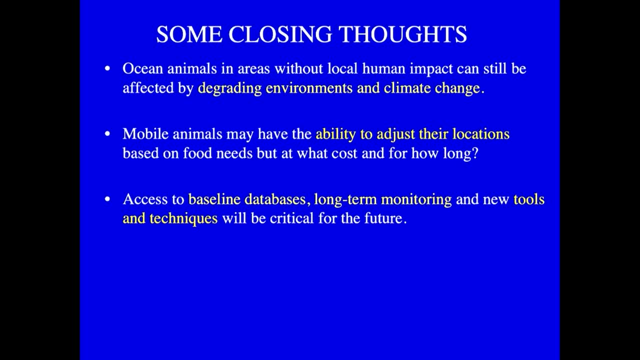 Really, really important, because if you don't have the baseline, you're not going to see the changes, you're never going to notice What's happening. so all these you know projects you hear about, Believe me, they're important- long-term research, whether it's turtles or dolphins or whales, and the tools and techniques they can all be. 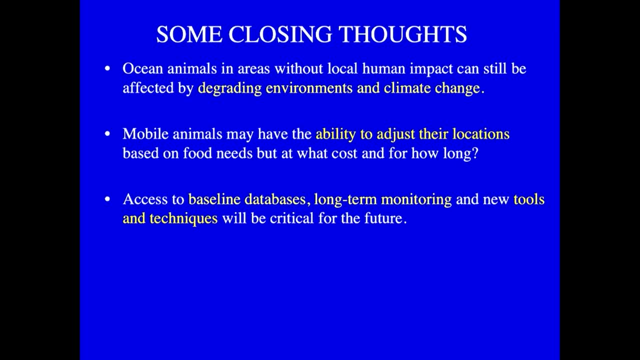 You know, really important and Oh you know this, students now are so smart and so tech savvy. I mean I'm just in awe, like thank God they exist right writing programs. I'm just the old naturalist with my binoculars, but anyway. so think global, act global. I think we have to do it all. 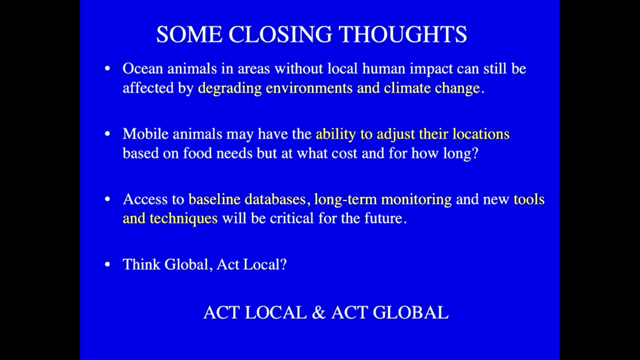 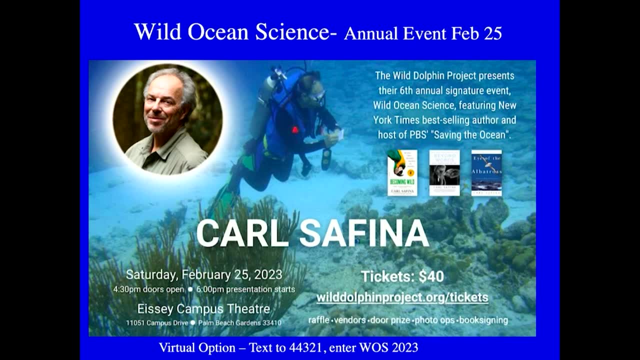 act local and act global, I think, and just some selfless promotion. we are having our annual event called wild ocean science on February 25th. I think there's still information back to pick up there if you want to come by. Carl Safina is a well-known author and naturalist and there's a virtual option. 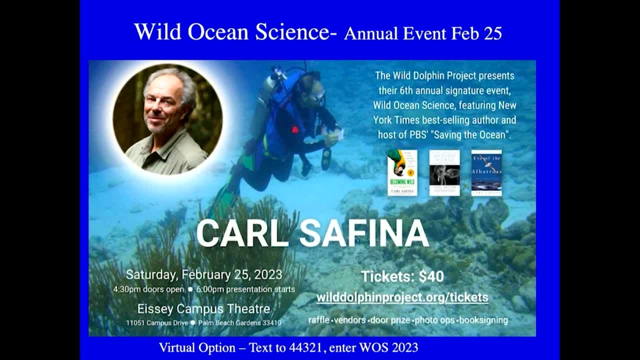 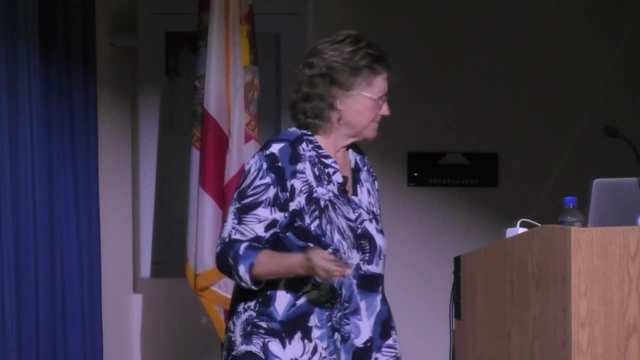 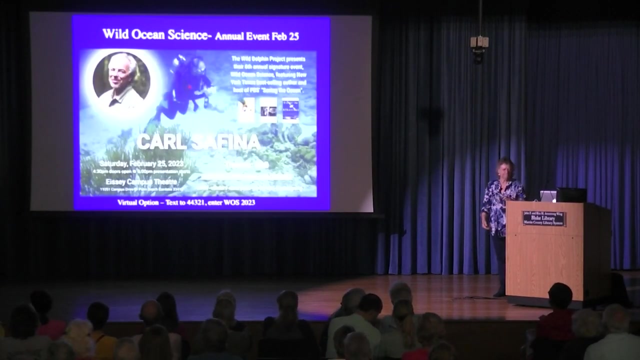 too, if you want to just come on virtually. but we're excited. it's kind of our only once a year, our way of giving to the public and getting a good speaker and sharing that information. so thank you, and I will leave it open for questions. let's see there. 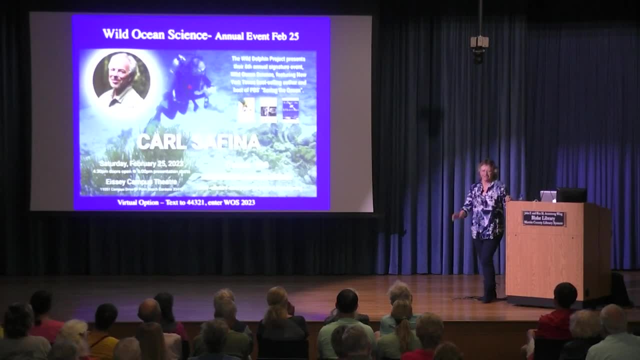 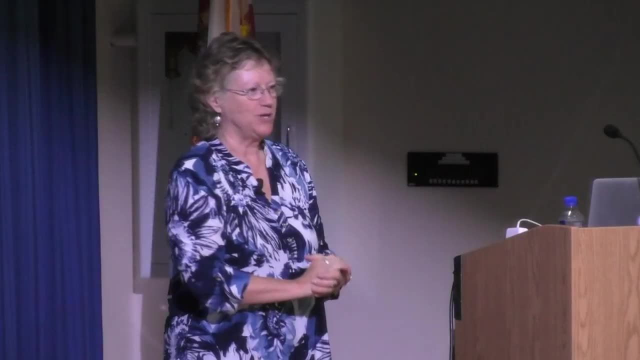 that's the big question. oh sorry, yes. so the question is: how do you think they knew to go to the southern bank? The northern dolphins move to the next sandbank down. how did they know to go there to look for food, right, so interestingly, we had actually done some. 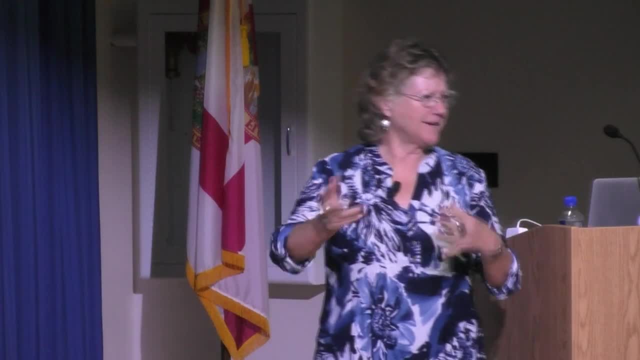 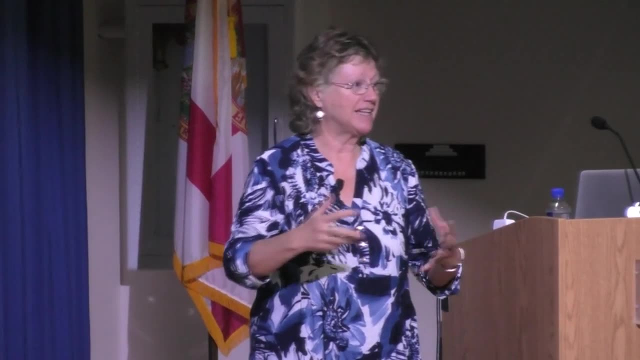 work on the Great Bahama Bank previously, kind of in the winter and kind of odd times, and we had never seen any photographic matches. and there was another research group also down there and we looked at their catalogs so we didn't think they ever went down there. right, you ever saw that. so we were like 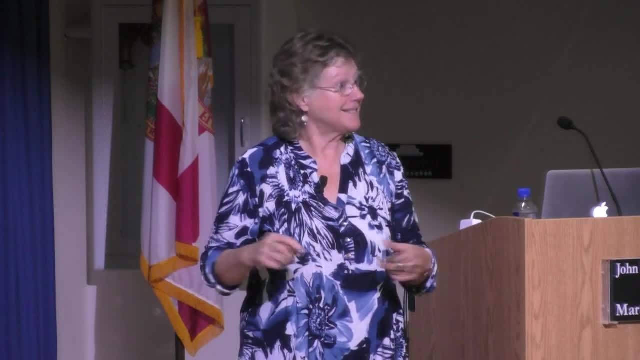 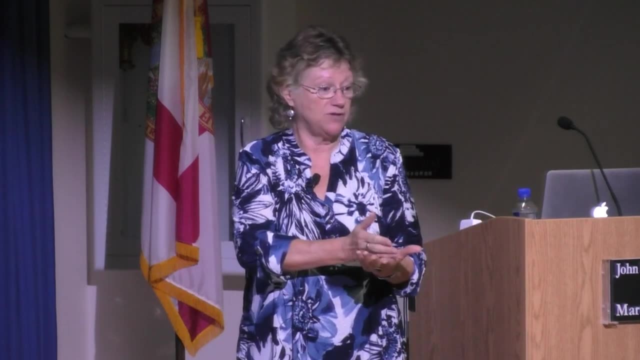 well, I don't know, did they move as a group and just run into it? Did they send a scout? Oh, it's possible. I mean we didn't see when they moved. you know, somewhere between September, when we finish our field season, and the next May. 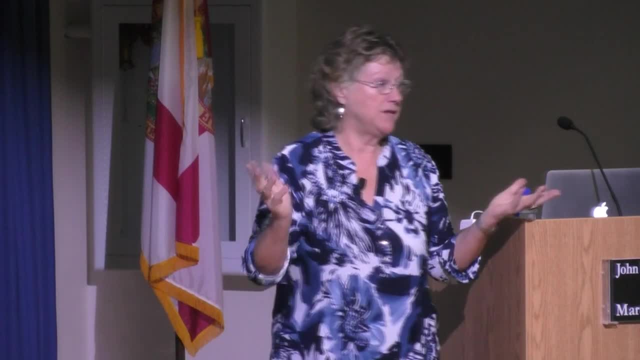 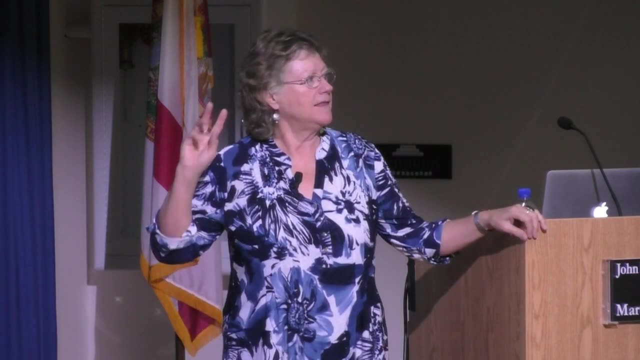 they were gone right so they could have scouted the area. I don't know. I mean, that's a really great question and I wish we knew- yeah, I don't know now- the fact that the other four animals, oh sorry, well, so we actually had a good. 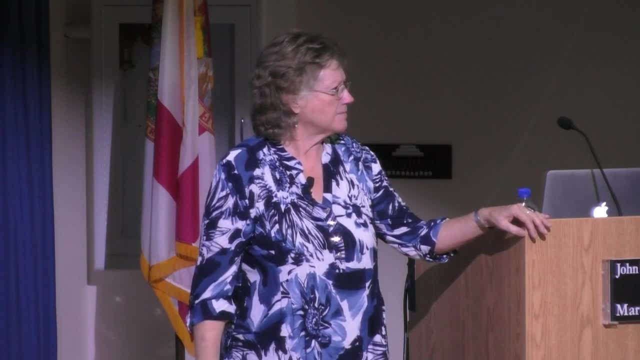 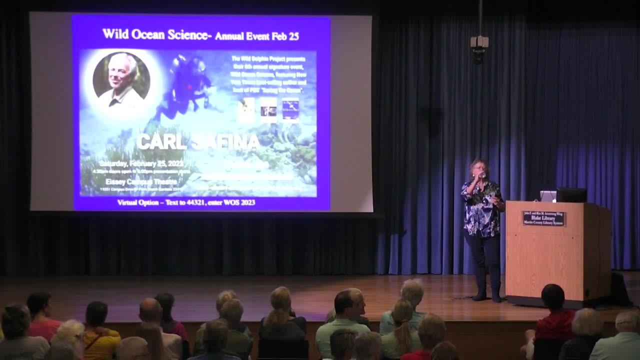 follow-up to that online. somebody mentions that some of the great whales- humpback whales, for example- have songs that can be heard over the course of hundreds of miles. is it possible that they could hear each other from the Little Bahama Bank to the Great Bahama Bank, or is that stretching it for for dolphin communication, I think? 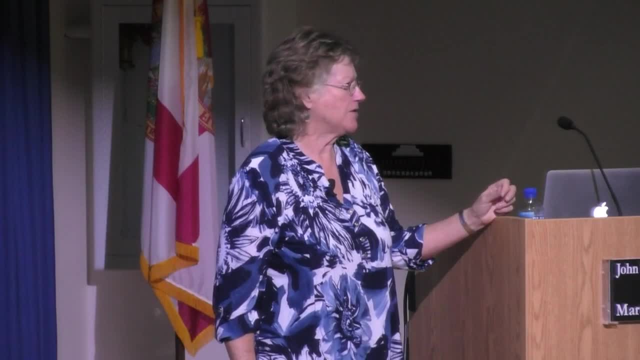 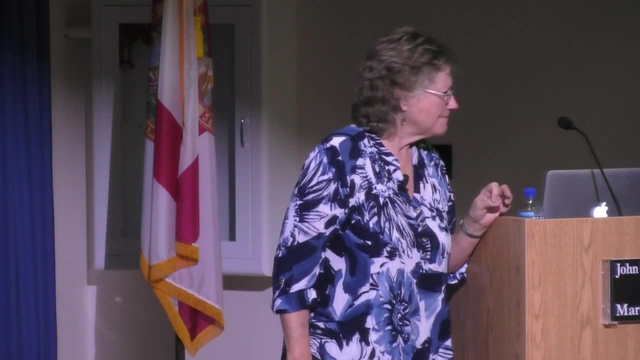 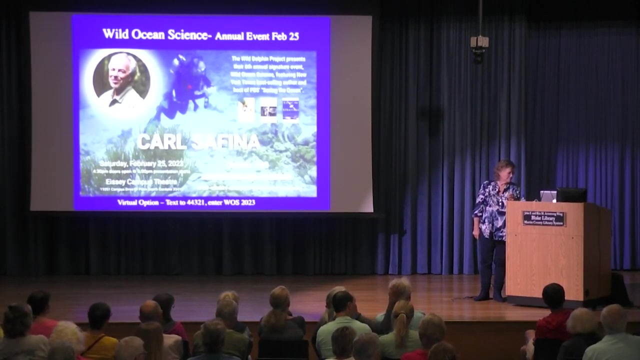 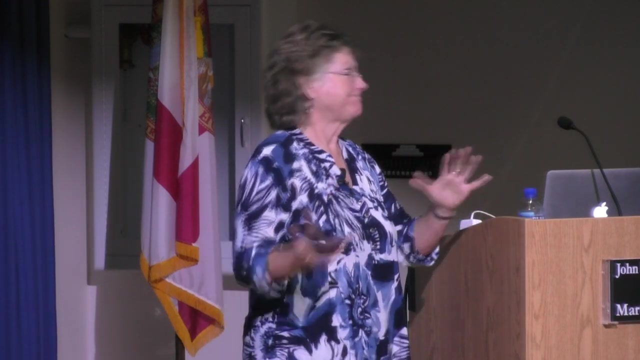 for dolphin communication. that would be stretching it as far as we know. their sounds wouldn't transmit that far, correct? yeah, so the question is about moving the beach sand. you mean off the coast here. yeah, so well, we do study the dolphins off this coast. to. the question was: did? 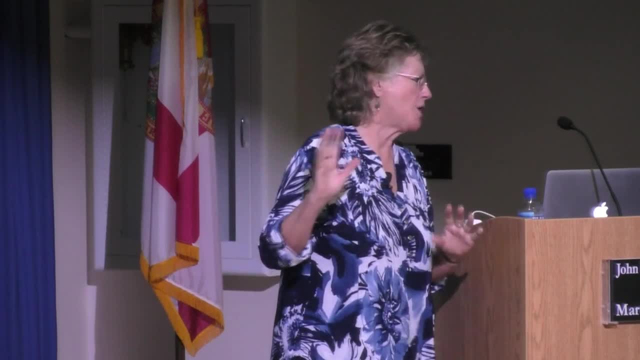 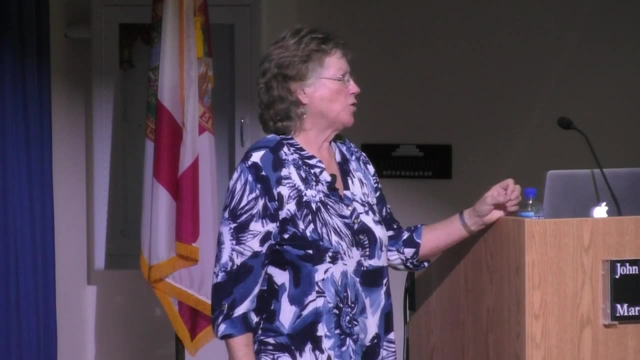 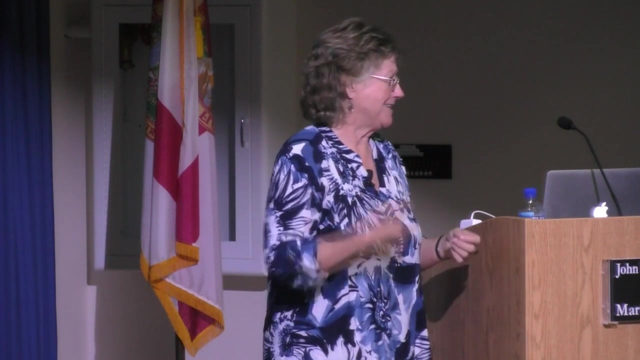 the dolphins leave and come back. yeah, I couldn't answer that. our work is really in the Bahamas, so that's really across the Gulf Stream. yeah, I mean, I imagine for local dolphins off our coast you could easily disturb that substrate, you know, if you're, you know dredging sand and putting on the beach and you know. 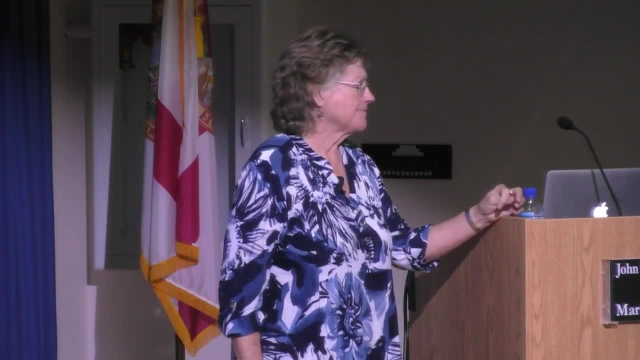 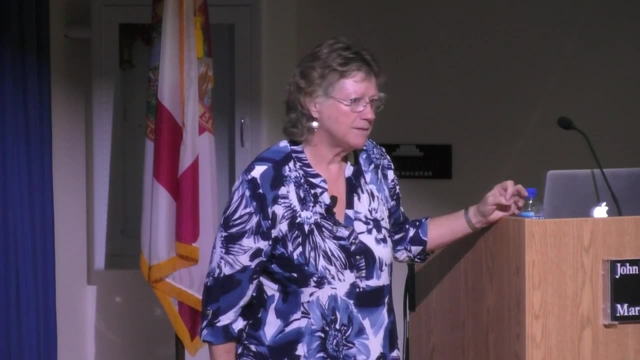 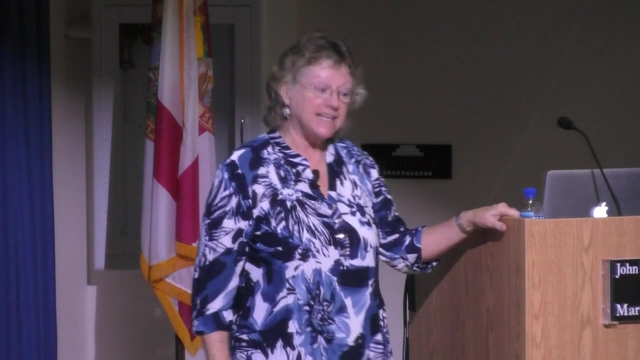 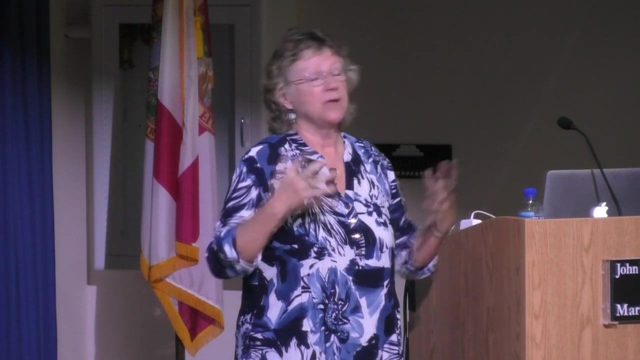 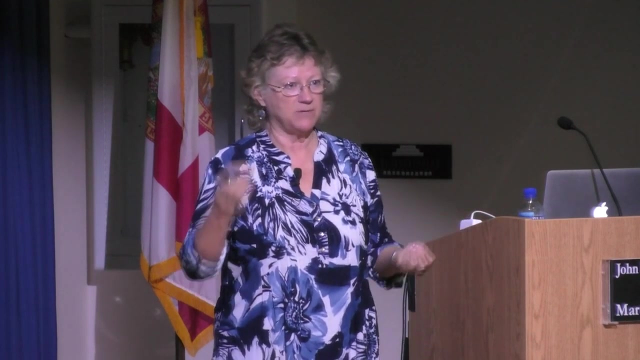 nobody really studies that, as far as I know. dolphins, what can I tell you about dolphins breathing? yes, they breathe, yes, so. so dolphins have one blowhole. you know most whales have two, and they breathe according to their activity. basically, right, I mean, they're really efficient at using air first of all. right, so they'll come up to the surface. 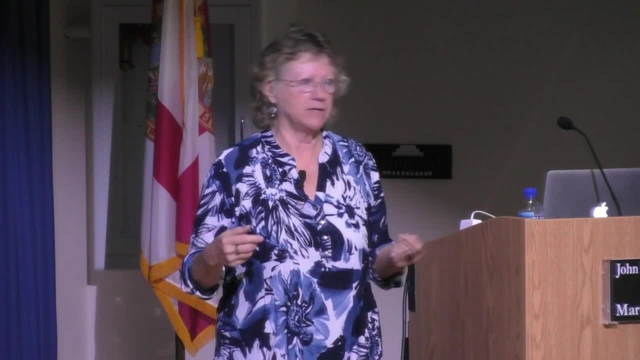 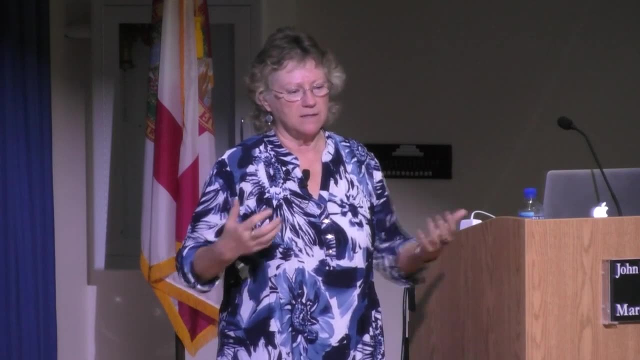 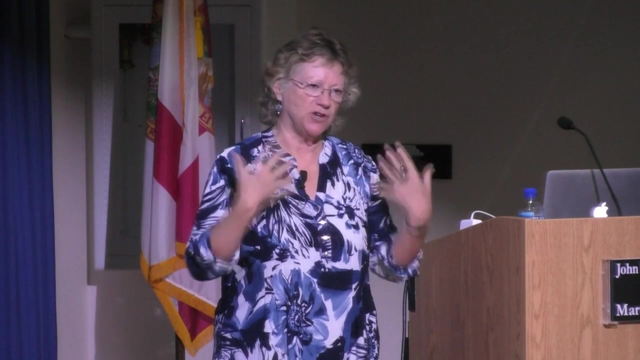 breathe and they can hold their breath for, you know, anywhere to 20 minutes, probably a small dolphin at depth, and they store most of their oxygen in their muscle, their myoglobin versus their hemoglobin, so they can dive deep. yeah, shunt all their, you know, blood and oxygen to the critical organs, but like 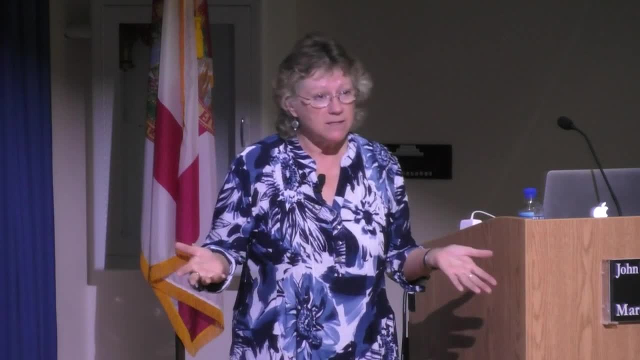 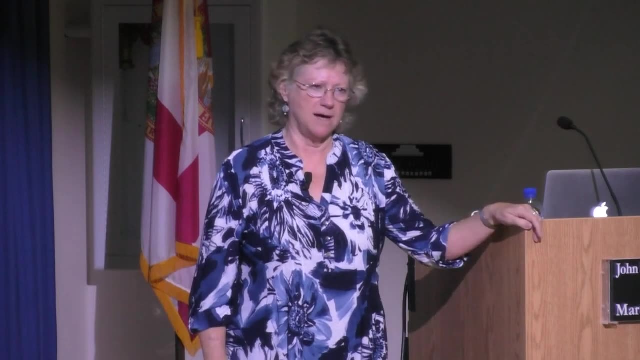 you know, when they're feeding on the bottom they'd probably be down two or three minutes, for example. they could be fighting down there for a minute or two. you know they're not on the bottom a lot, they're at the surface a lot, or in the 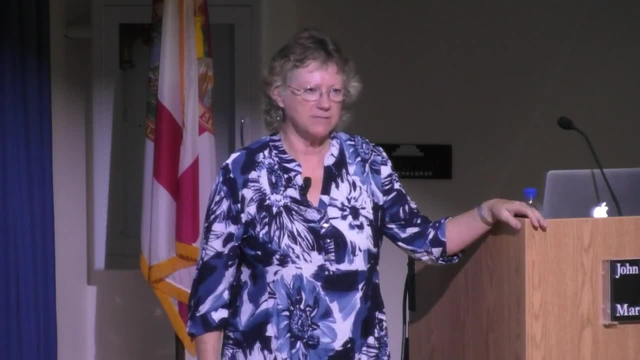 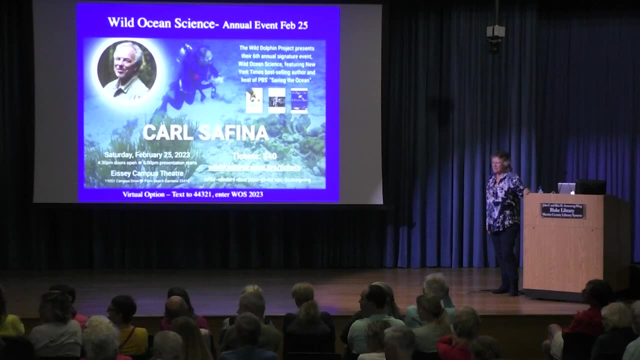 middle of the water column. but it really depends on, I guess, their energy expenditure more than anything. so what do dolphins do when they fight? so you saw some video. so remember they're mammals, right, they play and they, they have fun and they love each other, probably, but they also fight, you know. they fight for food, they fight for sex. 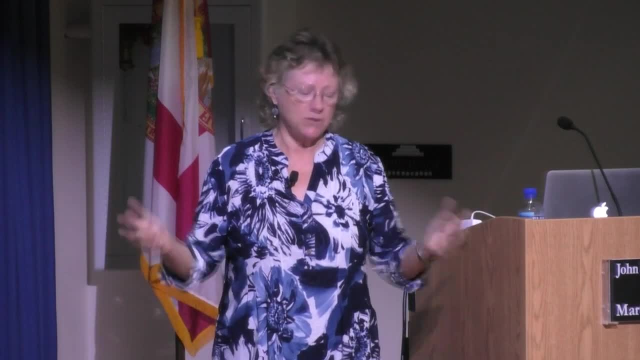 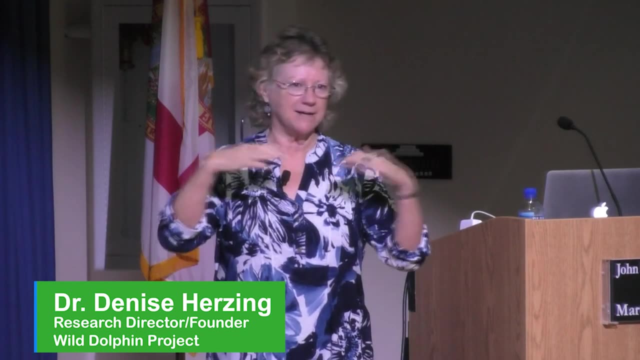 they fight for all of it, right, so when they're fighting. so what you saw was pretty toned down, you know they're. they're doing head-to-head postures, like you might see. you know rams, you know ramming each other. they open their mouths, are making 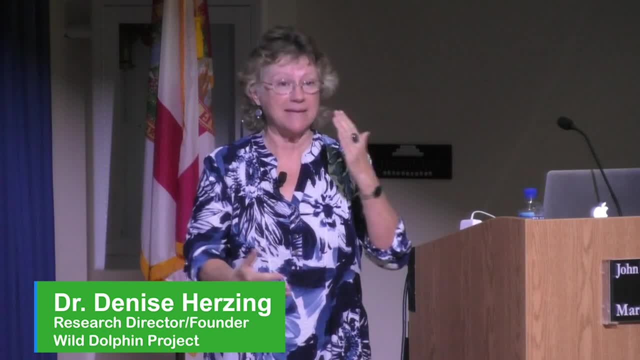 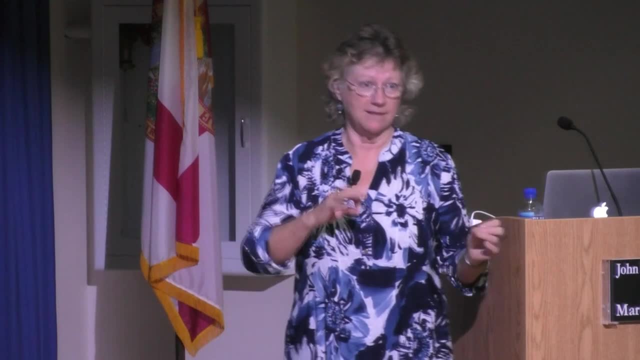 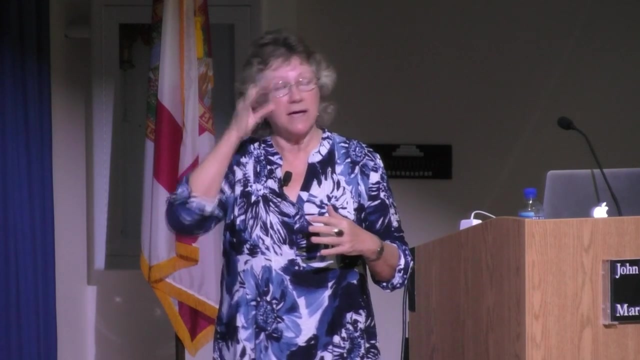 sounds, but they'll. they'll ram and charge each other, they'll slap each other hard. I mean, there's never been a dolphin. well, I take that back. there's never been an observed dolphin death during fighting, but dolphins are known for infanticide also. so yeah, so there's been a lot of strandings of calves. 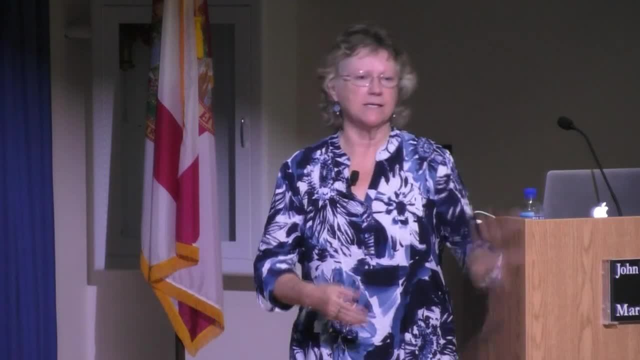 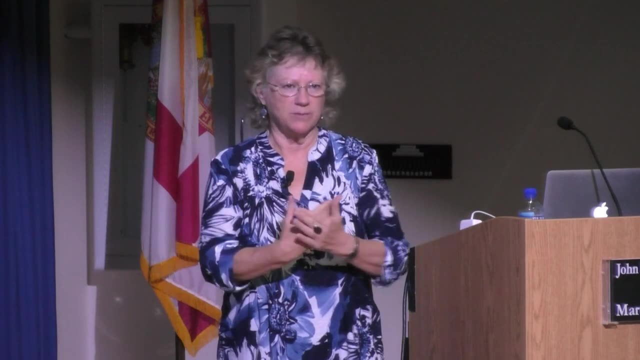 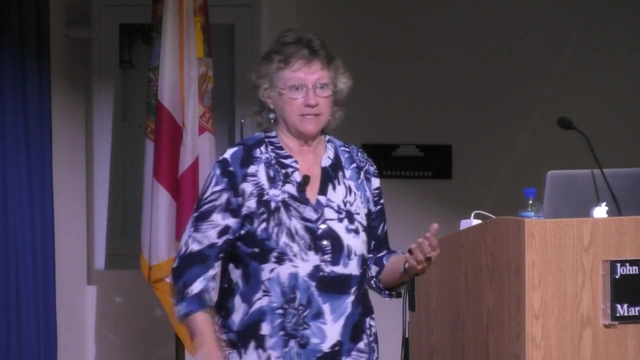 dolphin, a bottlenose calf on the east coast and they look like they're really impact marks, you know, from bottlenose probably slapping them around. and in the Scotland area the bottlenose kill harbor porpoise. they toss them around. nobody knows why, but 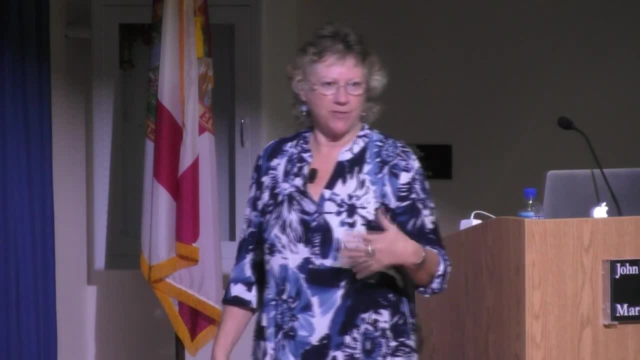 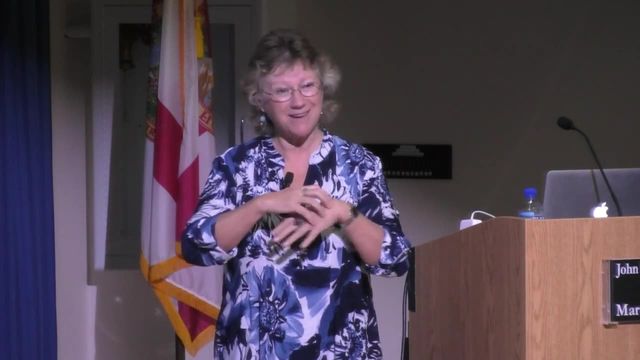 just blunt impact. I don't know if they think they're toys or they're threatening them, but no, they fight. they fight with what they have. their tails are really strong, their flukes are really strong. they can make really deep rake marks. we have never seen a spotted dolphin really hurt each other, but I've seen the. 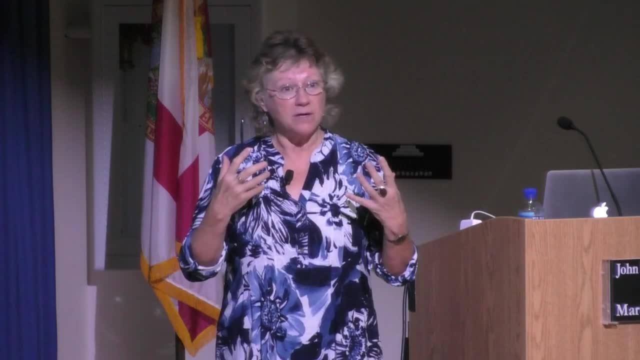 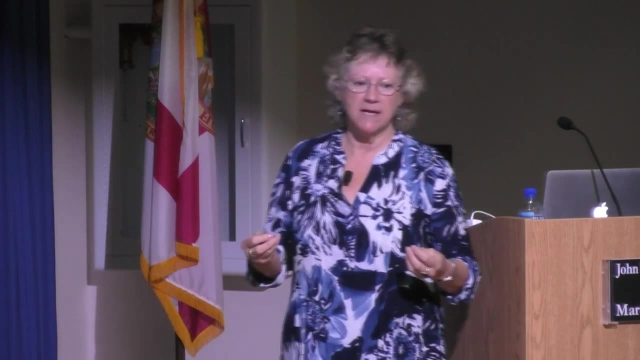 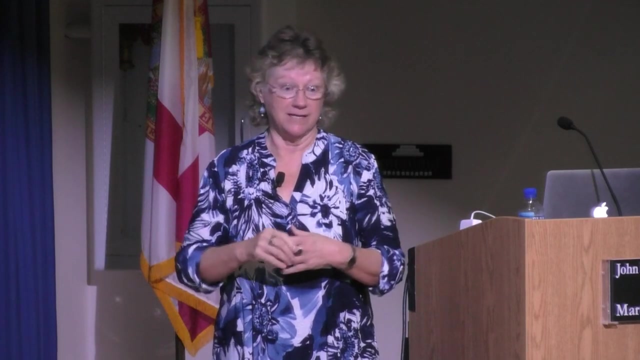 bottlenose fight big time and the sound. so sound is much more potent underwater than in the air, like the decibel level, so it's like a- you know a exploding gun cap under the water. it could actually really hurt your ears and I've heard sounds where it's like, yeah, and they could hurt each other with sound right. 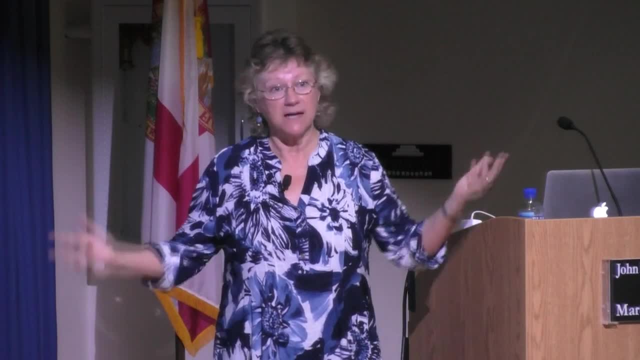 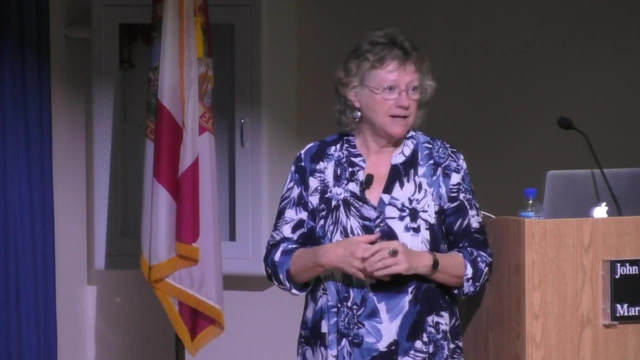 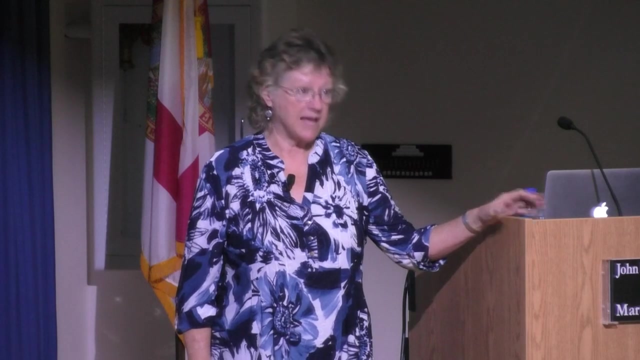 protecting sound? yeah, like a big, like a gun, actually underwater. yeah, I think it's a good question. Are they ever aggressive with people and have dolphins ever documented being aggressive with people? Yeah, are dolphins ever aggressive with people? yes, they have been both in captivity and in the wild. you know, my suspicion is because people are doing. 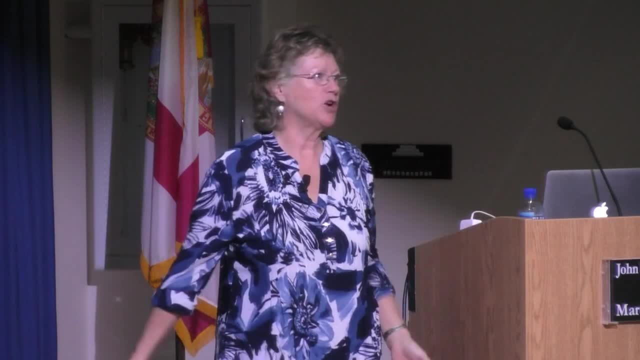 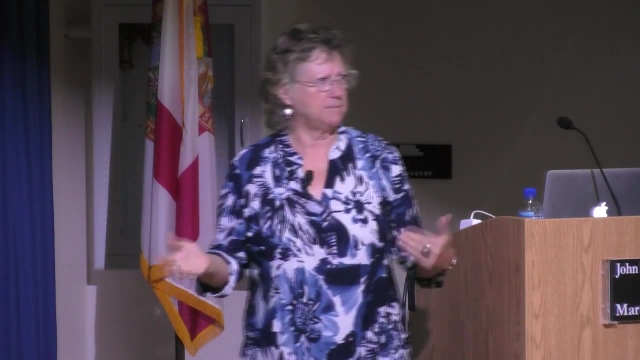 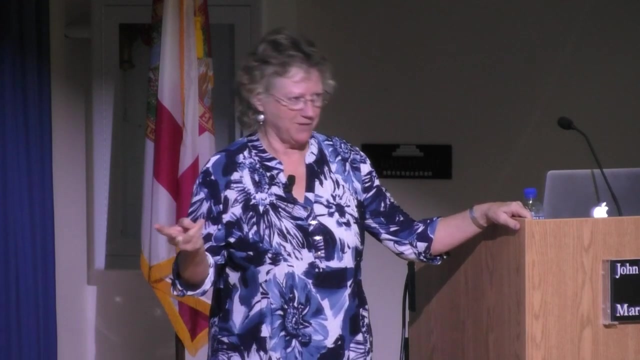 stupid things to the dolphins, right? I'll give you an example. there was a friendly dolphin off the coast of Brazil for many years, a while ago, and I believe it was a female bottlenose and you know, kids would swim in there and blah, blah, blah. and I hate to say it, but two Americans were. 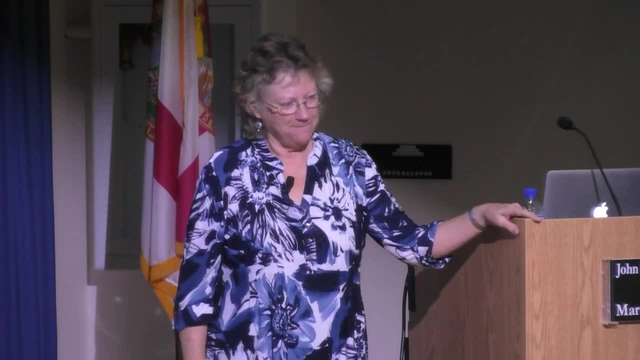 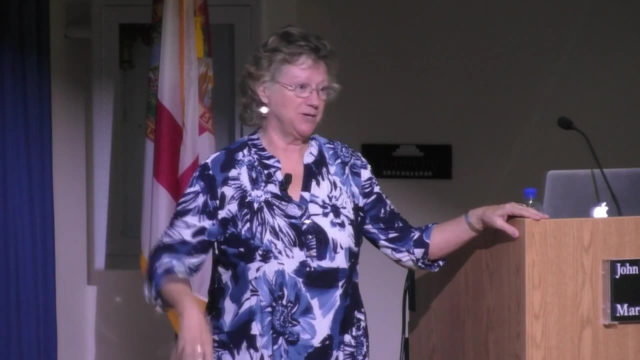 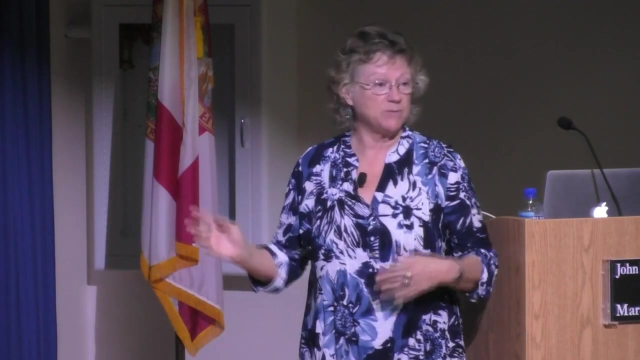 down and they decided to jump on her and stick a cigarette in her blowhole. so guess what the dolphins gonna do. I mean, if you jumped on someone in New York City and did that, you know he wouldn't last very long, right? so I think she actually, you know, slapped him with the tail and one guy died from internal. 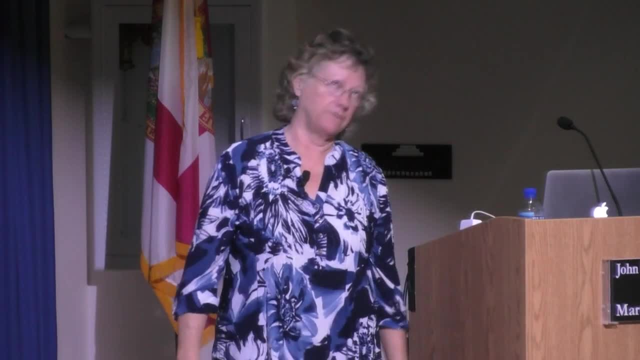 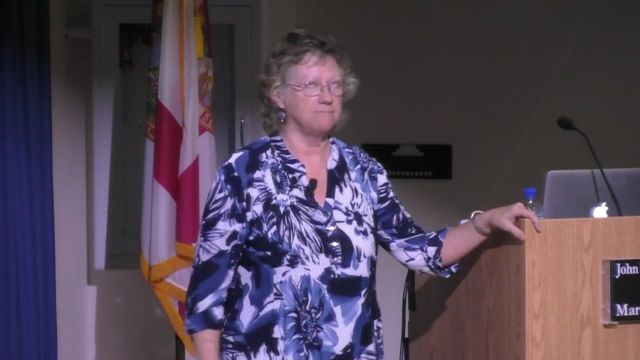 bleeding. so now they have a killer dolphin like really, yeah, seriously, so they were thinking of moving, trying to move her somewhere, and then finally there was a biologist, Marcos, down there, and he finally tried to explain to him that it's like it's the human behavior that you know she's defending herself. 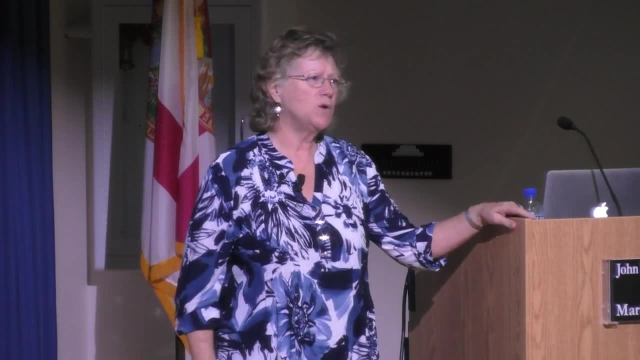 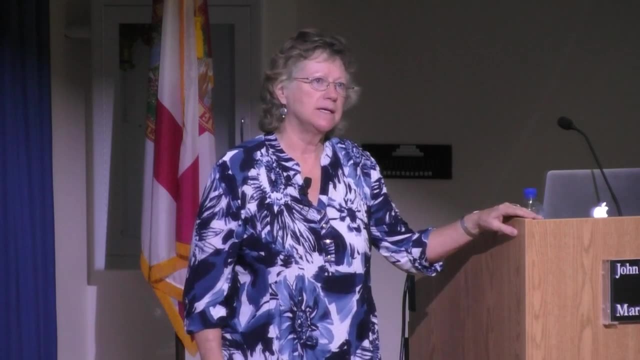 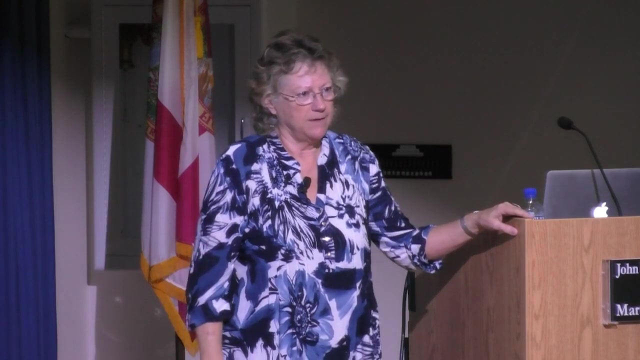 etc. there are other a few other kind of fluky instances. there was some weird instance off the Bahamas not so long ago where some woman was just swimming and I guess a dolphin came and beat her up. so you kind of go, did the dolphin just jump on her? 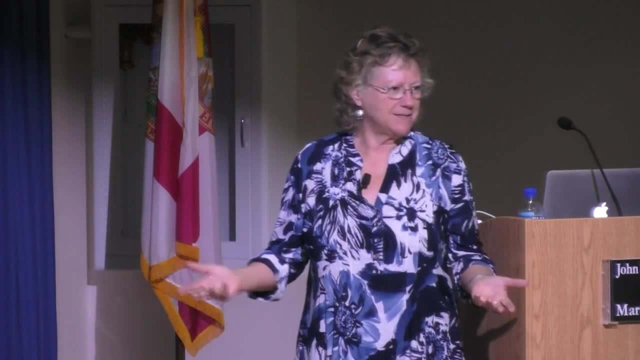 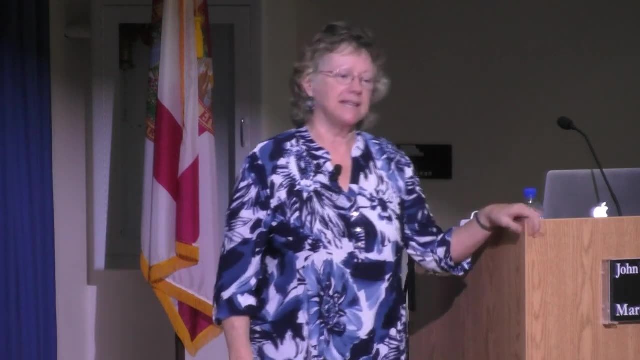 was it neurotic? Did it get injured by a human and it was pissed off. I mean, you don't know what you know these animals have had in their lives, right, what's happened. you know So, but I wouldn't say it's common. but I would also say that 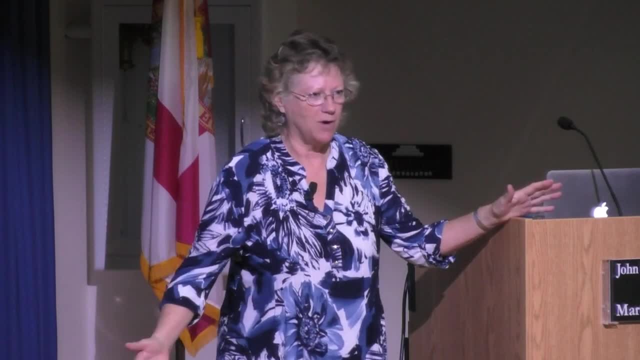 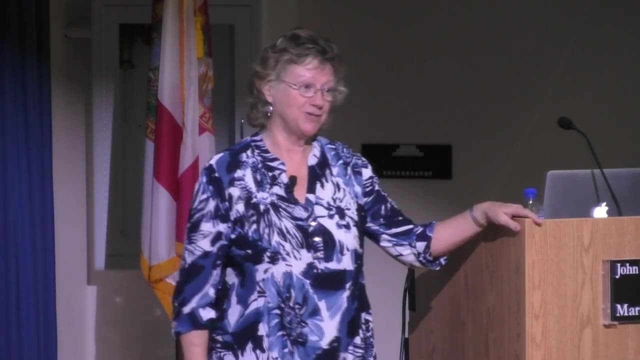 not every dolphin in the world wants to have a human in the water. you know They have their lives- right, I mean their lives. they don't need us. you know They have plenty to do and interesting lives without us. So when you try to get too 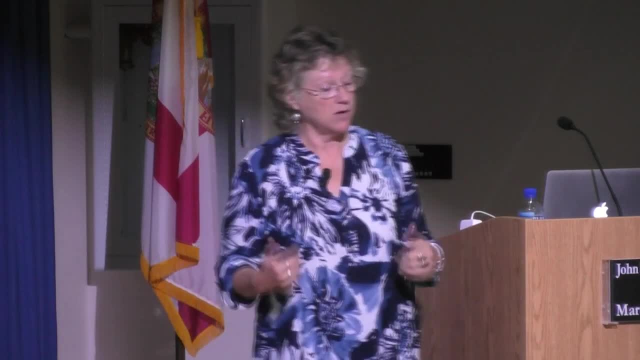 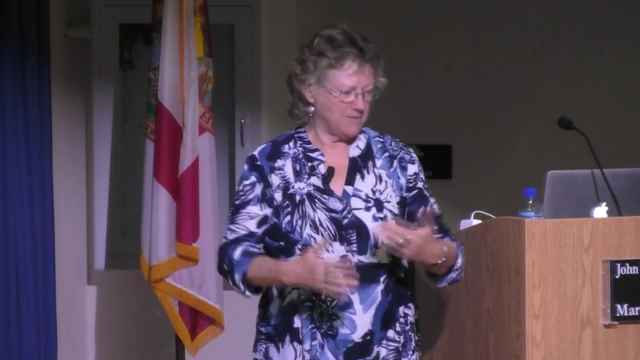 friendly with them or you try to disrupt their behavior, like, for example, our work because it's in the water. we're really careful about how we act. you know, And we think we know a fair amount about their etiquette and how to behave, but if they 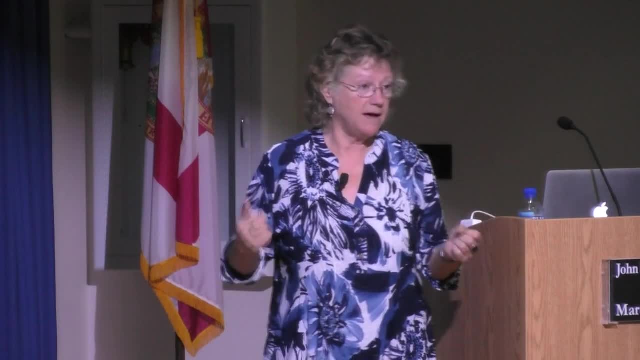 give us signals, sometimes like they don't want us in the water and they have, you know, they'll come up and they'll go, uh, and we're like, okay, we'll go back to the boat now And we get out of the water because we're like okay. 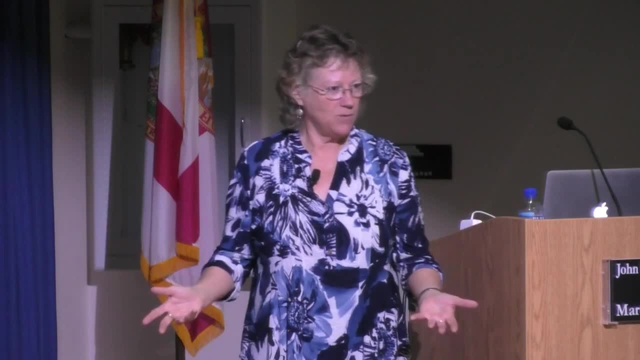 They're nicely letting us know that they just don't want us in the water and sometimes we don't know why. We didn't feel like we did anything, but it's not so bad. But it's just like they want to be alone or left alone. 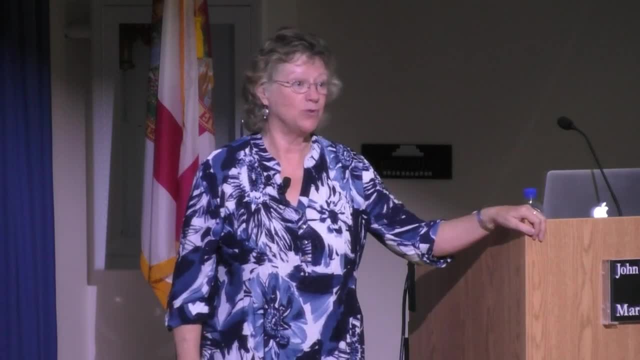 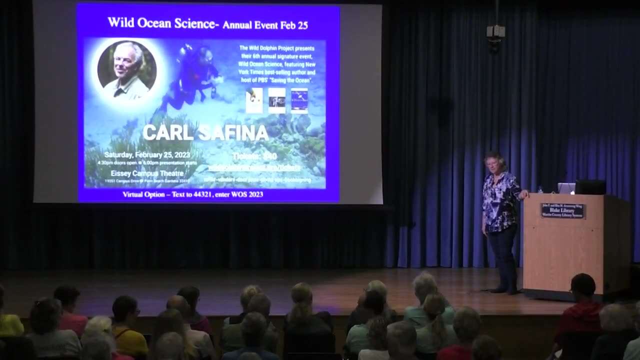 or maybe they were annoyed by five boats that day. You know, you just don't know. So you have to be cautious. When dolphins follow a boat, what is that behavior? Is that just playing with them? When dolphins follow a boat and jump in the wake, you mean? 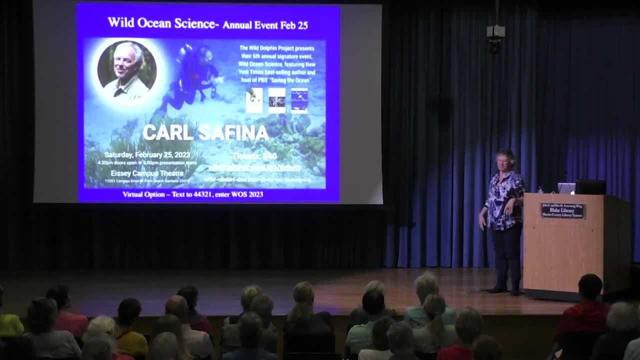 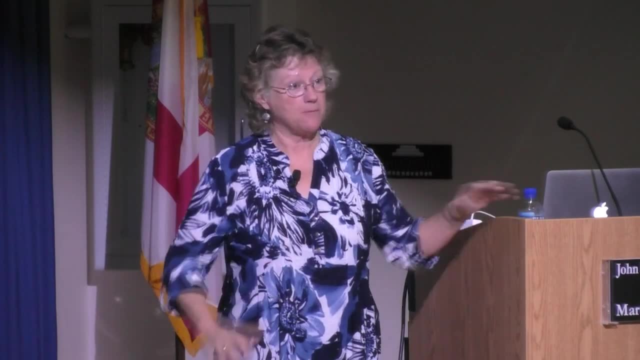 Oh, that's just fun. They're having fun. They're having fun with the boat. They're having fun, They're surfing. Yeah, yeah, that's fun And it's a free ride. You know, they get a free ride in the bow right. 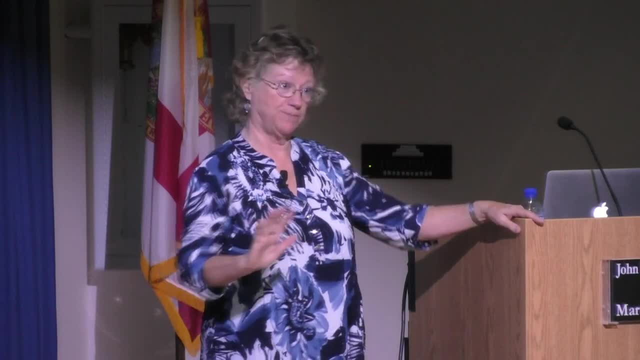 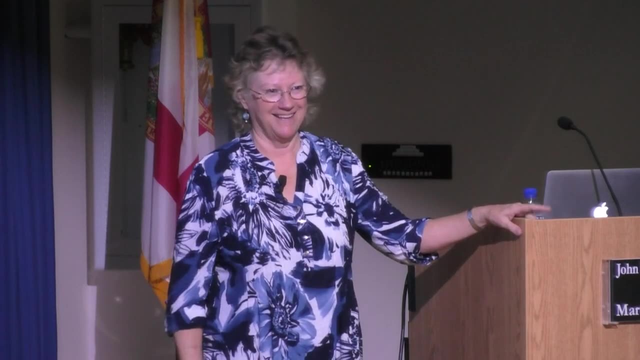 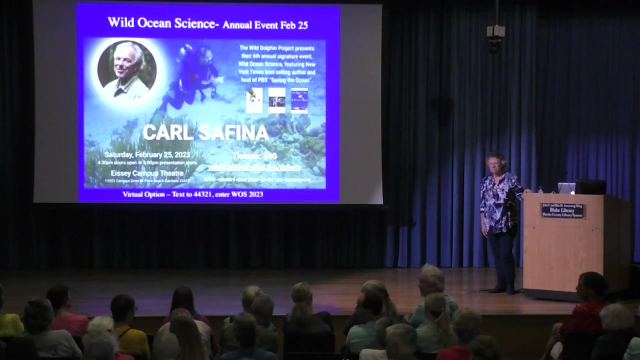 They're pushing ahead And they actually bow ride whales because whales will make such a push that they'll like, so we didn't invent that with boats. How deep do dolphins dive? Do they have to decompress? So how deep do dolphins dive? 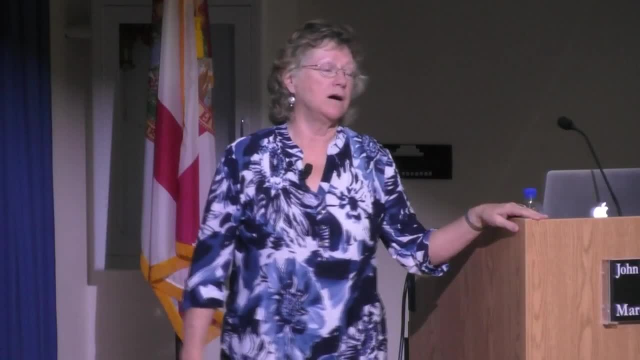 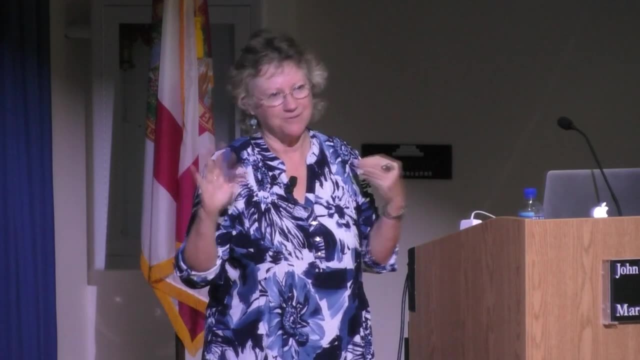 and do they have to decompress if they go deep? So I guess the answer to the second question is no, because they are taking one breath at the surface, They're not breathing. They're breathing compressed air, right, So that's a good thing. It depends on the species. There are over 30 species of dolphin. Not all of them have been measured. Some of the larger dolphins, like pilot whales, which are actually a dolphin, believe it or not. they can go to 1,500 feet, say. That's not unusual. Some of the seals and sea lions are actually better divers, believe it or not, They're like master divers. You know. they go up and down, up and down Sperm whales, which are toothed whales. 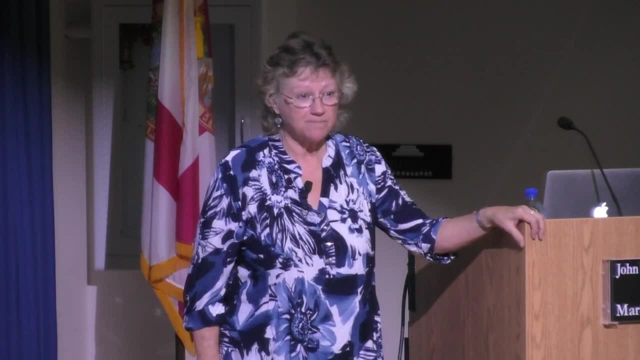 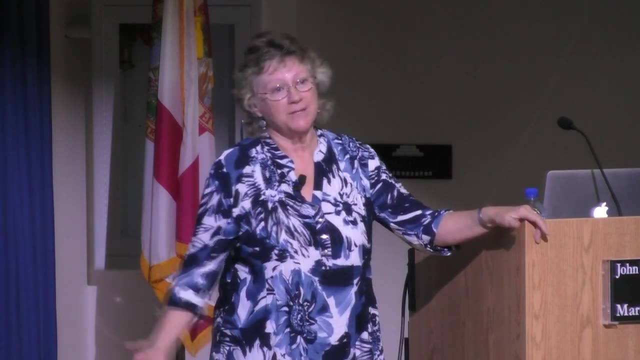 they're actually better divers. They'll go two miles down, But they really. you know, everything gets kind of sucked in and they're just doing the important stuff. But yeah, I mean, they're designed for that basically. 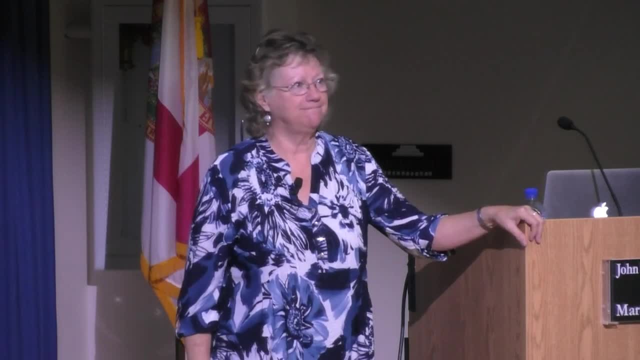 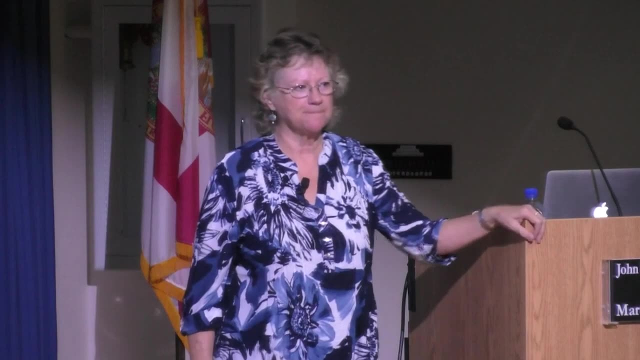 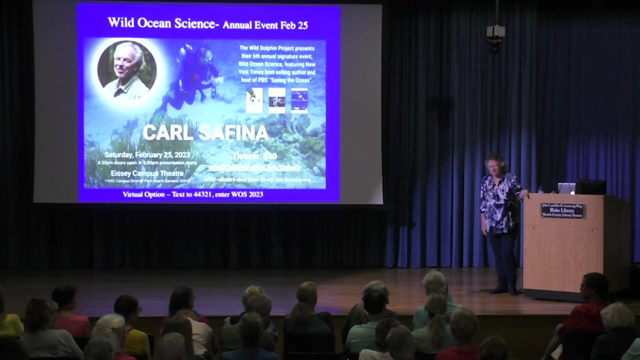 But you know, your average dolphin that you see, probably 300 or 400 feet maybe, maybe deeper, but it probably depends on the fish they're chasing. Yeah, Yeah, So among the population, has the most experience with this? 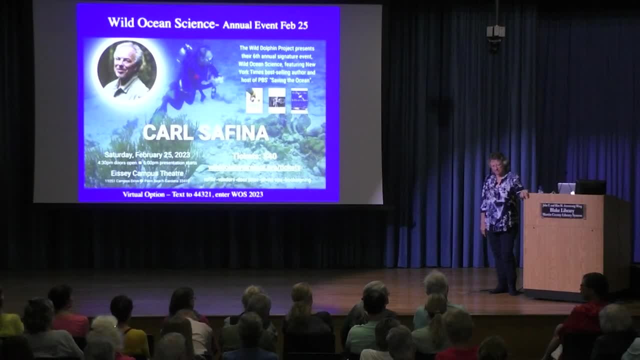 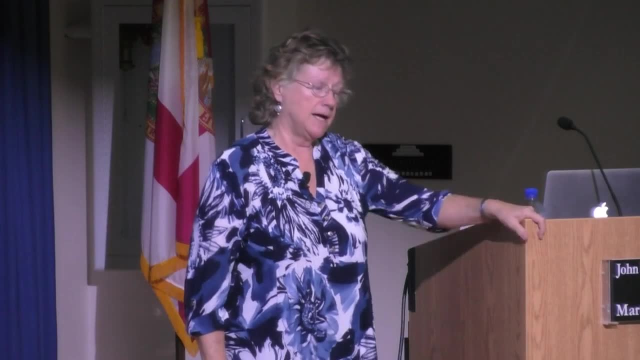 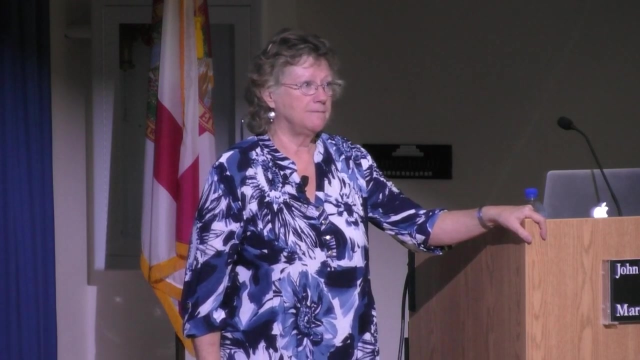 The local dolphins have their dorsal fins bent. You mean the ones in the Indian River. What's the reason for that? Well, I don't think it's common. It does happen a lot in captivity. I would speculate. it's probably nutrition, maybe. 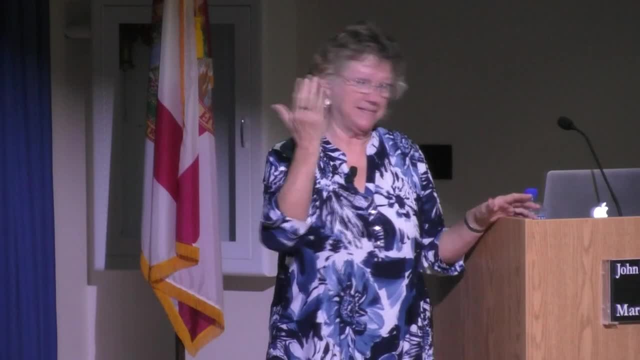 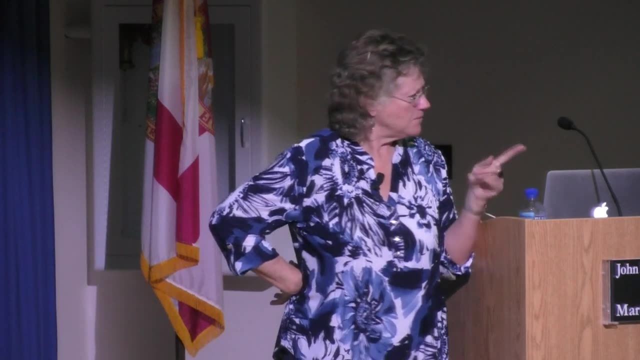 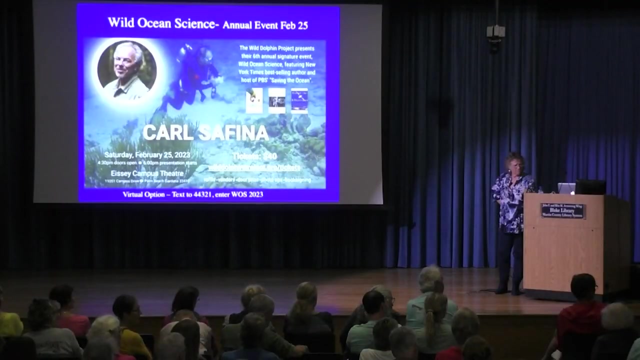 It wouldn't be normal, just because you know they're meant to be a stabilizing element right on their body. Yeah, I don't know. I'm not sure I've seen any photos of their Nick. So Nick was just saying that sometimes their fins are cut. 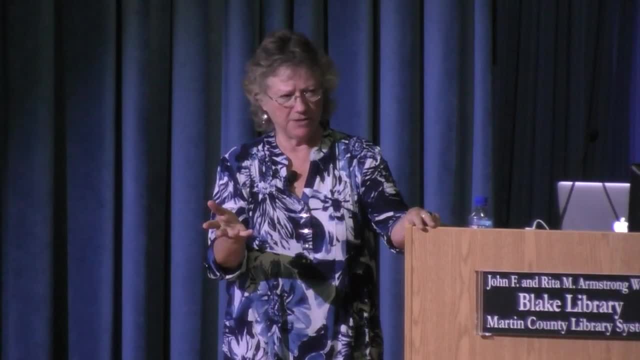 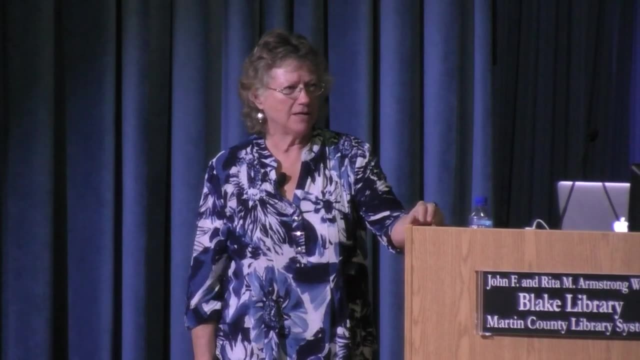 or bent over from monofilament or boat injuries. but that's not a normal bend, That's a chop. Yeah, Which is a little different. Oh question from Yeah. we'll jump in with a Zoom question. How does the behavior of spotted dolphins? 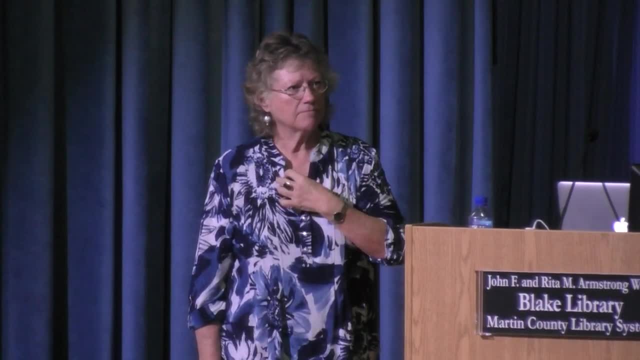 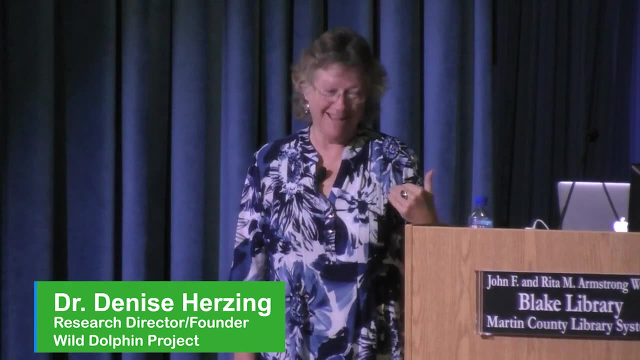 and bottlenose dolphins differ so that they can coexist in the same niche or habitat? Good question. Well, our sense of it. I might be a little biased, but the bottlenose dolphins' temperament is quite different than the spotted's. 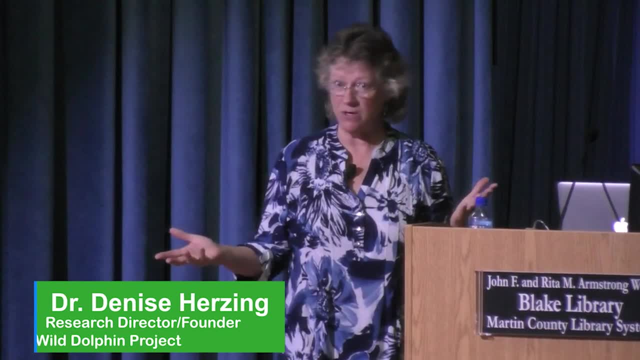 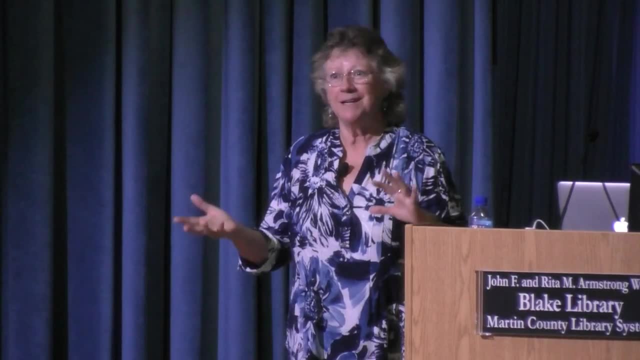 They're a little more aggressive And this is the species we know the best right from coastal work, from marine production, marine parks. The spotted's are a little more playful, not as aggressive, But, like I showed you, there are some interspecific things they do. 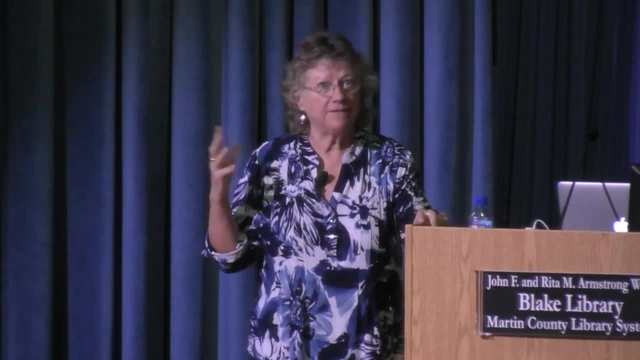 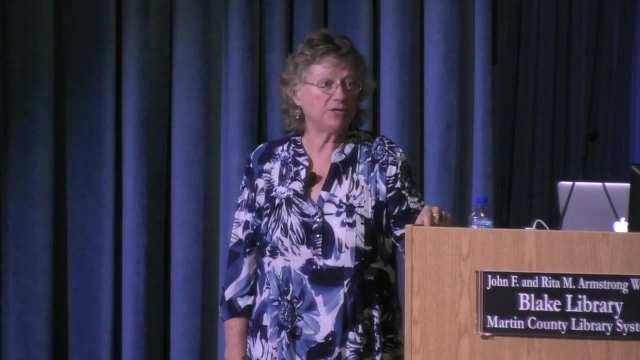 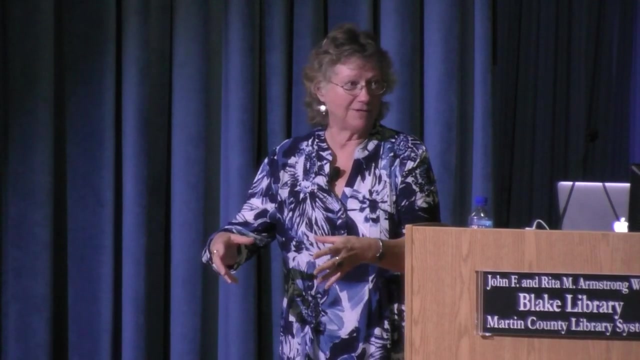 you know, babysit each other's calves. They fight sometimes but they help each other. So I guess it's getting to know your neighbor and developing specific relationships with your neighbor too, Like we'll see sometimes traveling pregnant spotted dolphins with pregnant bottlenose dolphins. 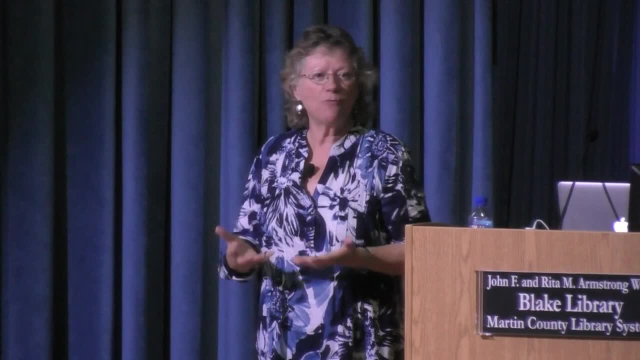 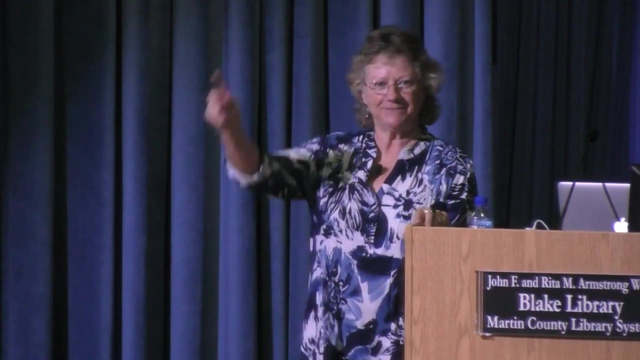 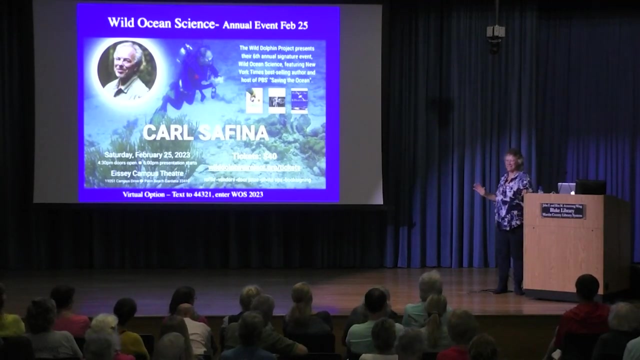 So, like you know- yeah, I know So clearly they recognize the other species. I guess it depends on you know what's at stake. basically, When do dolphins sleep? Ooh, the question everybody always asks: When do dolphins sleep? Well, they don't. That's the first answer. So what it looks like dolphins do is that it looks like they shut down half of their brain at a time To rest right. So the studies that have shown that they kind of go. 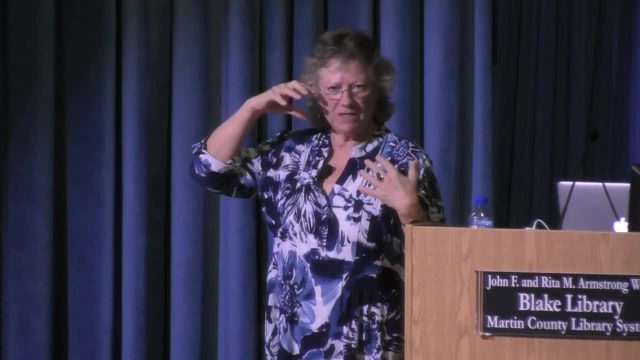 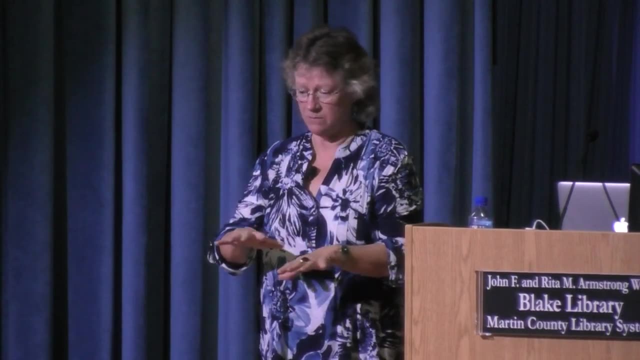 into like a meditative brainwave state on one side and the other side stays active. So they'll- and I've seen it in the wild, actually They'll- be swimming in the water column And it's like you look at them and their eyes are closed. 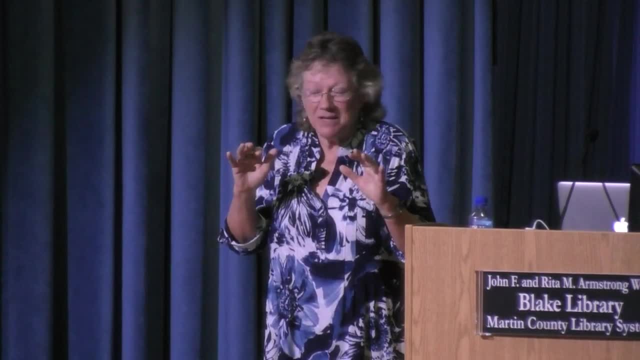 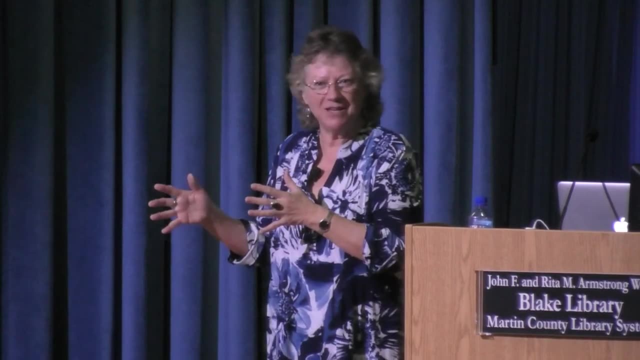 But as soon as you make like one little click or just movement, they're like you know, all of a sudden they're alert. So they rest on one side of their body And they keep the other side of the body awake. Yeah, which is interesting. 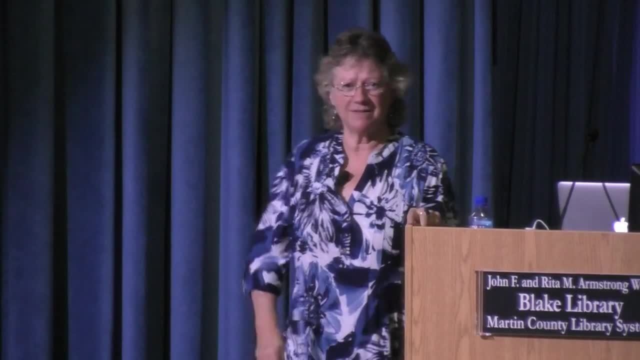 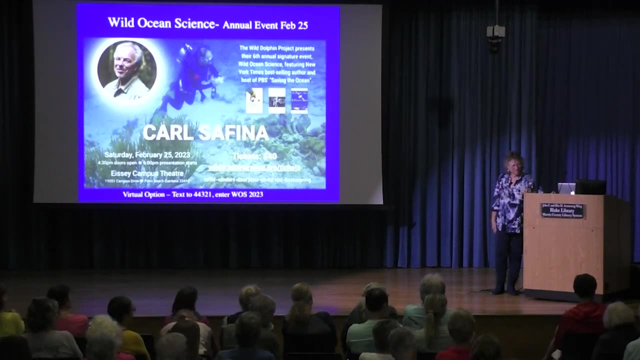 So I don't you know they don't sleep like we think of sleep. Could you like put monitors on the dolphins to see where they're moving, Like they do with their driving the way over? Yeah, the question is, could we put monitors on the dolphins? 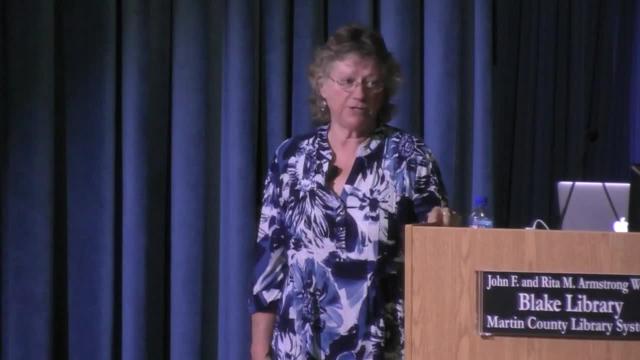 to see where they're moving. We could, We choose not to, Because you have to kind of capture them and drill a hole through their dorsal fin And you know it's a lot of work. It's a lot of work. 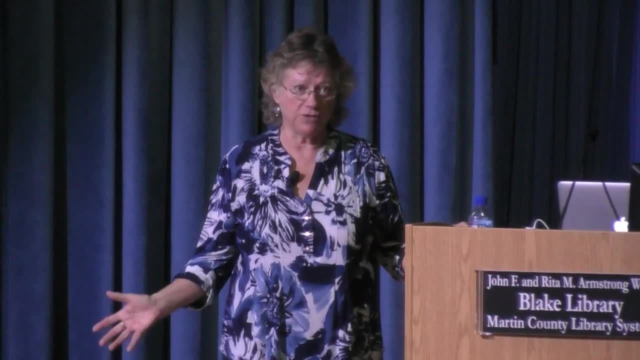 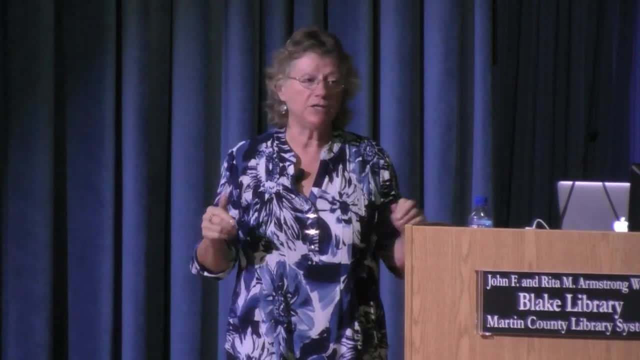 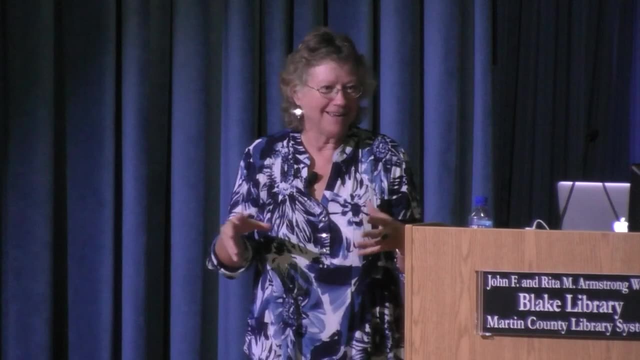 But now you can satellite tag. Yeah, it'll tell you where they go. You know, our sense of our particular study area is the animals would never hang around with us in the water if we grabbed them. So we don't really do that. 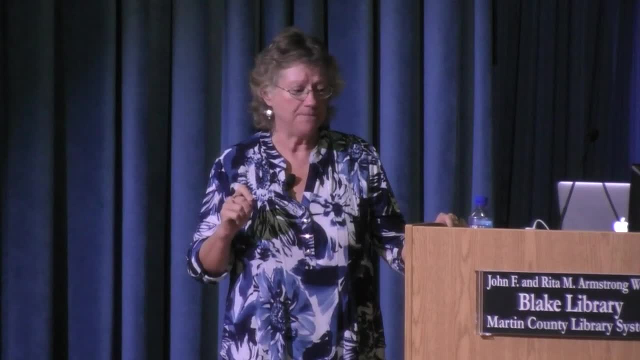 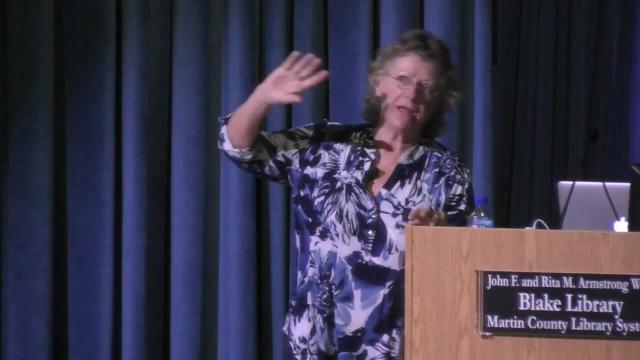 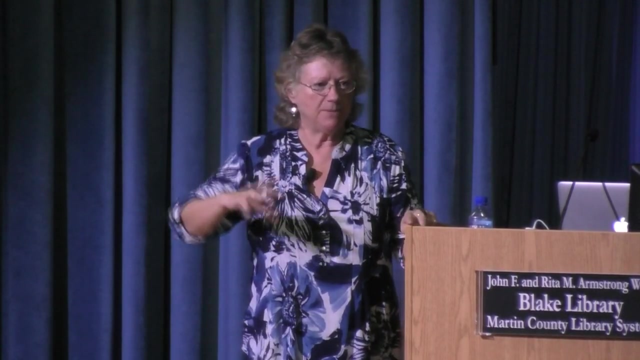 Now I will tell you that we had a stranded spotted dolphin in 2018.. He stranded in the in the Bury Islands, which are kind of way east of Bimini, And he was rescued. He was flown to NASA and rehabilitated. 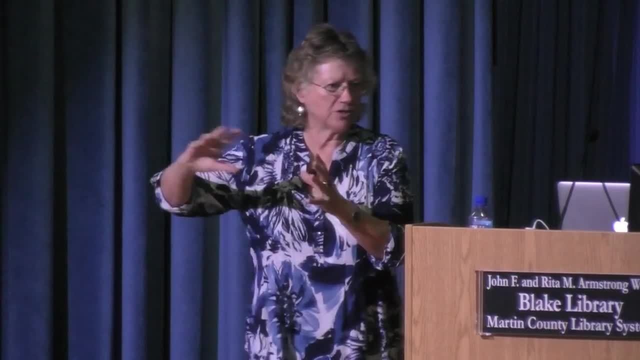 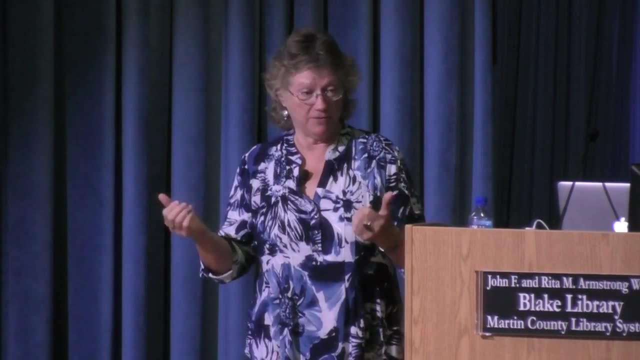 And we saw his photograph. some other researchers we know were working there and we could identify him. He was one of the males from our group, And so the Bahamian government, after he was rehabbed, allowed us to release him back with our group. It was incredible, And so in that case he was already out of the water. So we did put a satellite tag. We put a satellite tag on him And that guy took off. he went 120 miles the first day, The second day, another 120 miles. 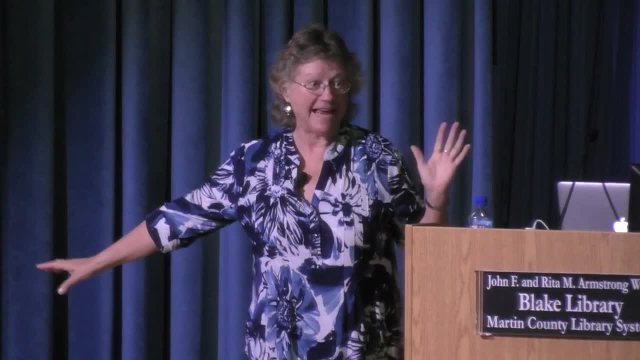 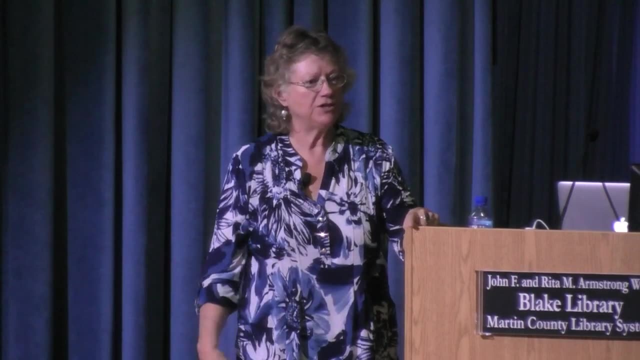 He went almost to Cuba- And this is from the satellite data. Hung out there for a month Still in the Bahamas, but right out the edge of the Seme. Then finally came back to his regular group And he's happy, happily living with his regular group again. 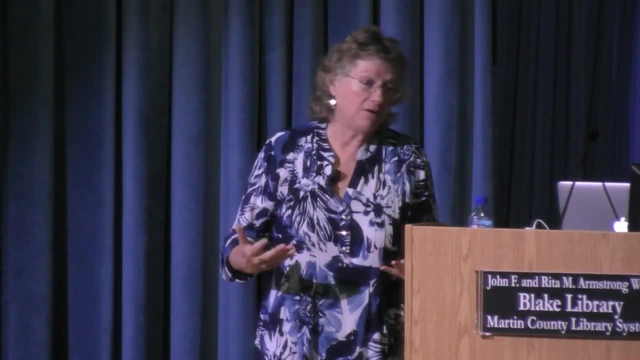 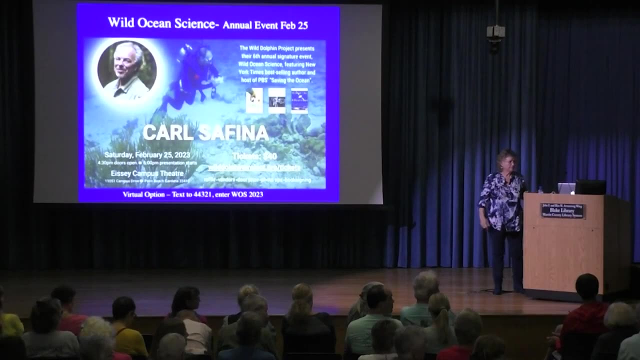 So it's a great tool, But you know, do you have to tag them all? You know it's tough to decide how you're going to do that. Another question: We have another question from our Zoom audience. Actually, this is a two-part question. 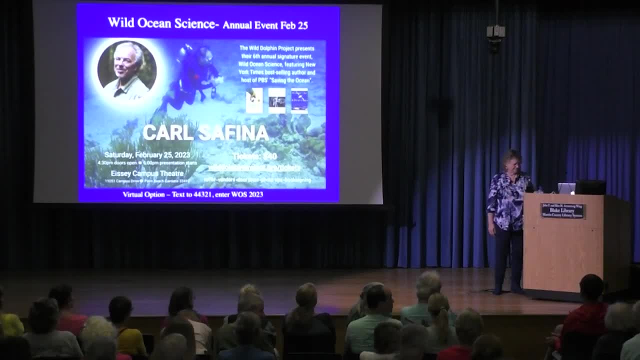 Are there different dialects among dolphins from different regions And is there anything that a general citizen can do to volunteer to help with the Wild Dolphin Project? Ooh, good question. Yes, dolphins do have dialects. In fact, they can be really different in adjacent groups, right? 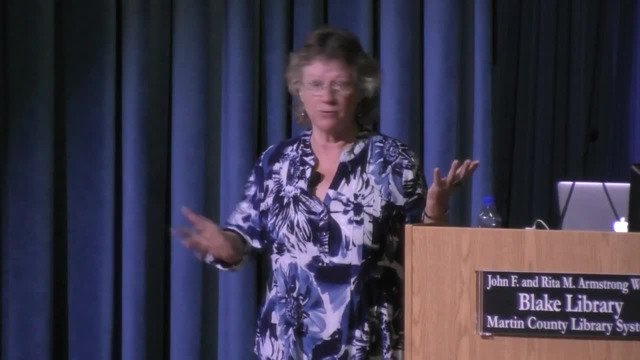 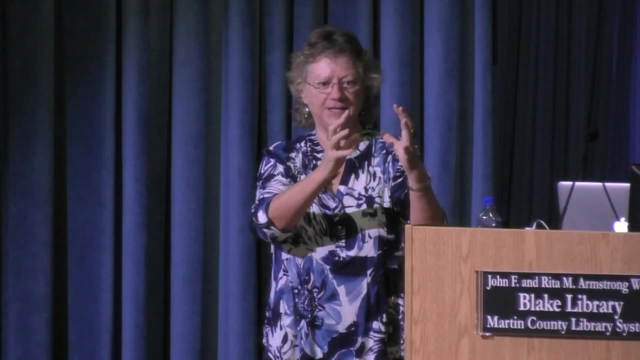 So yeah, it's all about the group, Like how do you know what your group is? So kind of think of it as like they have a species sound and then they have dialects. Well then the species and then the pod probably has a little bit of a dialect. 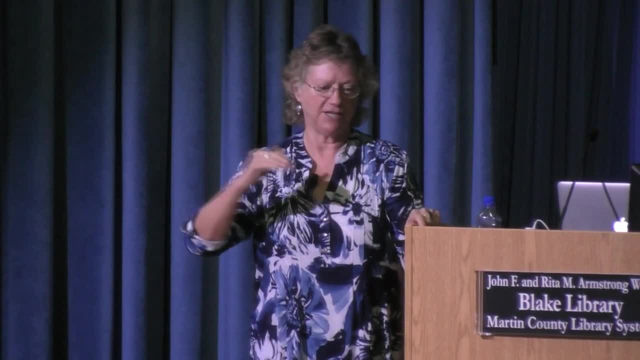 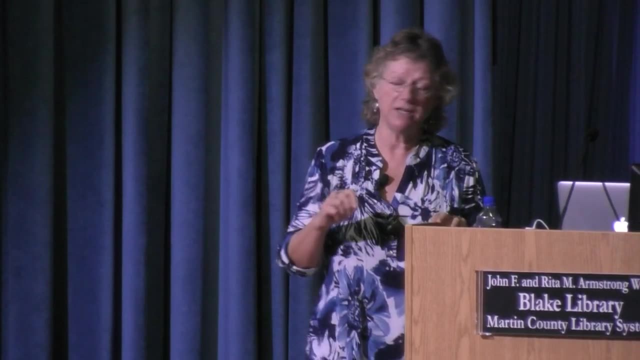 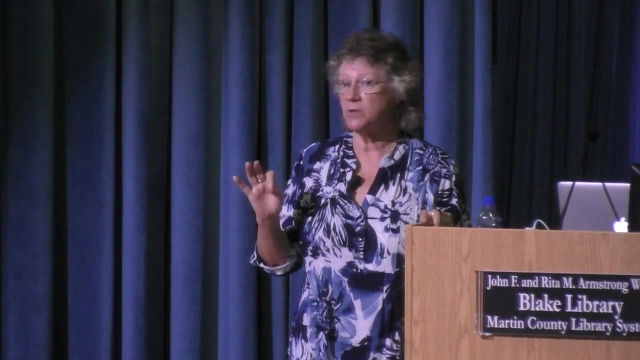 And then they have their signature whistle. So there's all these levels of identification. And, yes, Wild Dolphin Project has an online site. If you get a photograph of a spotted dolphin in the Bahamas, you can upload it, And it's through Fluke Books. 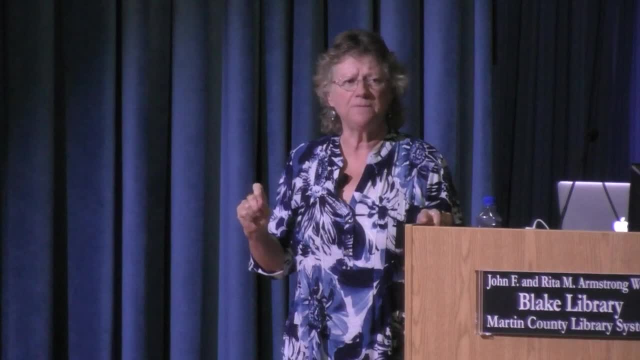 You can look on our website And it probably is in our newsletter too. And, yeah, that can help us identify If you could tell us, If you could tell us where you took the photo, and we'll tell you who that dolphin is. 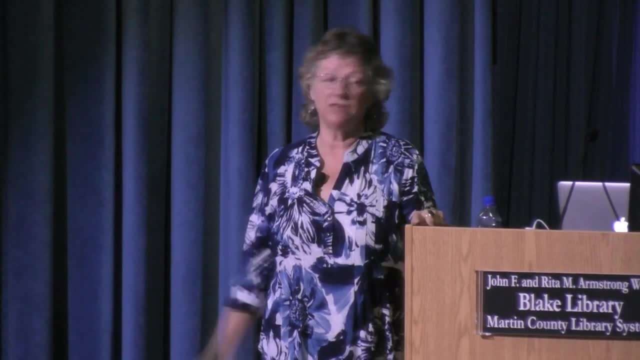 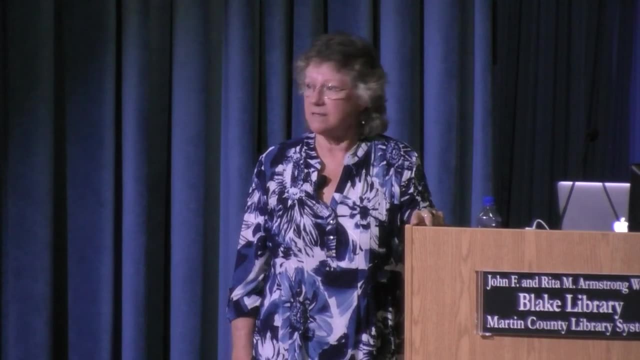 And that really helps in location. We have events you can volunteer for. You can come on the boat with us in the summer as an ecotourism kind of thing and help out, And yeah, and you can send money, large money. 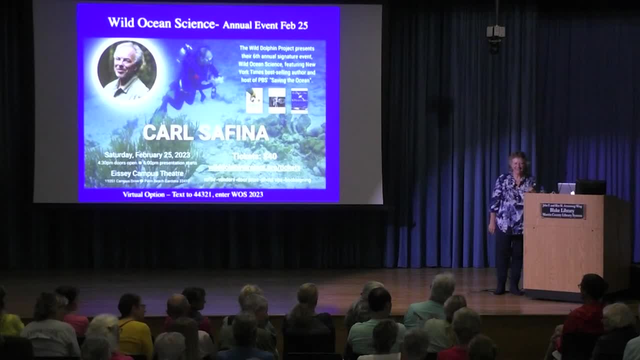 Just kidding. I'm here to see if you're able to get any acoustic data, either before hurricane or after, or or like during- Before, during or after a hurricane. Oh wait, a minute. during a hurricane, Can we get acoustic data? 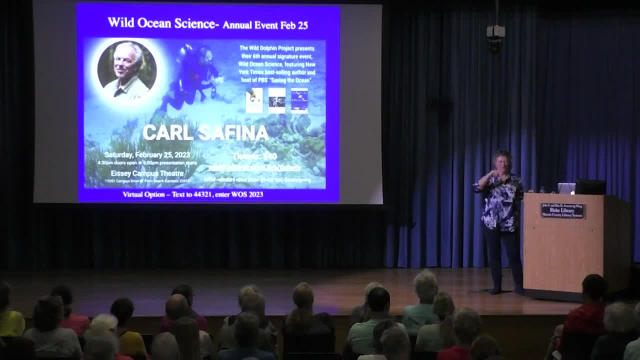 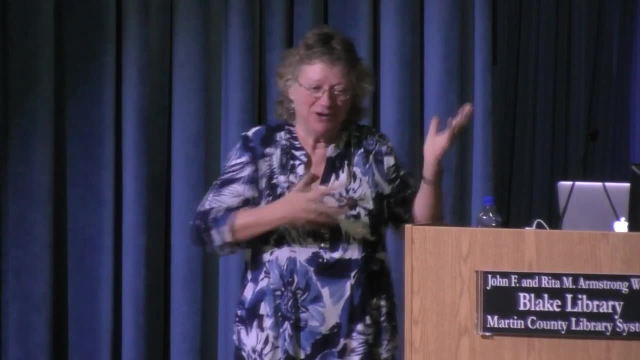 Can we get acoustic data before, during and after a hurricane? People usually say: what do they do during a hurricane? And we're like: oh, we're back in Florida And even our acoustic devices, we have to pull them up off the bottom. 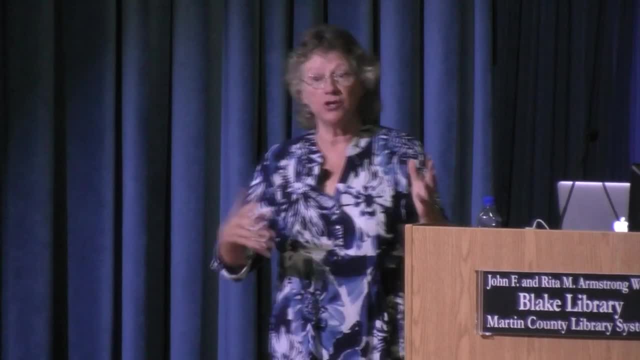 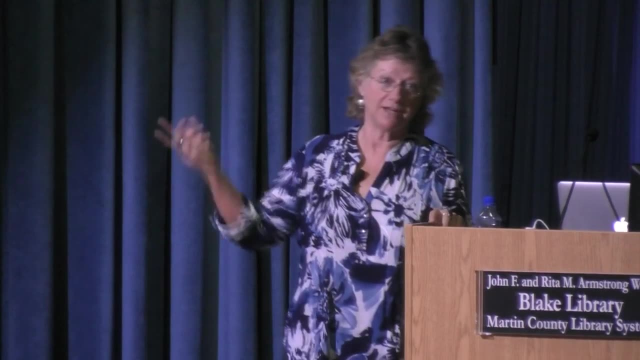 because they can just be lost, right? Yeah, so of course, sure, right before we leave, But then But it's hard to get. Yeah, You can't get back there after a hurricane, literally Like usually after the hurricane's. here we've done relief runs for the locals, basically. 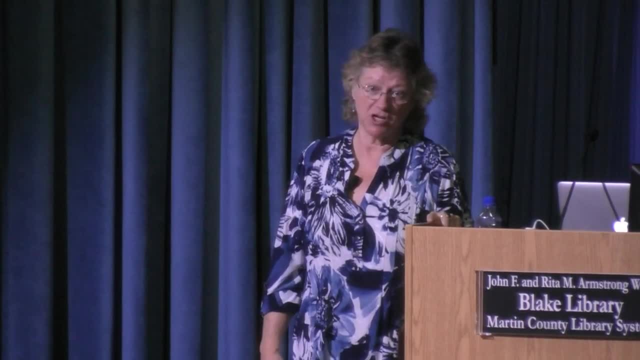 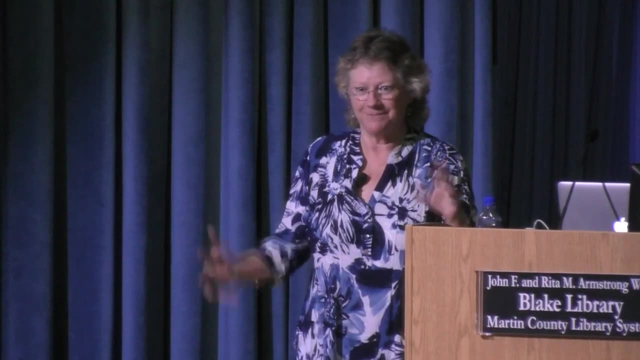 We load our boat. you know we, our benefactors, often give us a chunk of money to go buy generators and stuff, but we just load our boat and go over there and give them stuff, But and then we look for the dolphins, like you know. 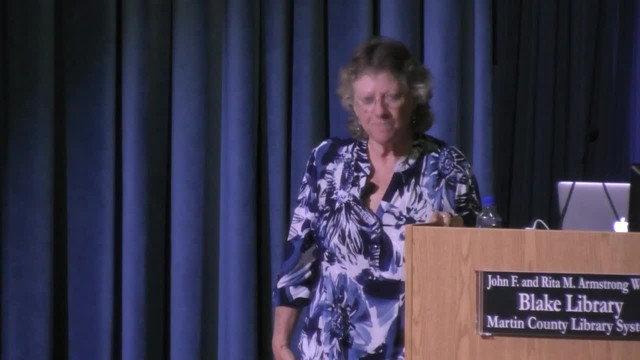 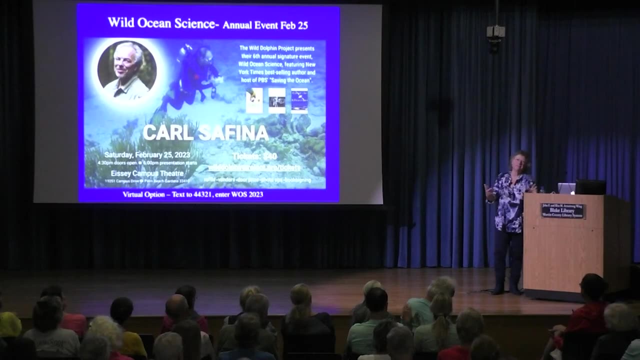 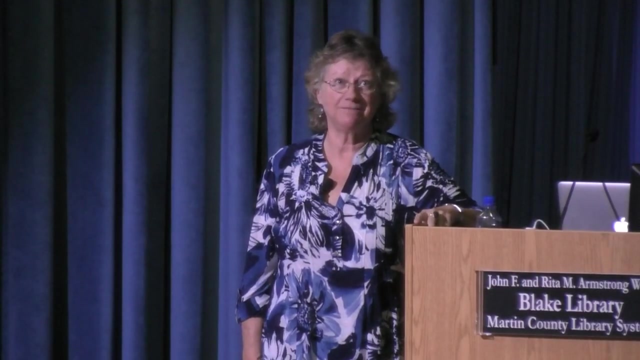 But we don't often have a lot of time. Yeah, no, I wouldn't. I wouldn't say, but you know What is that? like you know, we would leave, depending on the hurricane, you know, days. 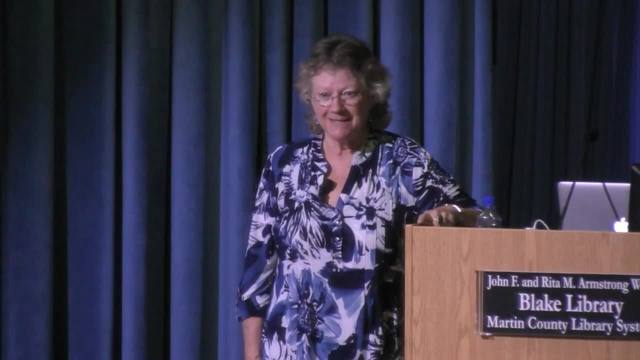 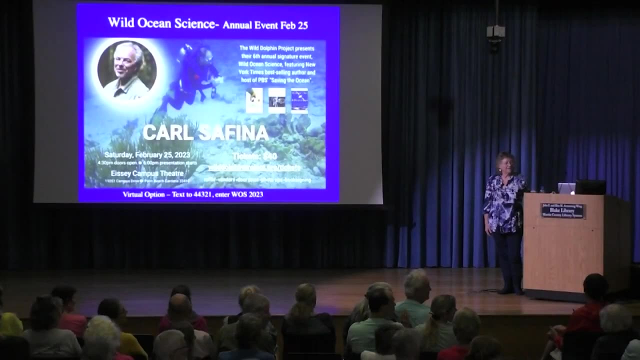 if not a week before, if we saw something big coming, and yeah, it'd be interesting. though, yeah, We have a hurricane follow-up question online. You mentioned a number of different hurricanes that impacted the Bahamas, but you didn't say anything about Dorian. 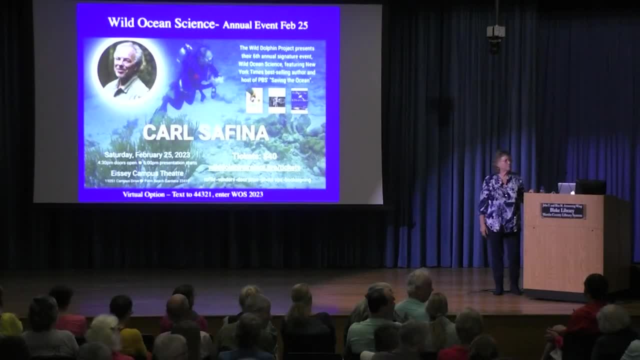 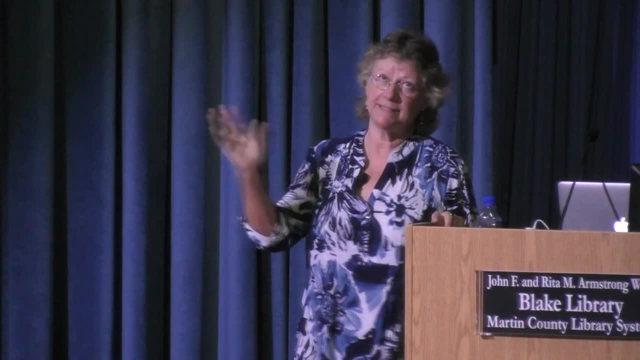 Do you have any data that discusses the impact of Hurricane Dorian on your study populations? Yeah, so Dorian actually Stopped. that was a monster. It's, as you know, the Abacos. it stopped in the middle of Grand Bahama Island, over Freeport right. And then it kind of went north. We didn't. we don't think it had much effect on our spotted actually, because they're mostly to the west enough. I guess that it made a difference. I know the Abacos dolphins had some effect. 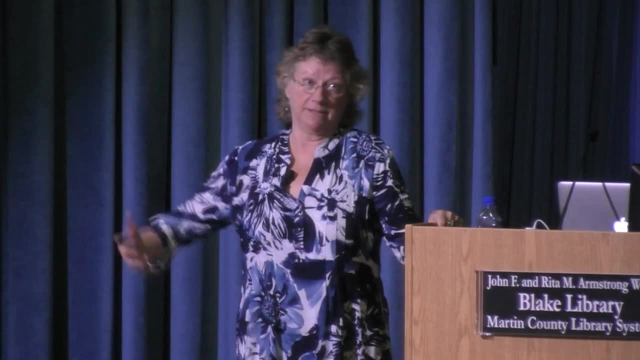 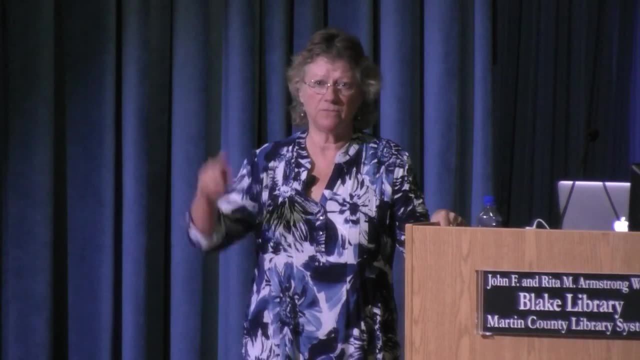 They studied the bottlenose over there, But still, I'm sure there were big seas and challenges, you know, But no, we haven't seen any direct So way back there, When you observe dolphins in the open ocean, do you use re-breathers or do you use scuba? 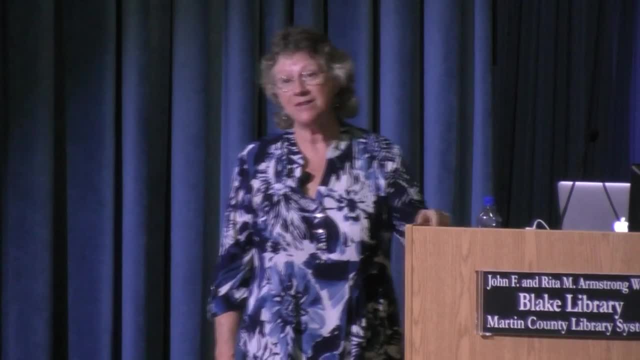 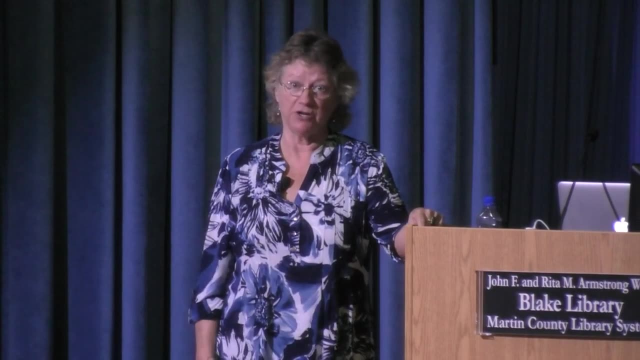 When we observe dolphins, do we use scuba or re-breathers? Neither. We actually just snorkel Because we're collecting a lot of acoustics, although re-breathers would be potentially good for that because they're quiet. Scuba: it's a little noisy because of the bubbles. 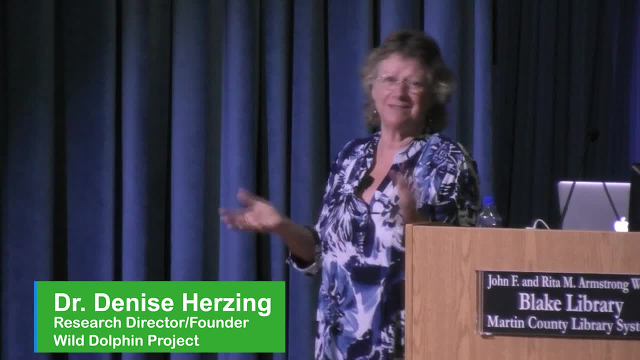 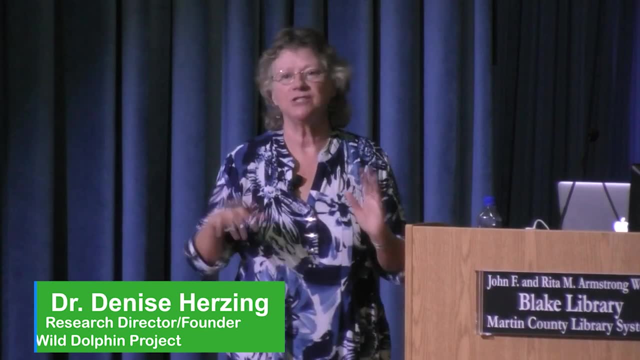 And the bubbles actually kind of disturb the dolphins sometimes, you know, depending on you know they use their own bubbles for aggressive things Sometimes. So we just snorkel. We find it's just easier to keep up with them and to maneuver. 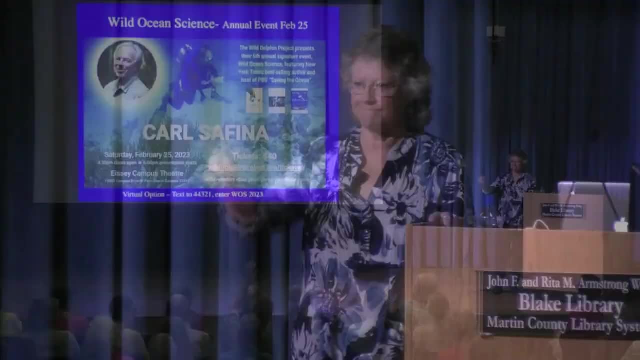 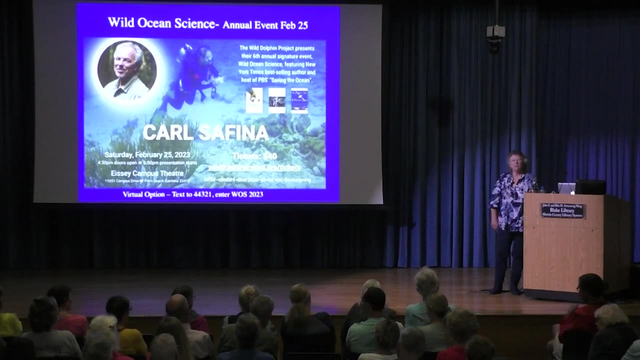 And we free drive a lot. basically, You said there's a 30% mortality rate in hurricanes. Do you have any idea how they died? Well, I should clarify that we're not sure they died, But we certainly haven't seen them anywhere. We've looked or, you know, found any matches anywhere else, So we assume they died. My guess is drowned Drowning would honestly be exhaustion, and drowning or predators. You know, you've got sharks. They don't need to breathe, right. 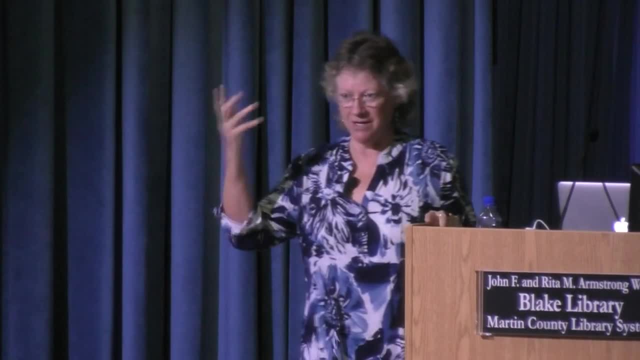 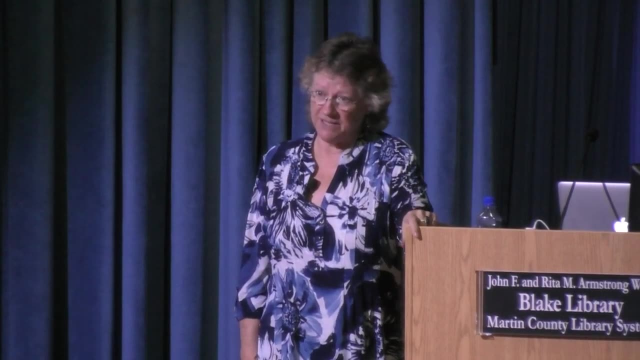 They can stand in the water. You've got dolphins that have to get to the surface and breathe and, you know, eat and yeah. So we have never actually seen a dead dolphin in our area. They just kind of are gone. 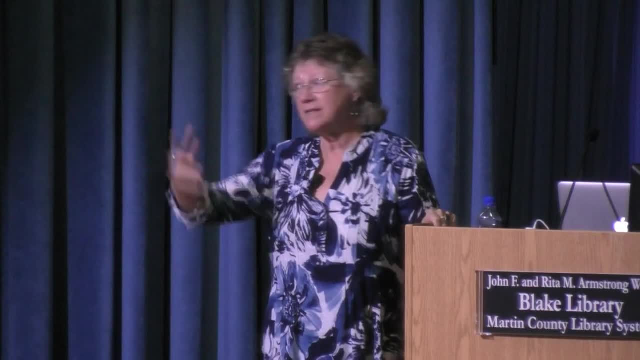 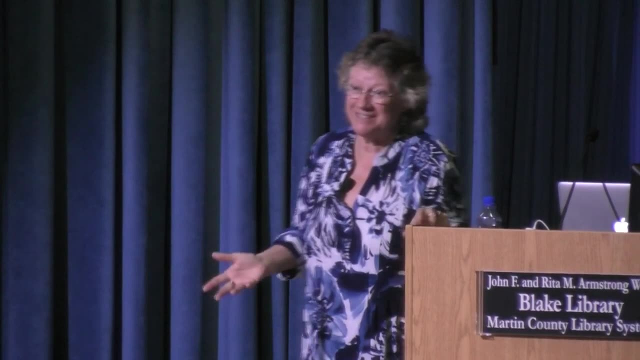 You know, I have a colleague that really said: well, you know, maybe they really did go somewhere else, right, Like that's very possible. It's just that It's a big Bahamas, So we haven't seen any photographs that would tell us that and why they wouldn't come back. 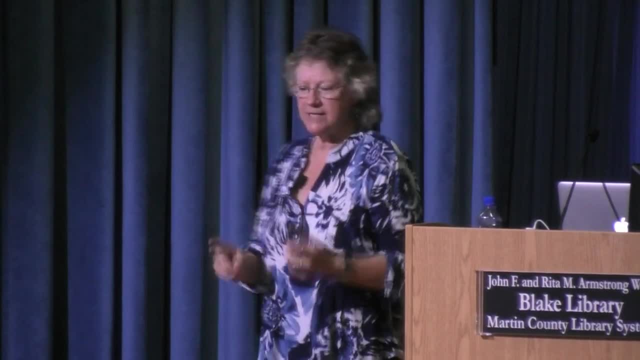 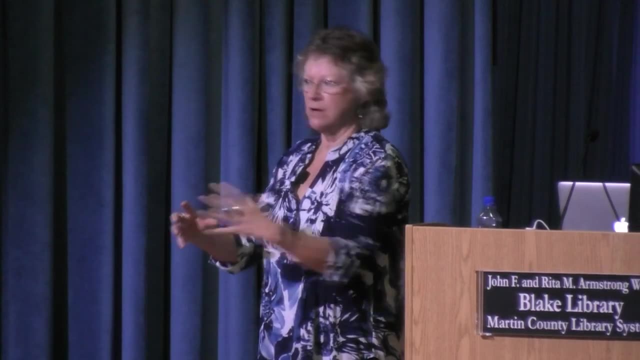 So like when we lost our spotted. what was really interesting is so we would have, like a family group was all gone, except for, like the male that was in the group, Or a juvenile group- they were close buddies. 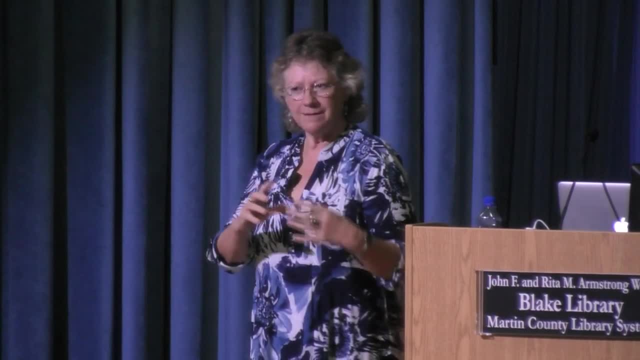 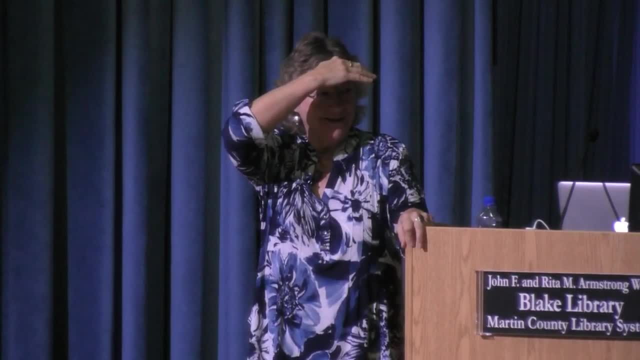 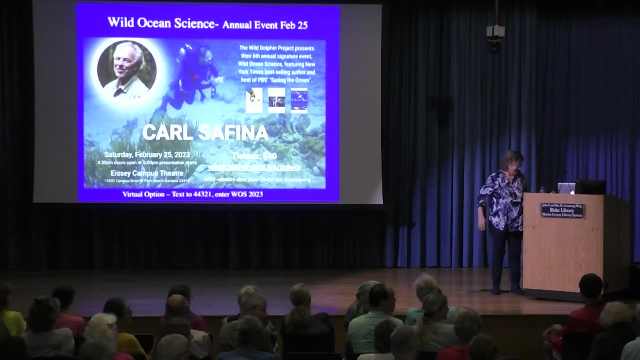 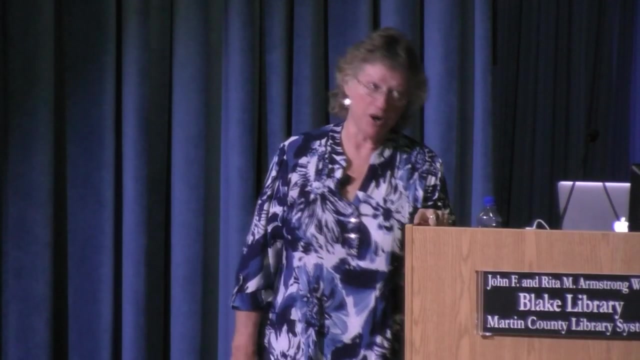 no, no question. okay, i've got more. there it is. it's a delay. i've got one more neat question from one of our online viewers: where do the group allegiances lie for the hybrid offspring that you mentioned? what a cool question. cool question, uh, yes, so hybrid offspring are are rare, so we've only seen a few. 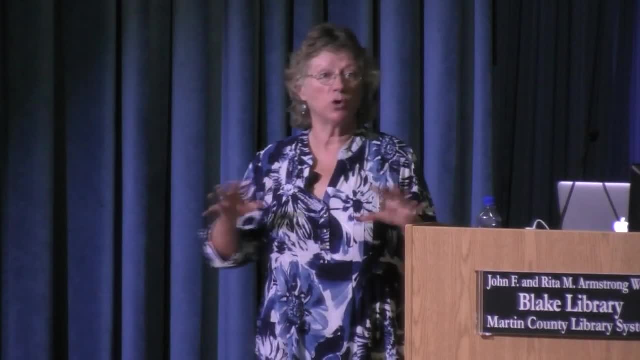 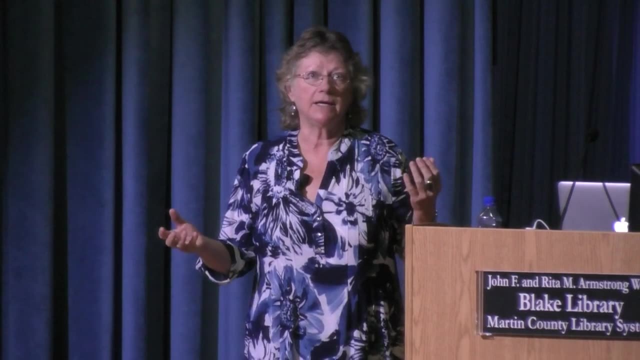 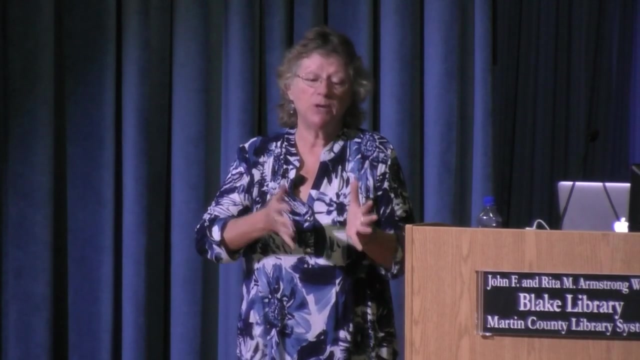 that morphologically look like hybrids, although all around the world now you can see people are finding hybrids in mixed groups, like there's always been reports, like in the eastern tropic pacific, where the tuna fleets have decimated all of the populations. tons of observations of spinner dolphins and pan-tropical spotted dolphins. showing strange shape. colored dolphins- right, so we know they hybridize. but remember if you hybridize to keep that genetic formula you have to mate with another hybrid, right? so a lot of species hybridize. So if you have a spotted bottlenose mix, say, that animal grows up, mates with a bottlenose. 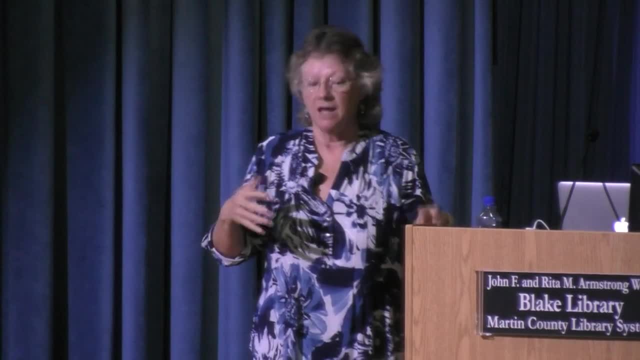 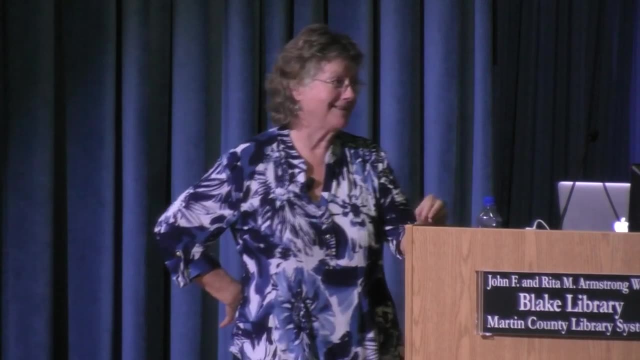 so then now all of a sudden it's less of a hybrid right. Where do the allegiances go? I don't know. that's a good question. I would hope with mom, but you know I'm seeing some hands go up in the audience. 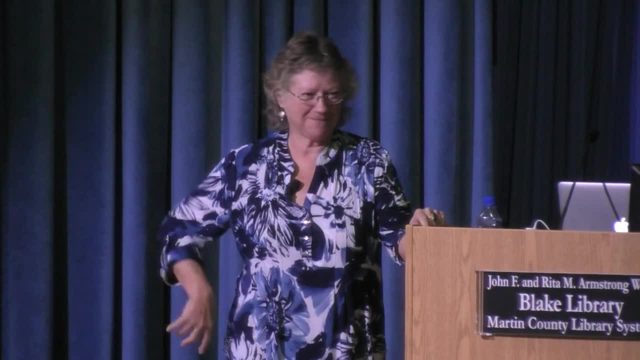 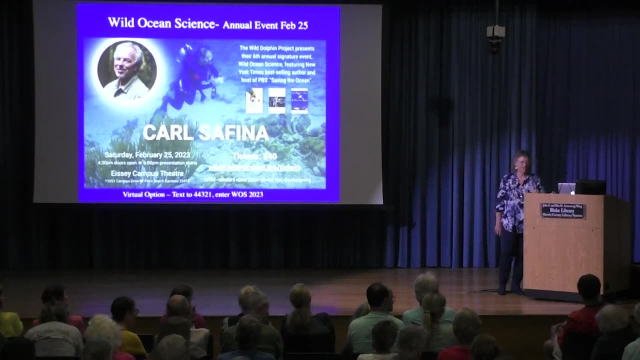 We do have enough time for maybe two or three more questions here. at the Blake I got another one: Does the temperature make a difference in whether they have males or females? Would you mind repeating that for this, Temperature have a difference whether they have male or female offspring? 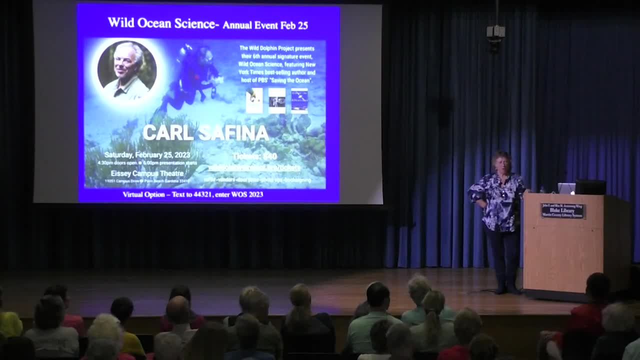 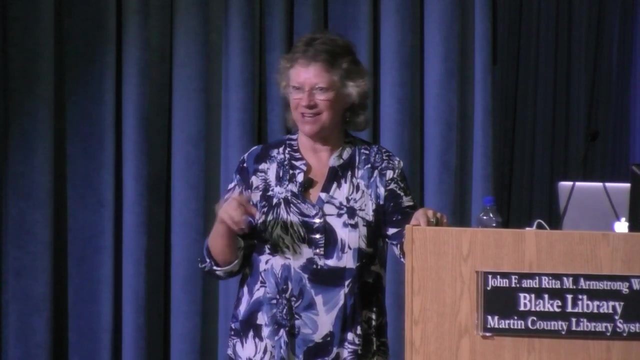 Right, Well, I don't know about in the wild. I'm trying to think if it's been studied in captivity. Yeah, I don't know. Good question, There's a research project for some young person, If your parents let you study that. So you're saying that hybrids are actually viable? Yes, they are. There was a- Oh, sorry. so hybrids are sexually viable? yes, Bottlenose dolphins have hybridized with 13 other species in captivity. OK, One good example was: Hawaii. there was a bottlenose dolphin- hope I get this right- that hybridized with a, not a pilot whale. what was it? Pseudorca, yeah, maybe. No, it wasn't a Pseudorca right. 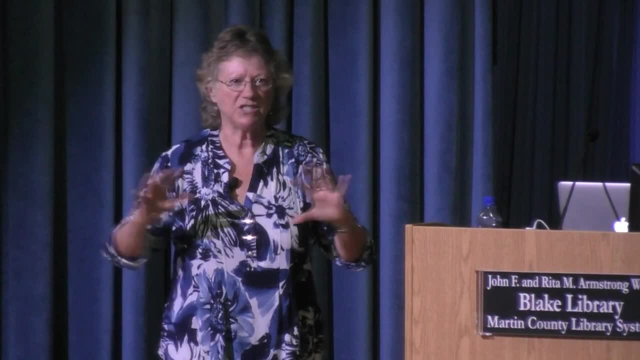 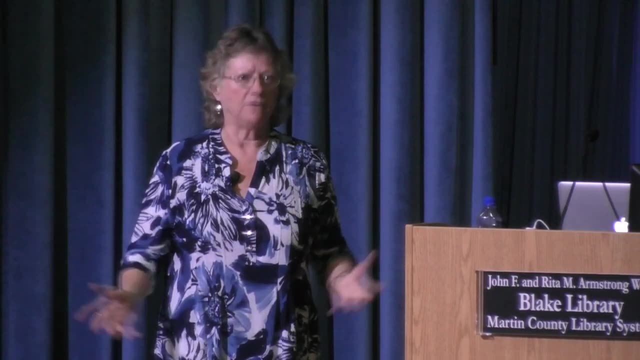 So this is like a false killer whale, it's like a kind of a pilot whale sized dolphin. Anyway, they were both in captivity. they hybridized the offspring, then grew up, mated with another dolphin. so yes, You know, they have they actually. hybridized fairly easily because they have the same amount of chromosomes and they don't seem to have some of the impediments that other species do with immune systems and things like that. But again, you know, if you want to build a hybridized community you have to have a lot of hybrid hybrids, right, That's. happened in Africa. there are a couple species of monkeys that had that happen. they lived adjacently. they hybridized enough that all of a sudden the hybrid was a community, you know, so they were on to themselves, Yeah, So, yes, they're often viable. There are blue whale and fin whale hybrids that were viable too. they found from old whaling records. so, yeah, kind of crazy. So, yeah, the question is about their immune system and does it get weaker? Listen, dolphins get all the diseases we do, You know. they get cancers, they get bacterial. 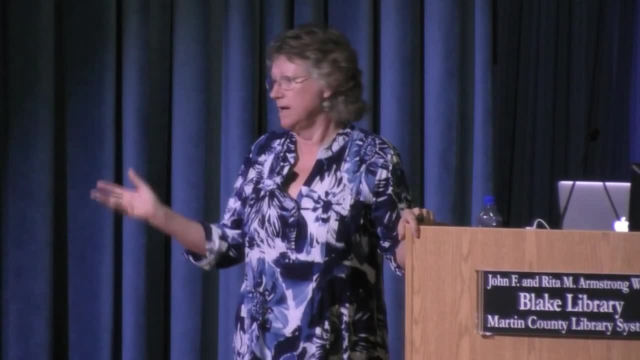 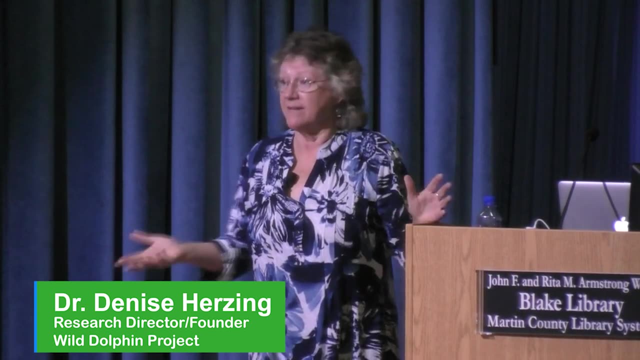 infections, they get viral infections, they get fungus. This is, excuse me, this is not unusual. you know, in the wild It's just what they do. You know, wild populations have to have a certain amount of immunity, but there's horrible viruses that can go around and 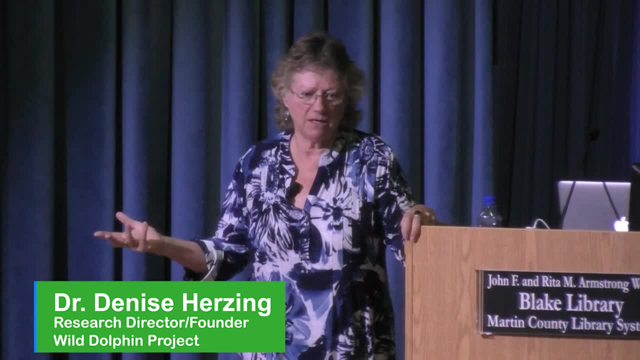 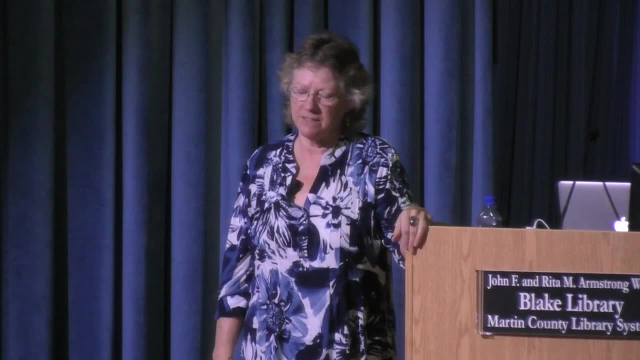 kill. you know, communities like Morbilla virus is one we've had here, lobel mycosis in the intercoastal. it's like white poopy thing that we see in a lot of the dolphins. So, yeah, I mean it's nature, right? Yeah, all right guys. unfortunately, 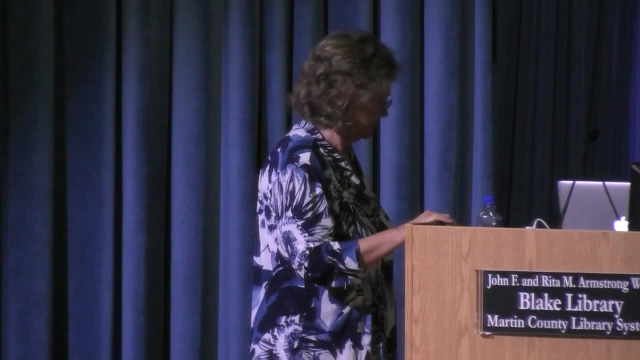 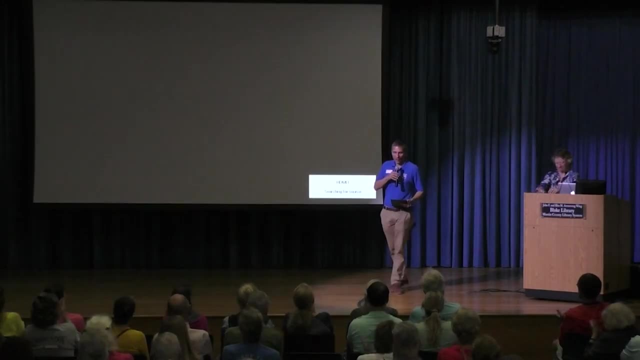 that's it for time. If I could have, you guys give Dr Herzing one more big round of applause as a thank you. I would imagine that if you have more questions for her, we do have to get out of the library here in a couple minutes, but if you want it I bet you should be happy to chat, for at least. 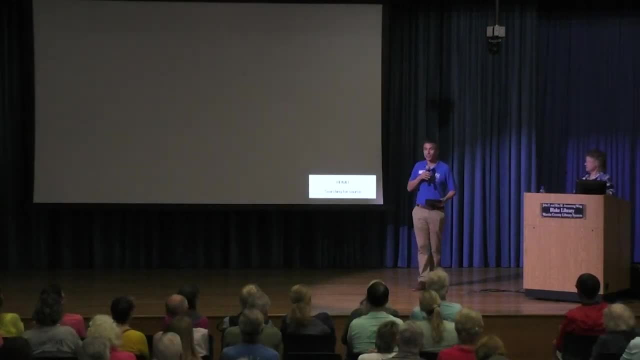 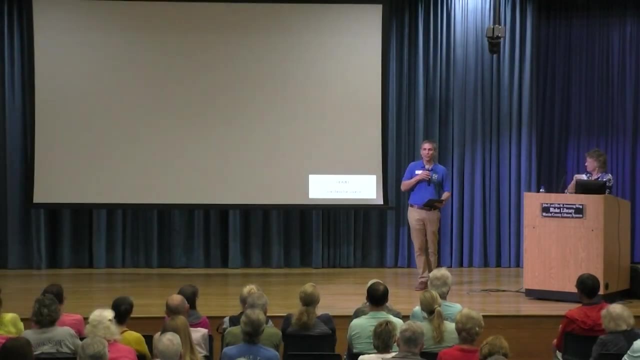 a couple minutes. She has a little bit of a drive to get home. I do want to get serious for just a second right now. Believe it or not, we had about 130 people here with us live at the Blake. We had another 200, just under 200- watching on Zoom, And I know some of you, I know some of you did. 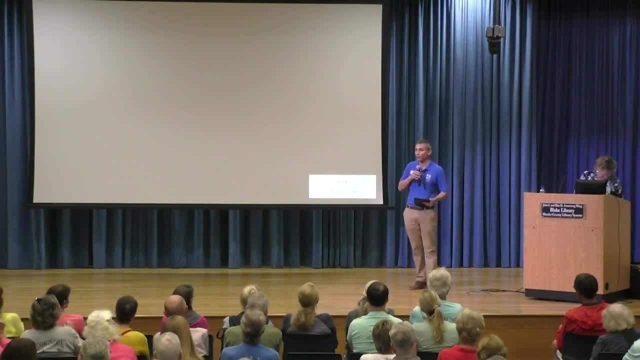 did not make it to the lecture that I gave two weeks ago about Florida's water quality issues, And I want to urge all of you, if you haven't seen it already, to go watch that recording on our website, And here's why It's very relevant right now. When I gave